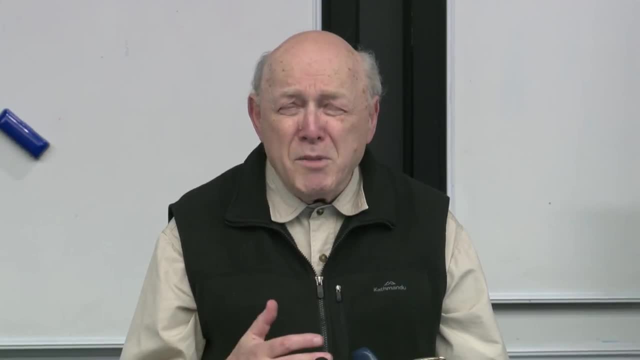 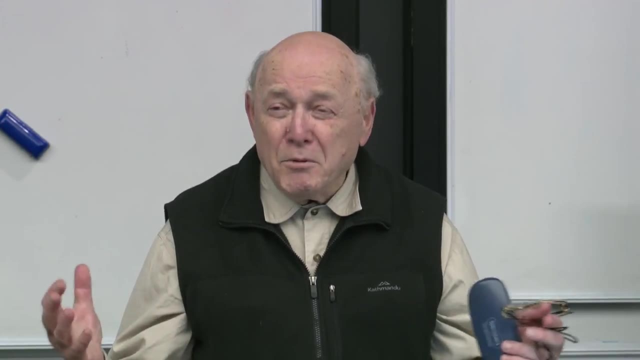 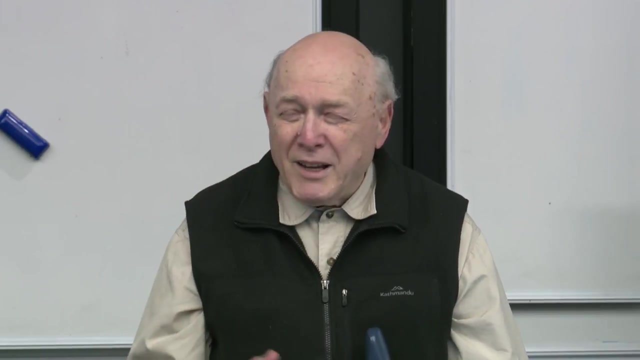 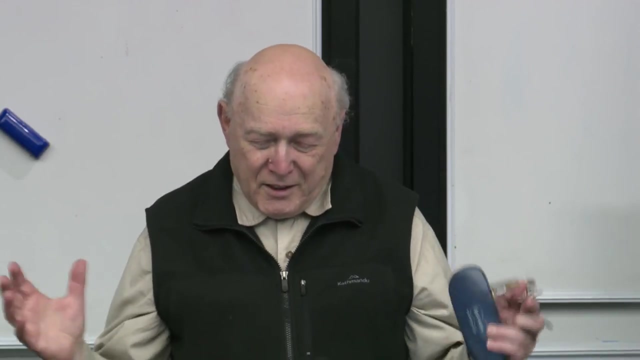 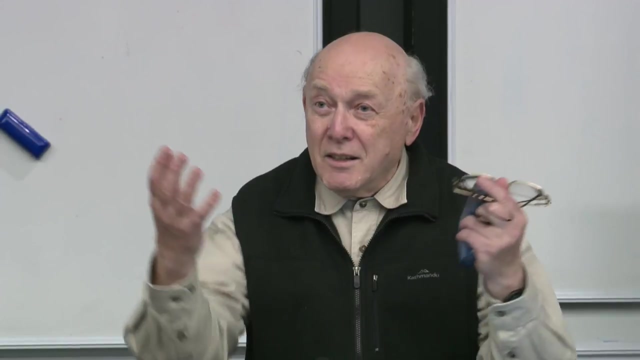 You can understand that robots should somehow mimic people, and vision is our main means to get information about the world: 80% by some evaluations, and about 50% of our brain is involved in vision And this fast and efficient perception of real world three-dimensional environment, by simply acquiring and processing a sequence of optical images, nothing else. it is a magic ability of our brain. 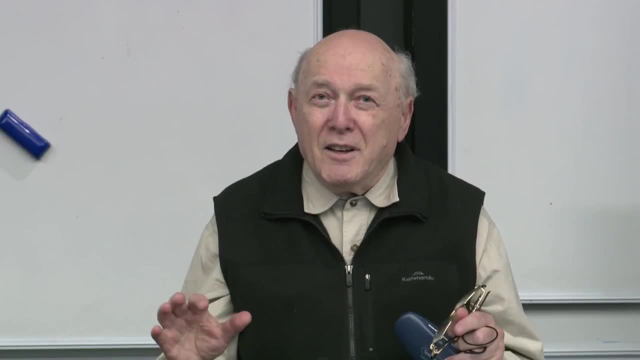 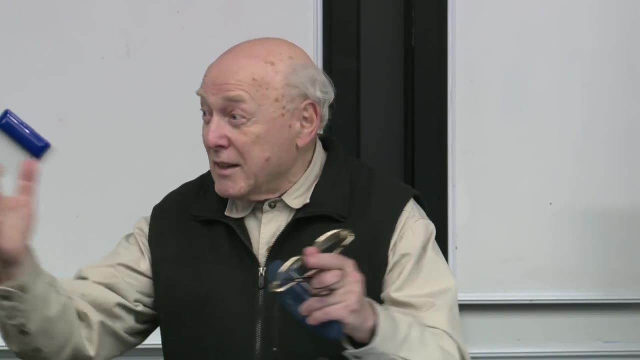 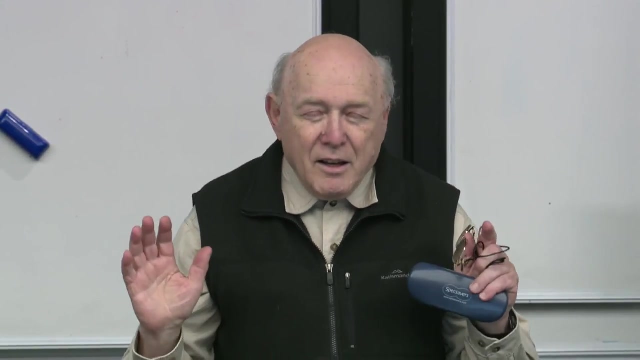 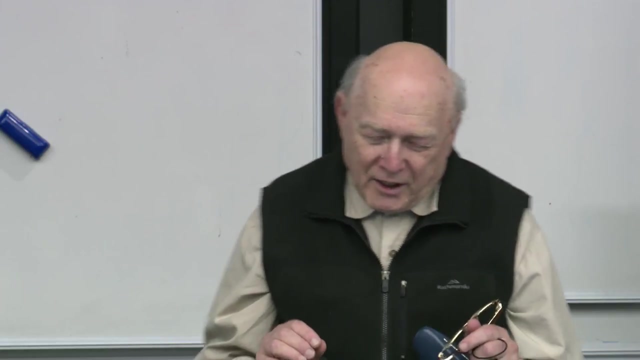 Actually, every of you have magic in your life and you are using it without understanding that it is a magic that we can see And understand and recognize everything around us. Okay, before we enter to this intricate and very interesting area, I want to recognize our sponsors. 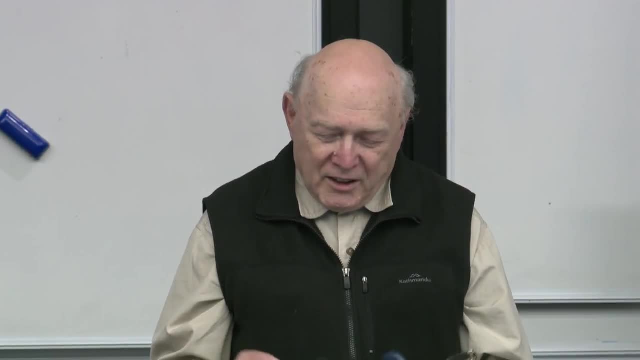 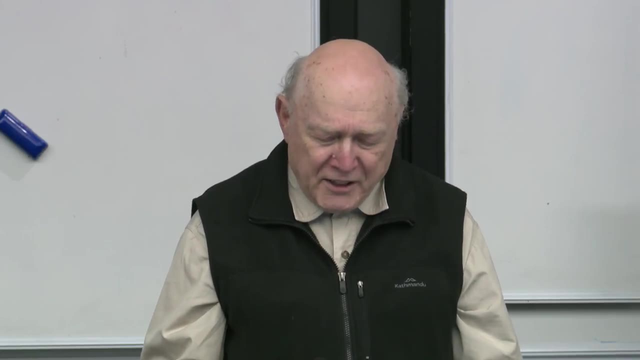 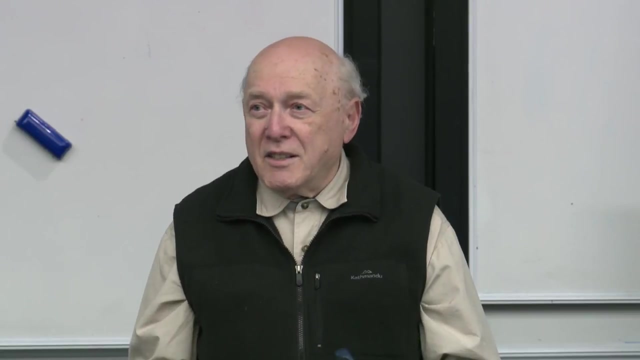 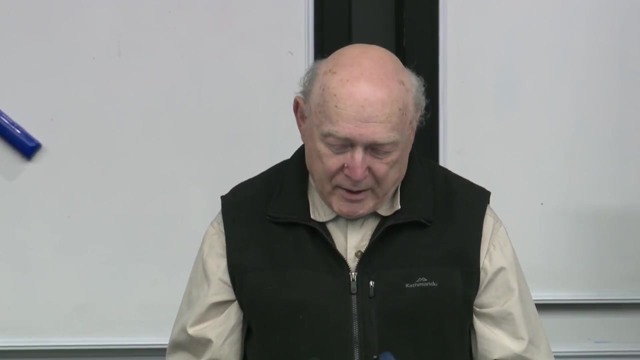 IT professionals and the Auckland ICT Graduate School. Thanks them very much for organizing, to taking part in the organization of this cycle of lectures And, of course, I want to recognize Peter Gibbons family. Always they are here for all our lectures every year on this series. 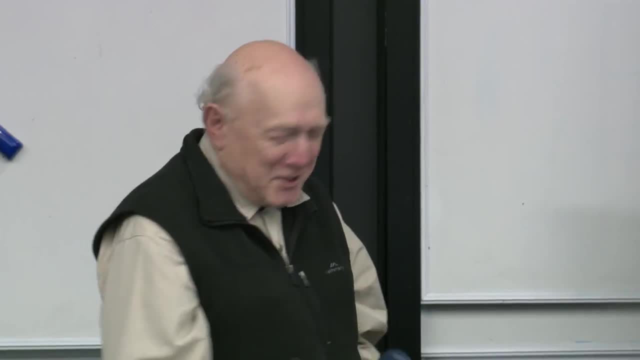 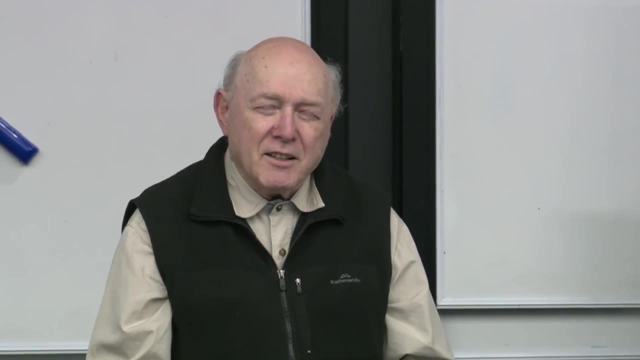 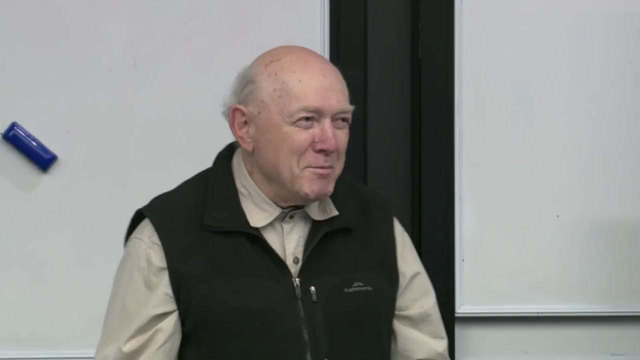 Our today's presenter, Associate Professor Patrice Delmas. I had the privilege to work with him many years. came to our department from France in 2001.. Because of his French origin, be very careful with questions. He has very good character and can explode without. 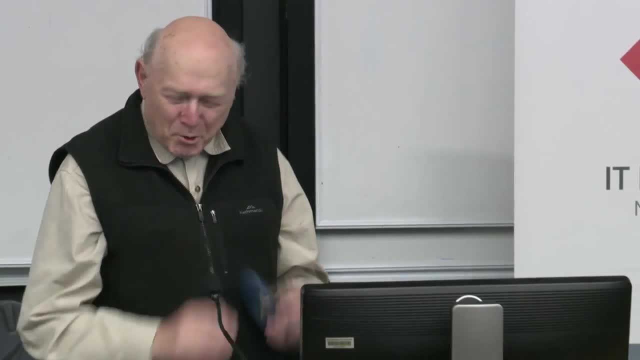 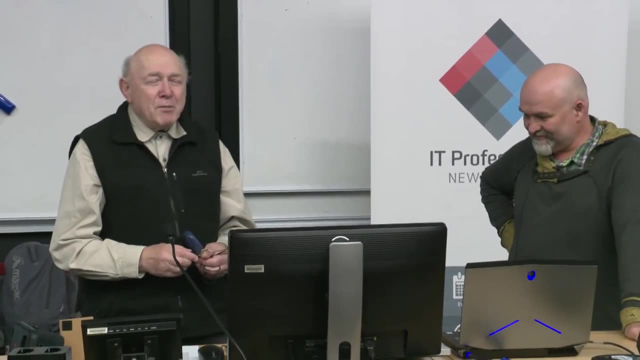 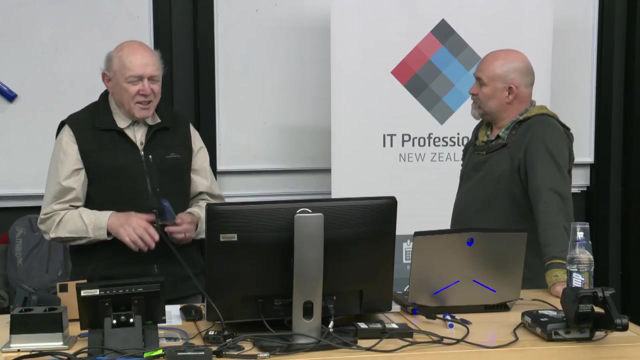 even notice. So questions should be very polite. Okay, it's just like pulling his leg, sorry. So Patrice has about two decades of experience in computer vision. It wasn't theoretical and applied. His main interests cover computer vision, computer science, computer science. 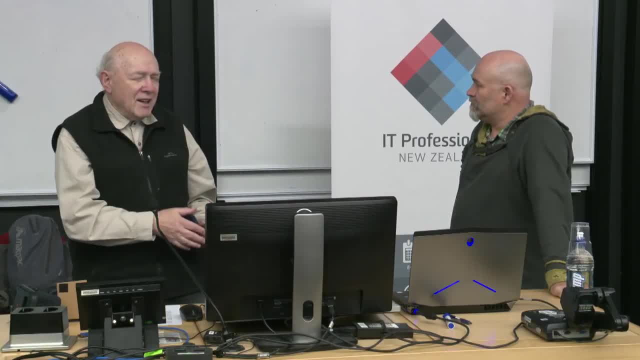 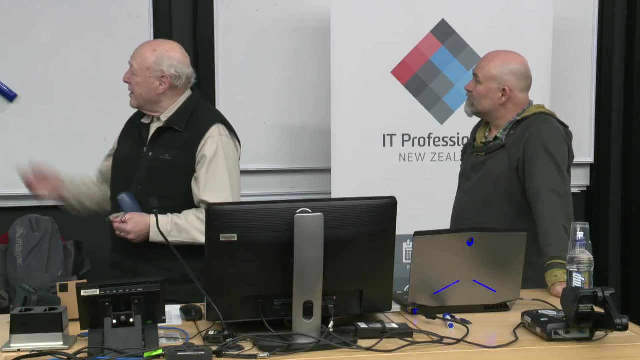 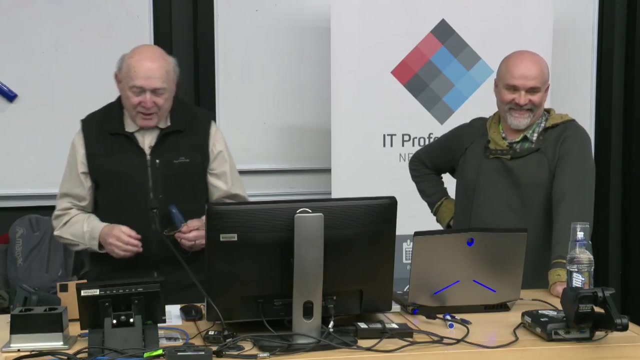 a broad area of 3D face modeling acquisition recognition. You can see these lips and deformable boundaries which try to get these lips. It is Patrice's work when he was young. Also, he is interested in computational three-dimensional vision. In short, he is interested in the. 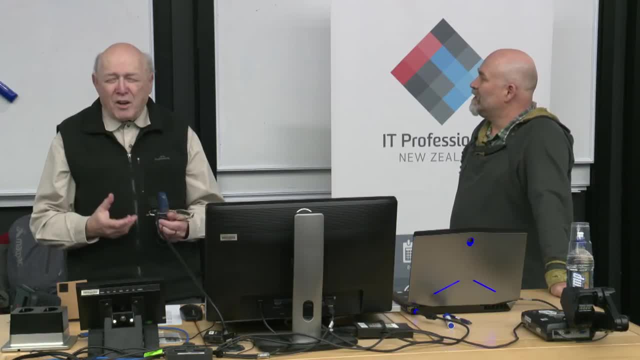 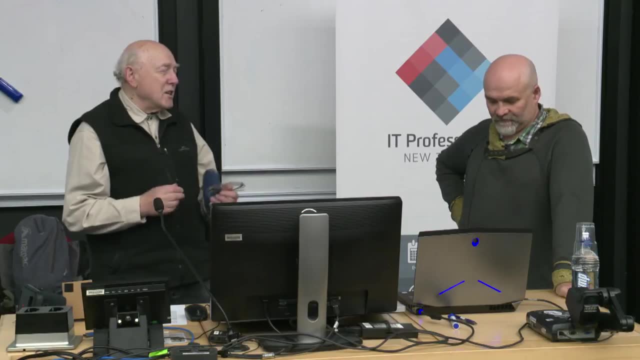 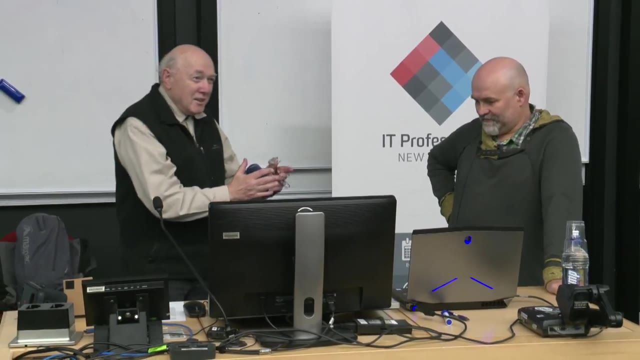 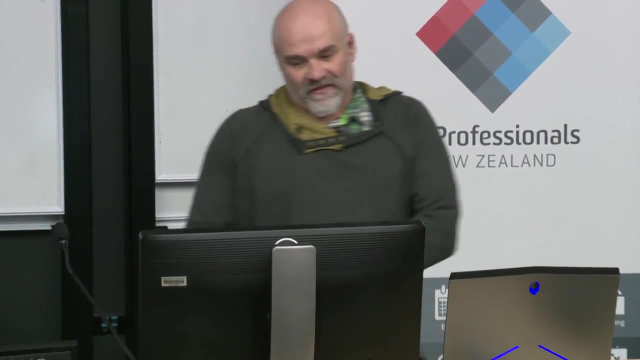 world of 3D vision, in particular in stereo vision, which mimics our vision by two eyes, And image processing application to soil science and medical imaging. Now let Patrice explain us some things that I don't believe by myself, Right? So if you have difficult questions, in the end he's the real expert. I'm just 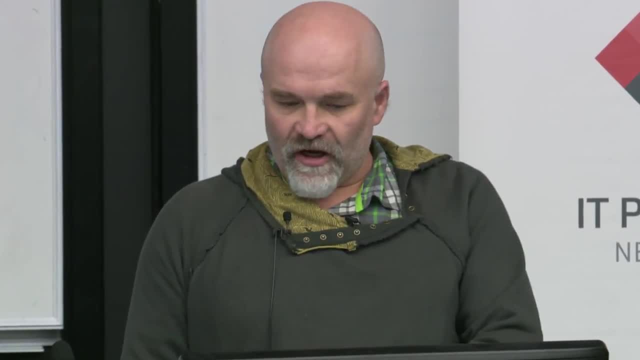 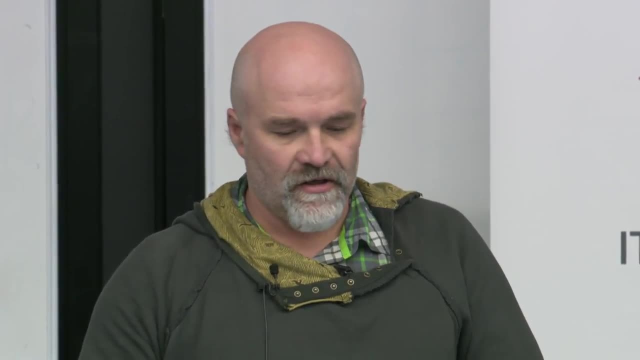 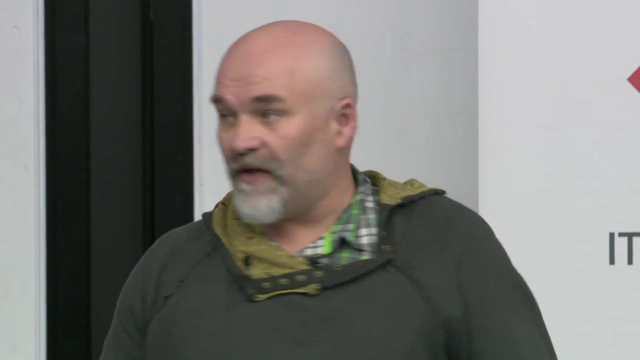 here because Thanks a lot. So I tend to make a lot of jokes while I give lectures. Usually it's to try not to fall asleep while I talk, So don't really notice. It's just for myself. The typical one I make when I go overseas is to put a cow there because 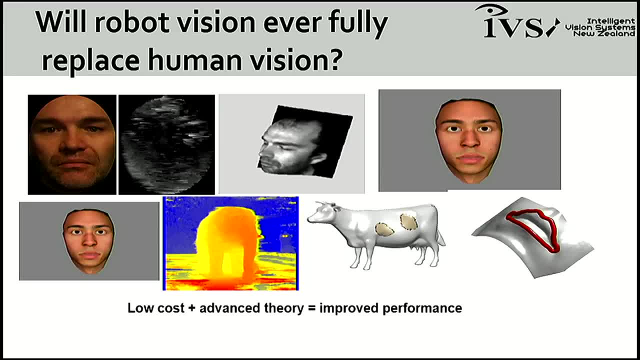 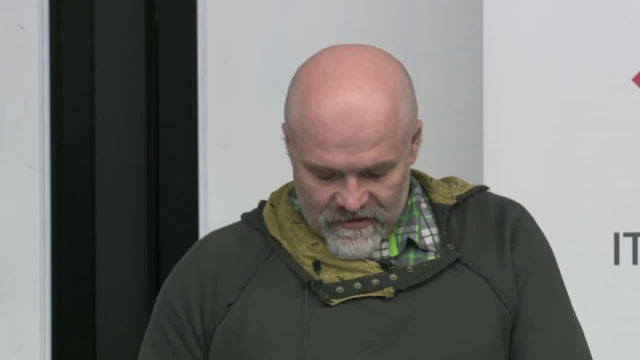 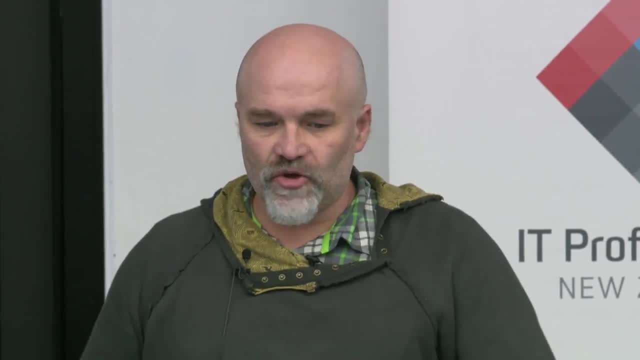 New Zealand is dairy farming famous, well famous. So we don't do anything about the patches of that cow, It's just for show in our dairy farming industry. All right, Let's move on. All right, So I have to go to this one, All right, So fairly short, So yeah. 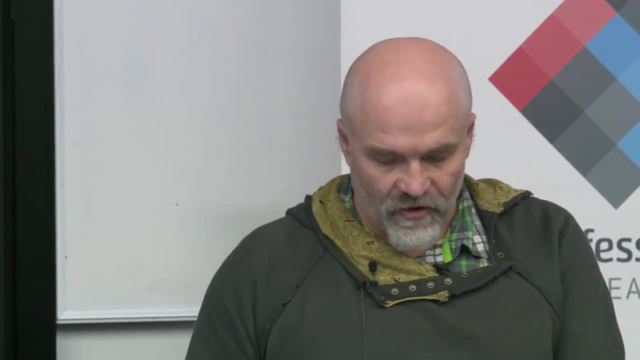 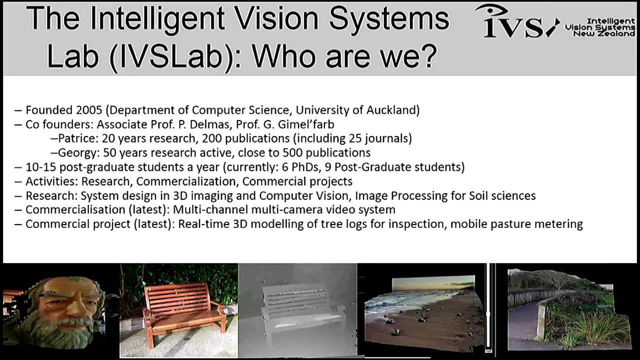 about the title. I think Gheorghi is right not to believe the title, And we'll see a bit more. We'll start with introducing the lab that we created together with Gheorghi. So I had the privilege to work and still work with Gheorghi. We founded an intelligent vision. 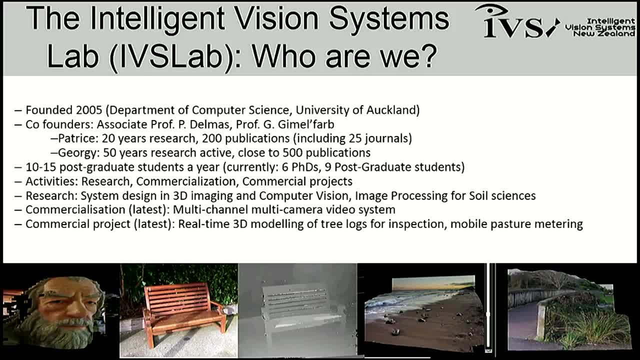 system lab, And I can tell you there's a word called intelligent in there, And do we believe we're doing anything intelligent? I don't know, But we're trying very hard, So that's important. Talk to you about our publication. We get a massive influx of students. We are 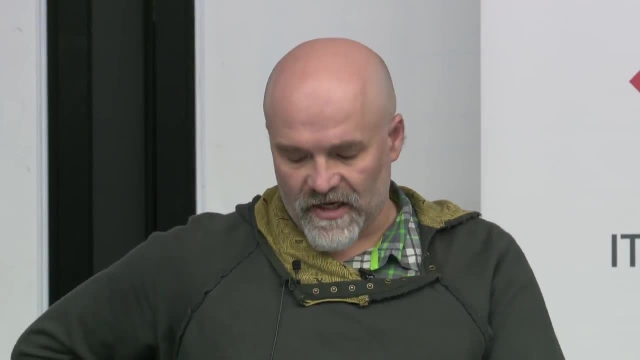 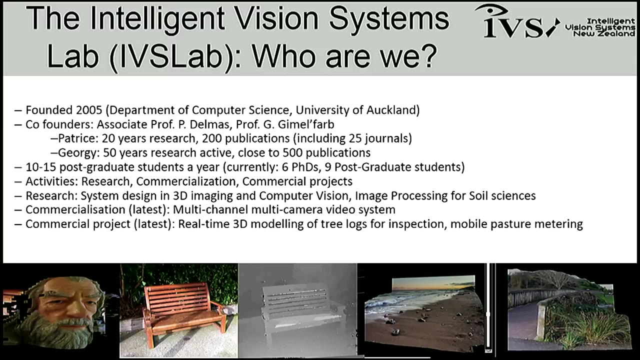 very fortunate to have a large lab and very well resourced thanks to the University of Auckland. Overseas visitors are always jealous of the amount of computers we have and different systems, Because computer vision doesn't have a lot of people working in New Zealand. it's. 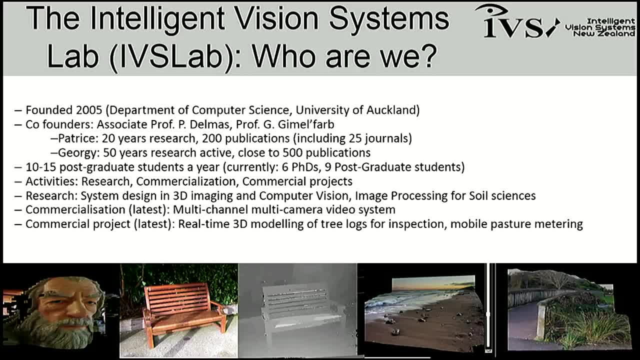 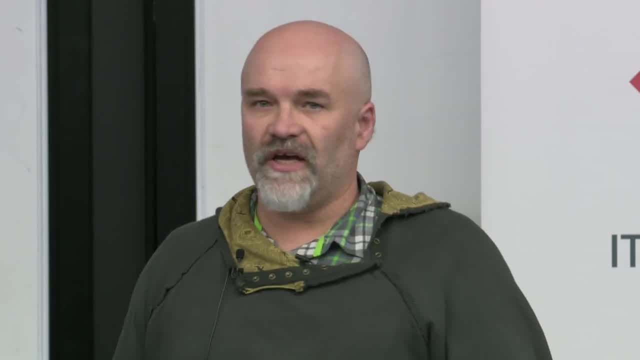 very rare in New Zealand We do manage to get some commercial projects. Our activity is really system design, which is we take the theory that we invent and there's tons of algorithms Gheorghi has created and some we created together, And my goal is always. 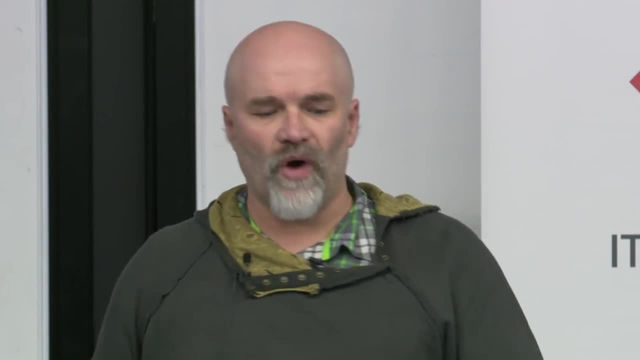 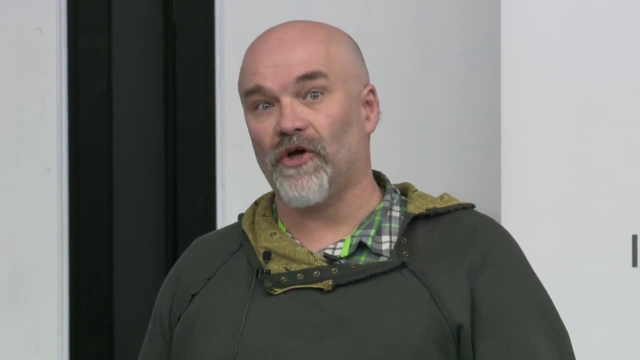 to say: how can I use that for something useful for someone? or to have some fun, which is, take some equipment, put some algorithms and see what happens in the real world, which usually means it's not going to work. That's what happens when you leave your lab: Nothing works. And today I hope to show you. 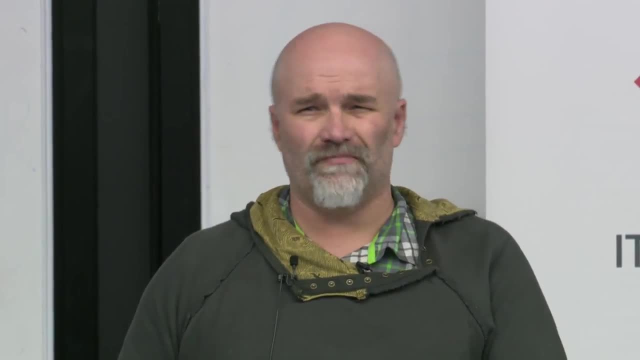 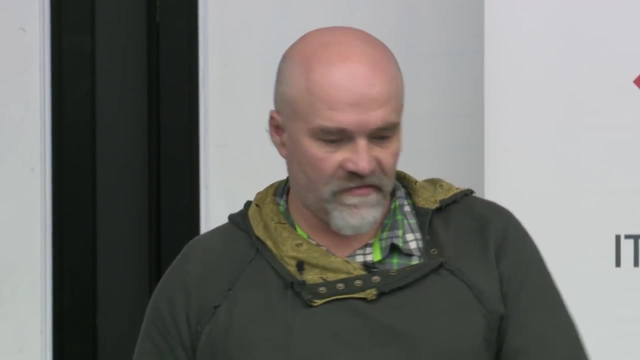 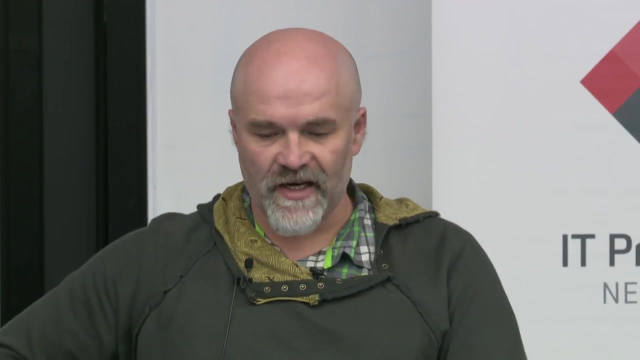 that it's cool, it's fun, but often it's quite painful as well. As a philosopher said, no pain, no gain. So I think we're there, All right. So we have also the famous Gandalf Academics from Wellington University. I think It's maybe a movie, I don't know. All right. 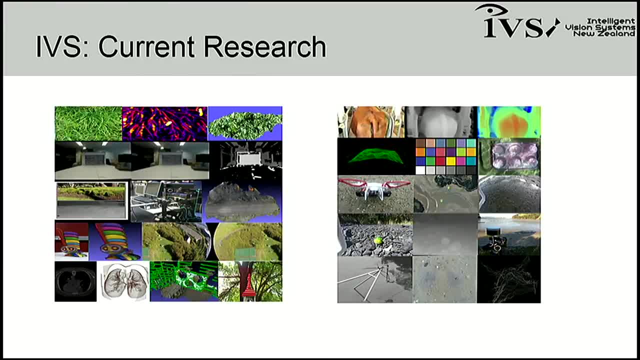 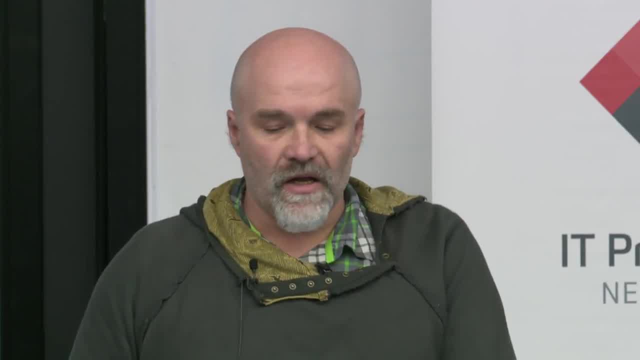 So our current research. I don't want to say too much about that, I'm going to talk about it. We tend to use a lot of different cameras, different systems for various applications in dairy farming, marine science, New Zealand, environment is what interests me a lot, And 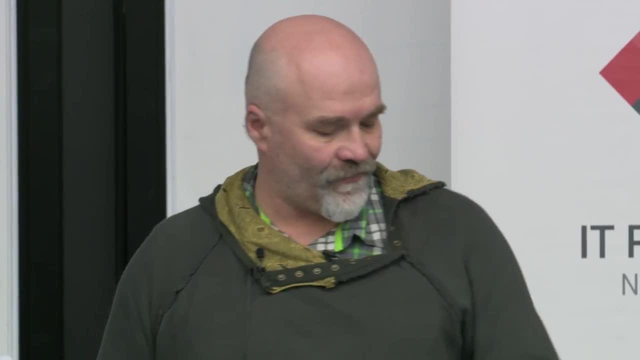 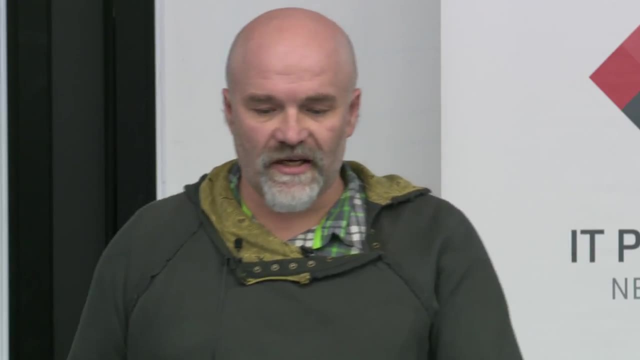 also soil science, but we won't talk too much about that today. All right, To do research, you need money, not just to pay your salary, but to basically travel, go to the fields, engage with overseas people, And you need projects for that. So I think we're there. 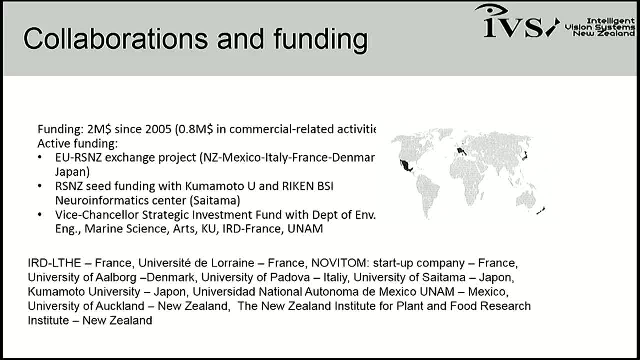 So we're fortunate to have several of these funding currently running. It allows me to travel a bit too much maybe, but to go see a nice do and work with nice projects. So mostly my engagement is in Mexico, Europe, New Zealand and Japan. All right, Now let's. 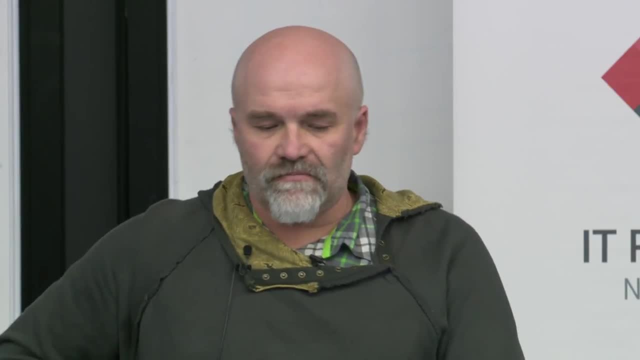 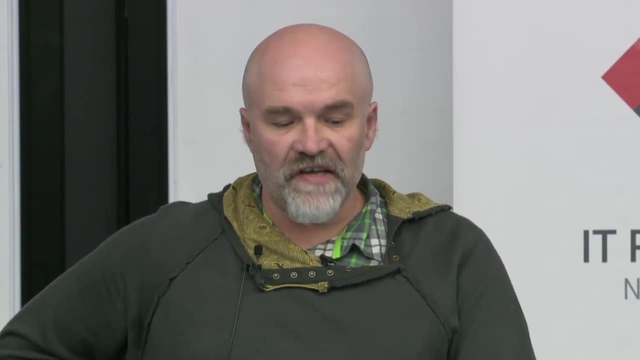 try to define exactly what we're talking about. It's always a problem. It's like philosophers discussing their own household and family. It's always a problem. It's like philosophers fighting over it. Even definitions can be tough to decide. So, basically, if you look, 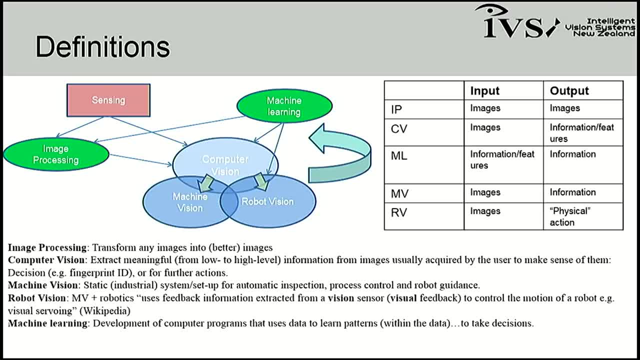 at what we teach to our undergrad, it's image processing. If you look at what we teach to our post-grad students in the area, it's computer vision. The difference is image processing. is you take any image you may find on the web. You don't really care where they come. 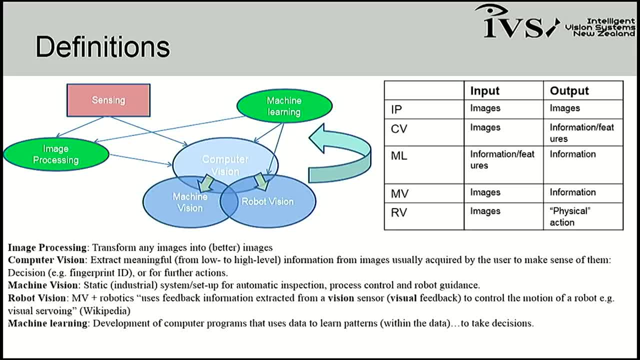 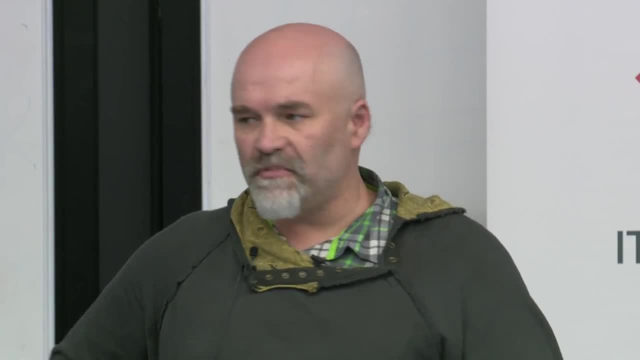 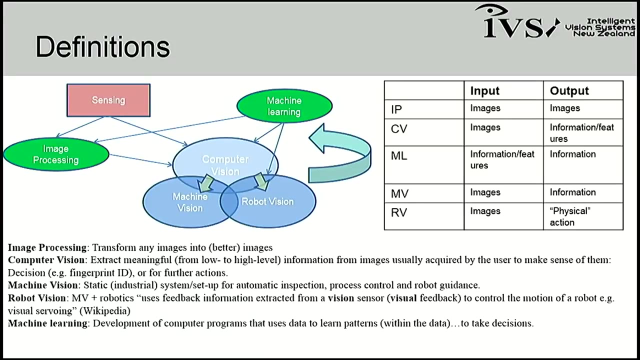 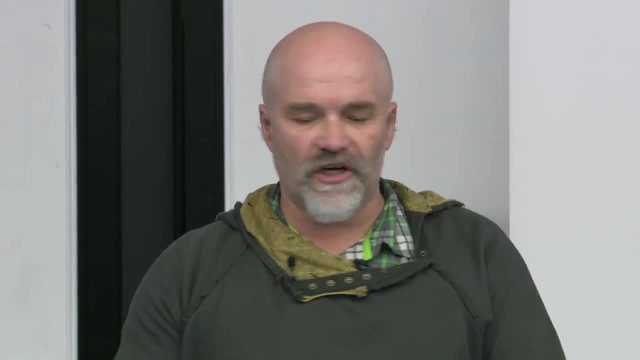 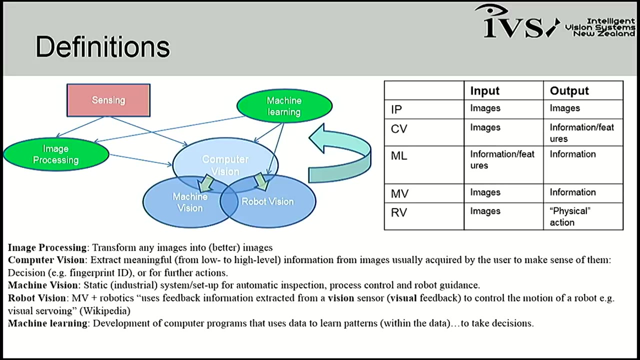 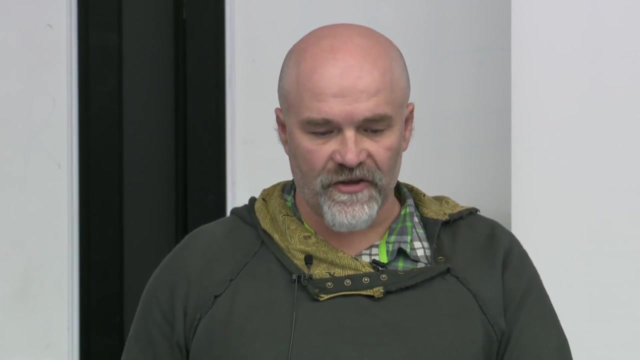 Like I said everywhere, it's just a bit fuzzy. I'm often at the intersection of machine vision, robot vision and computer vision. So today it's likely the robot talk with no robot, But we're interested in the vision, So that's okay. I'm really trying hard to. 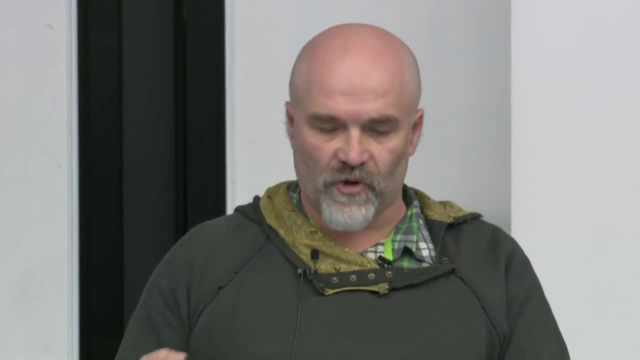 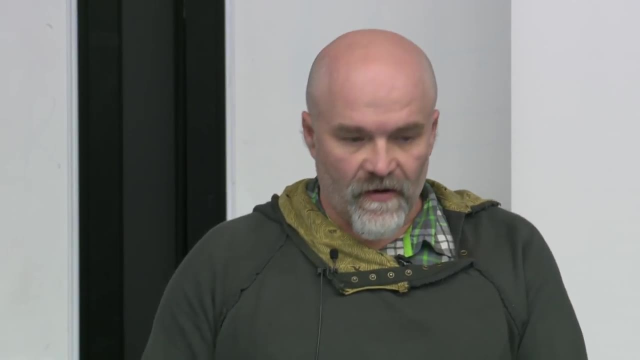 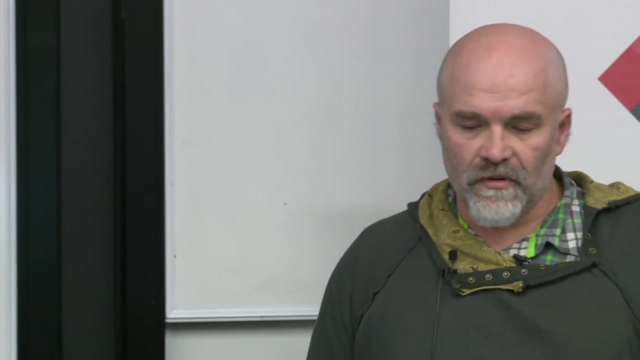 make systems that actually could be used for robots. So we have projects with Bruce where I'm actually trying to help him robots to see better, Okay. So I hope it's clear. Oh, I always get the wrong computer. Okay, did I go too far? 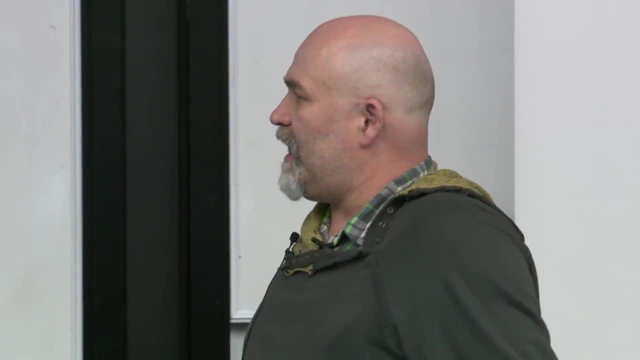 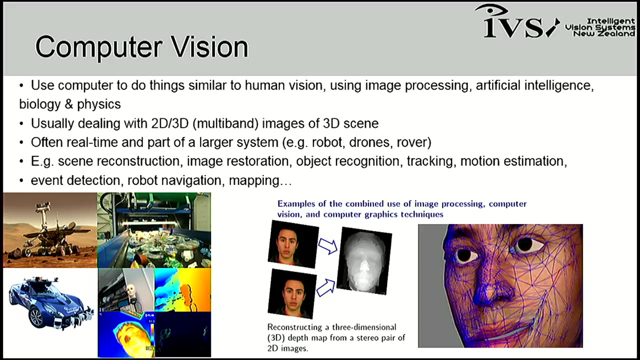 No, All right, looking at computer vision and looking at possible applications, I actually verge into so here I call that computer vision. See, I'm a bit confused because actually there's a robot there, There's the Martian robot- that could have actionable parts. 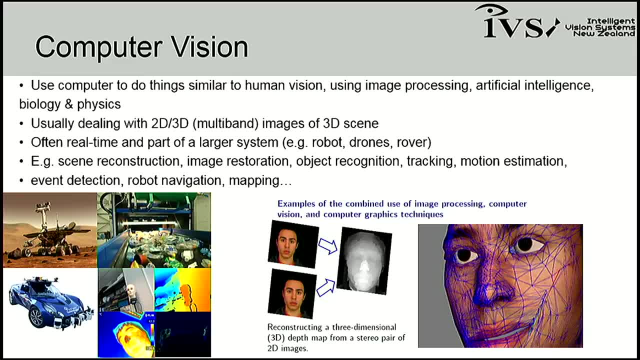 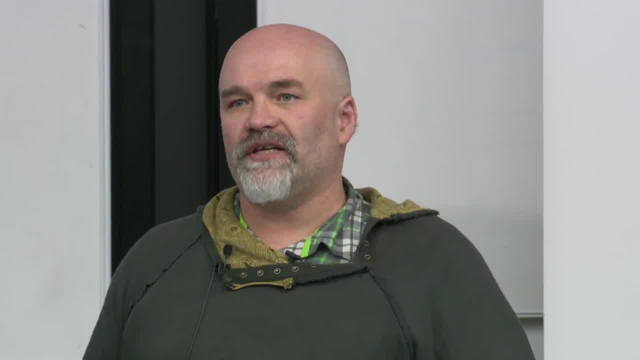 And what they would do with the NASA. they would do a small step, wait 15 minutes to receive images, decide on what they could do, send the robot, say, oh, maybe turn left. wait another 30 minutes because you send the action. 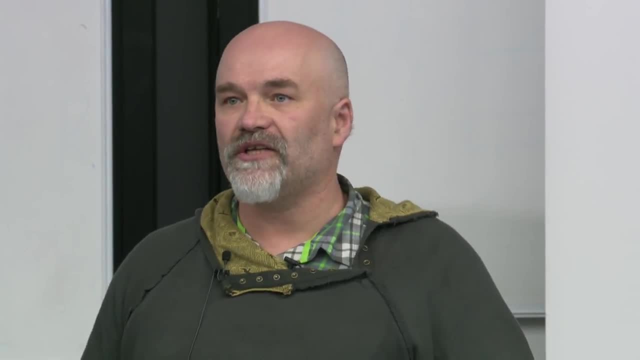 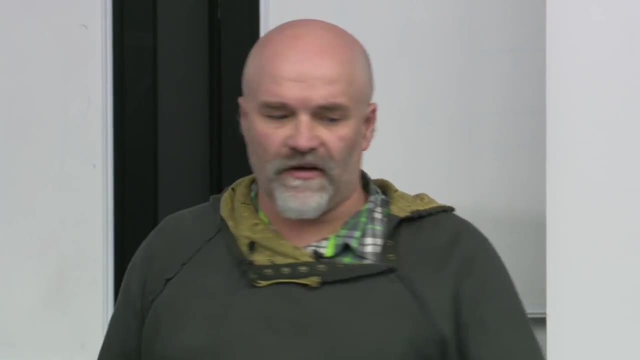 you wait for the action, you wait for the photo to come back 30 minutes later and you progress slowly and slowly And you can say, oh, I like that rock, I'll test that rock. So it's definitely robot vision. 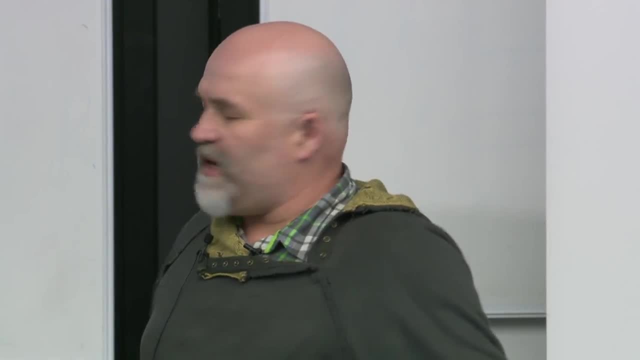 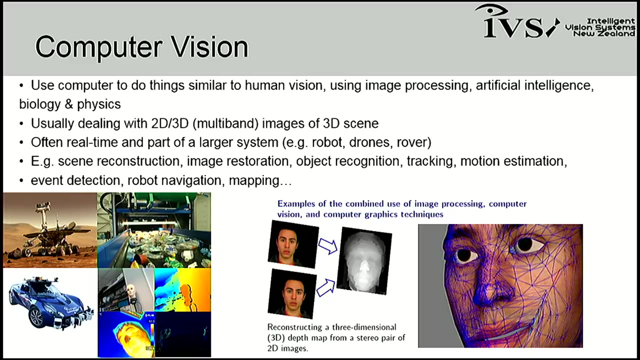 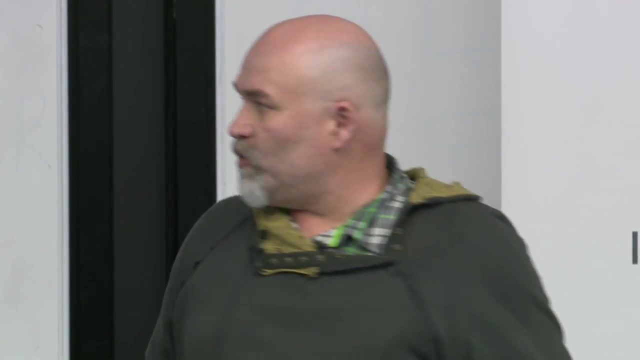 If you look at the triage of your rubbish bin, you can see that it's more machine vision. Objects are presented to a machine which is static and there's decisions on the triage. There's more of the grand challenge that blue car. 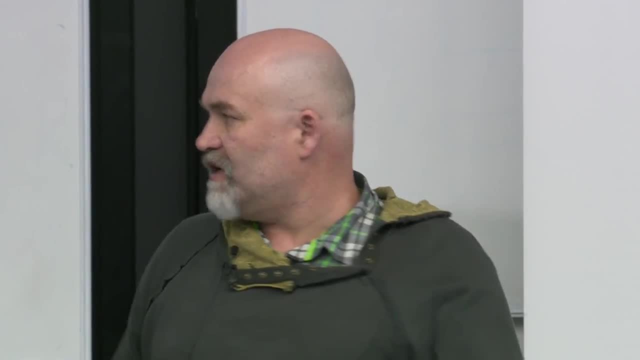 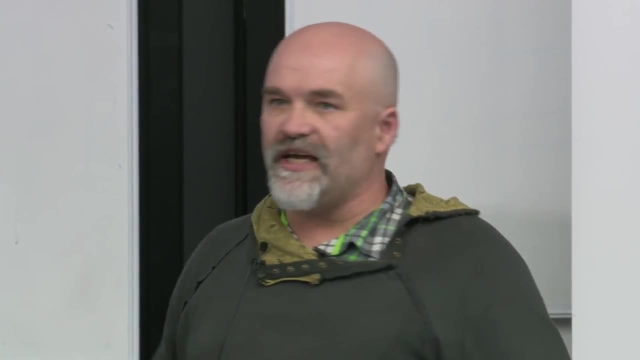 which was equipping a car with a lot of different sensors, active and passive, and trying to navigate automatically. That was the precursor of the automated navigation systems that you see now on the Tesla and other cars. If you look at the images a bit on the right, 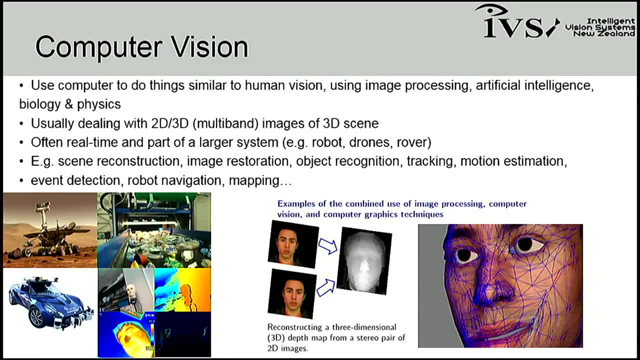 basically there's not only one modality you can have, like eyes, which is just basically optical range- We can see red, green and blue- But also thermal imaging, so the images that look very blue as actually colored thermal information. And you have also at the bottom right the LIDAR. 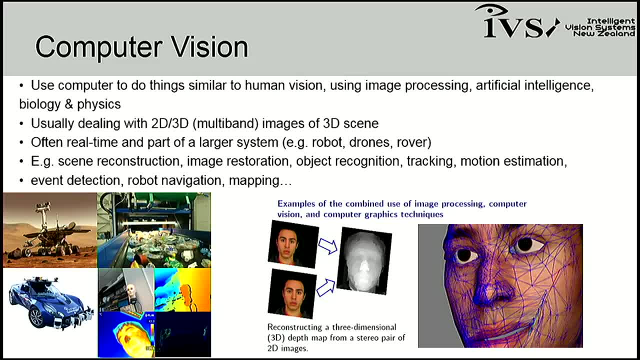 So we have several LIDARs now. It's just laser line and the beam of them that are projected towards the world, reflected and basically give you an idea of how far an object is. All these, all these cameras we have in the lab. 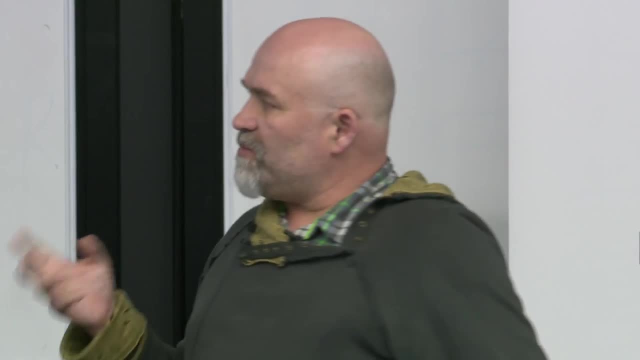 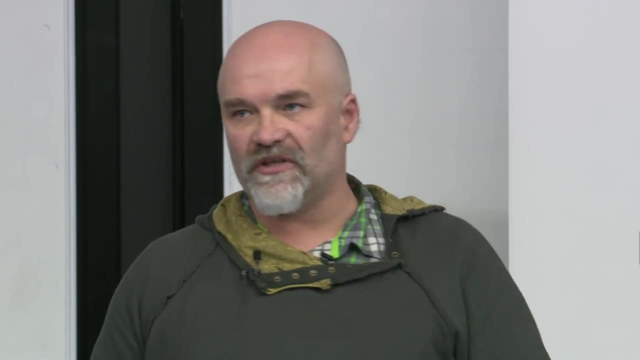 So what we are looking at is often an atypical project in computer vision. You will acquire a set of images and basically I came to New Zealand because in France at the time, the people I was working with didn't believe in 3D. 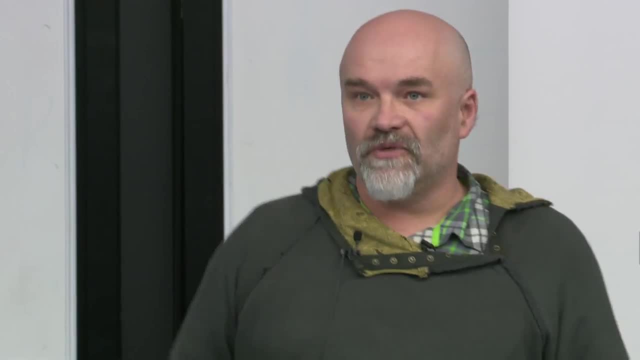 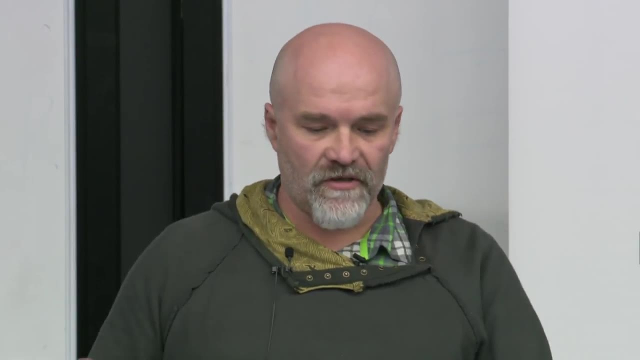 That was too early maybe, But there was a guy in New Zealand with some strange, weird shirt, Gyorgy, And I realized he was the guy I needed to work with. So that's why I came to New Zealand And basically, you need, you need, you need you know. you need. you have two eyes. It's not a mistake. Nature took half a million years to evolve humans, or more. That's a good reason for that. You need to be able to have two eyes to see in 3D. I need to be here to. 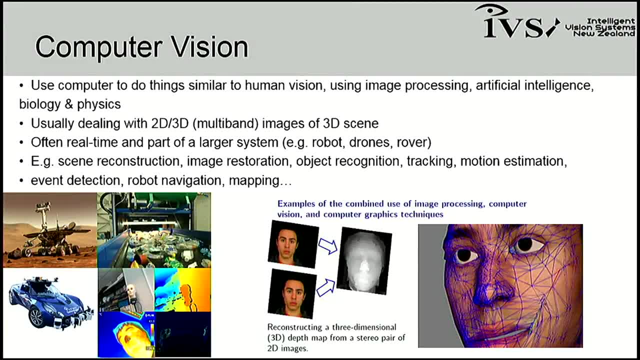 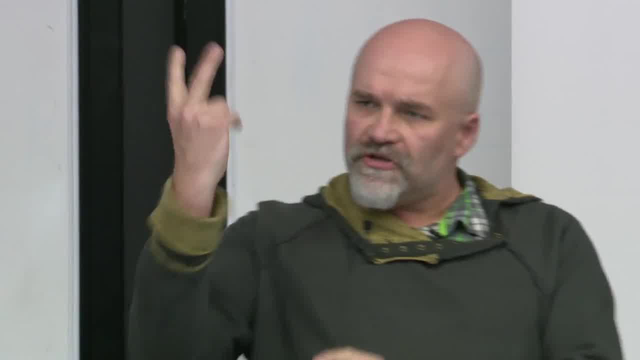 What you can do is- and that's quite an old project- is you acquire two images of someone Here it's Alex, a former graduate. You create a 3D map of his face with just two images and you use some physical models to try to animate. 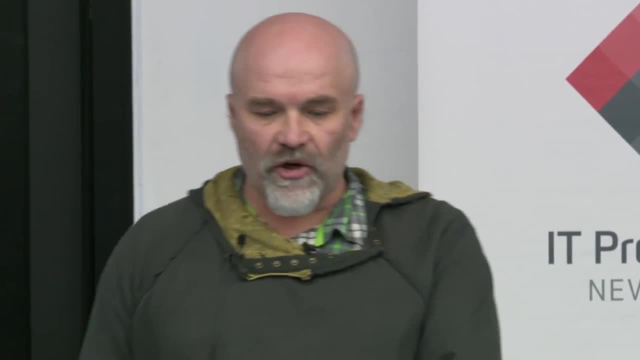 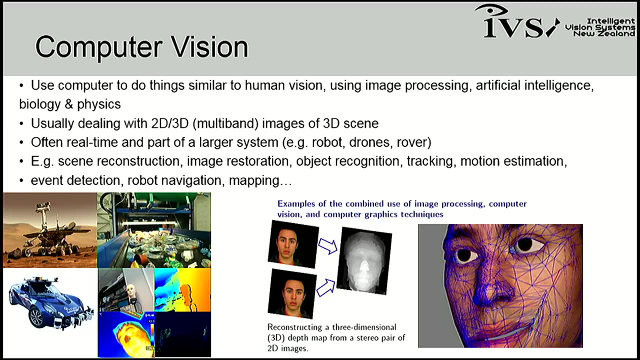 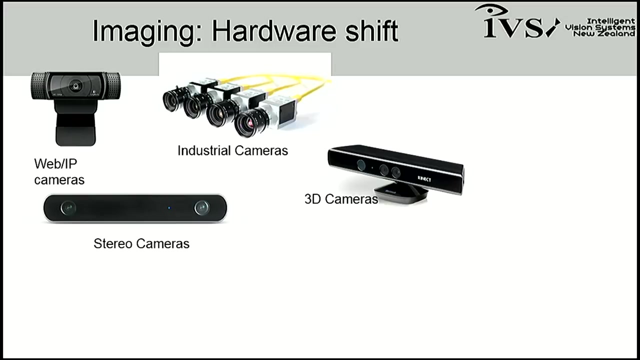 in a realistic way, something else, So typical computation problem when your goal is animation of a physical model, And we have several different problems we're working with on that. What happened recently? The world has been changing a lot for us. We are in a field where you cannot look back. 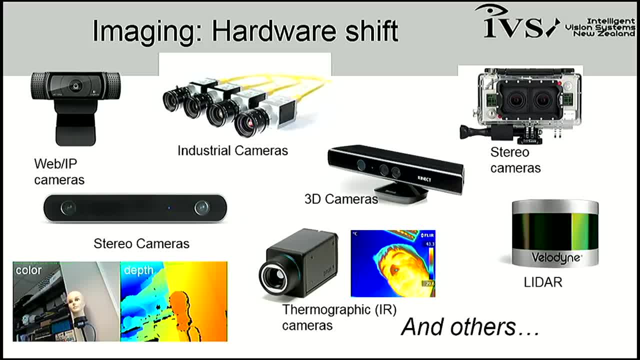 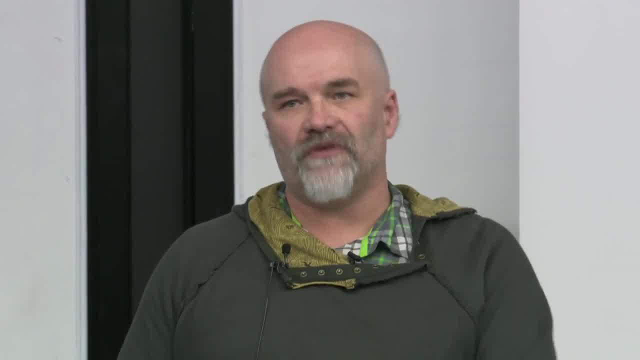 So computer science is a bit. it's a bit tough because, compared to other fields, like dinosaurs were there, They're still there, They'll be there in 10 years, in 20 years, Technology might change, but you can relax. 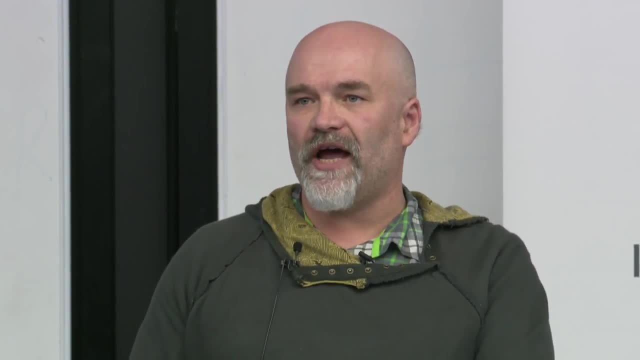 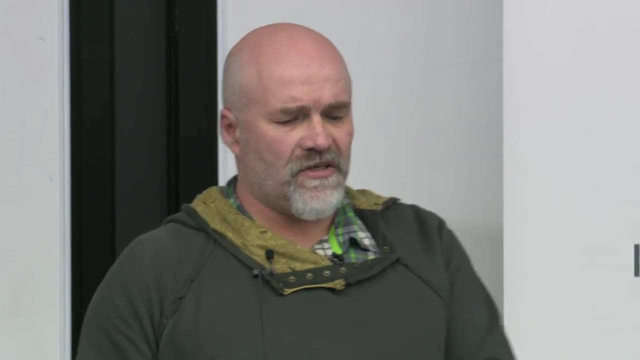 What I was doing for my PhD on the strongest computer can be done now in the medium range mobile phone. There's nothing new anymore and it's only not 20 years, less than that. So it's quite challenging and the equipments change a lot. 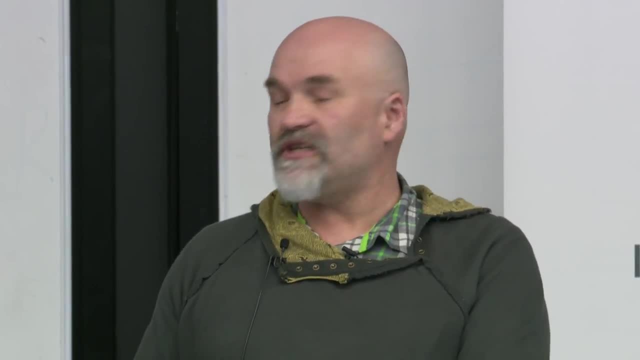 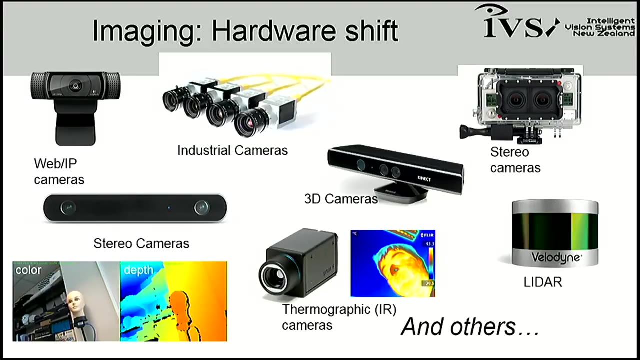 Even some of the equipments I'm showing you now are almost discontinued. The Kinect has been discontinued. The GoPros in top right: We got the last one refurbished from America. We got the last ones available in New Zealand And we're still trying to source them. 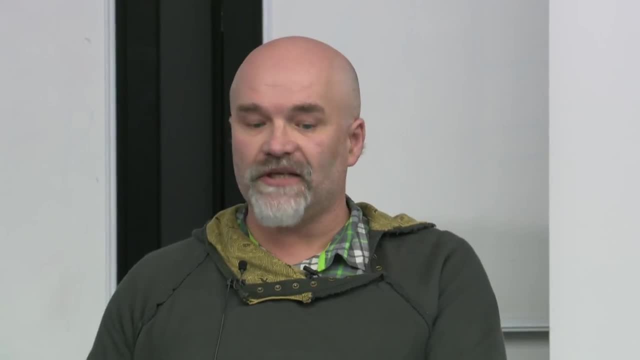 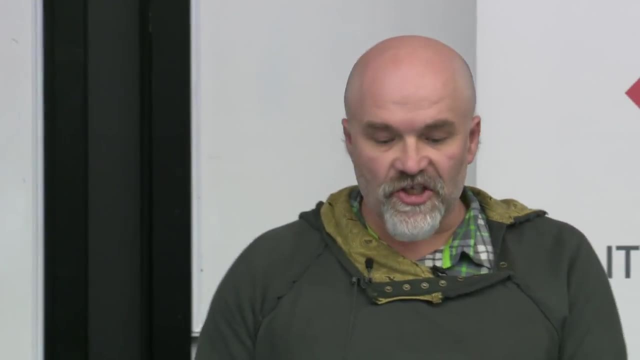 because they're the best possible cameras for our purpose. but they're not being built anymore, So that can be quite tough. evolve quickly and not necessarily for the best. But what's great, it's getting cheaper, So it's getting easier to actually buy more. 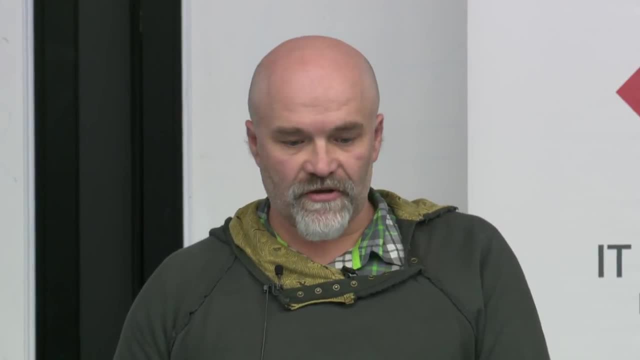 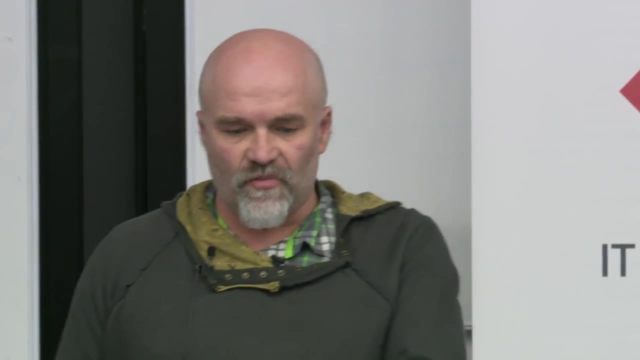 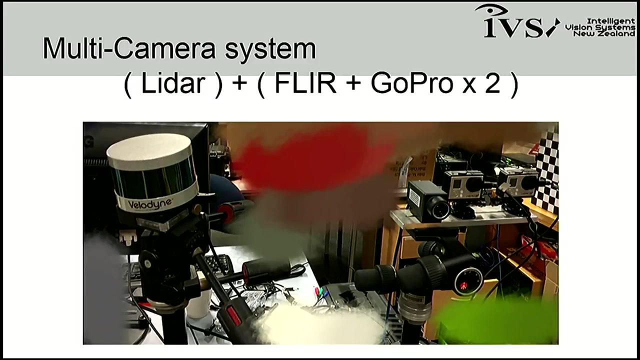 destroy them, try again, destroy them, try again until it works or not. So that can be right. So one of the system we currently play with as a mix of different sensing- and that's why I show that as a mix of different sensing modalities- we have a lidar on the left. 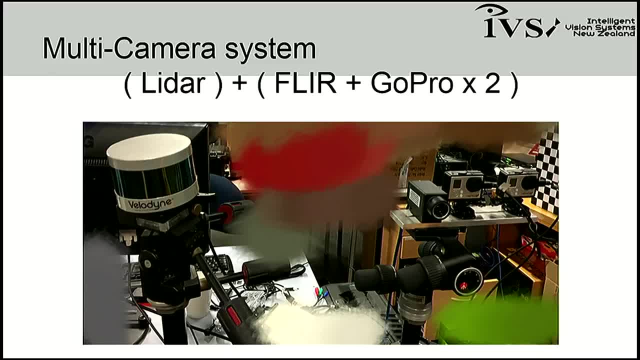 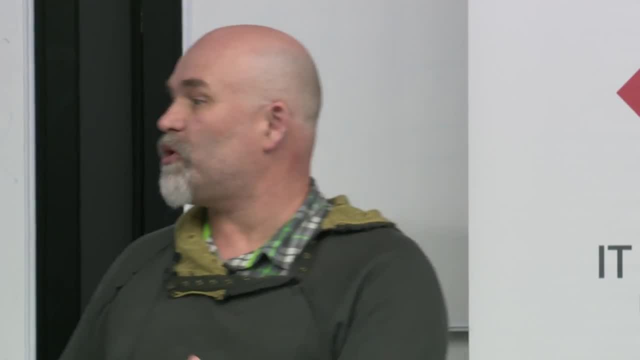 side. we have a formal cameras and two GoPro cameras. so basically we are. it's almost like an augmented human. there was like a human that could have thermal imaging and like laser lines. it's almost like a Marvel Comics superhero. so that's what we're doing in the lab. actually, we're creating super humans and 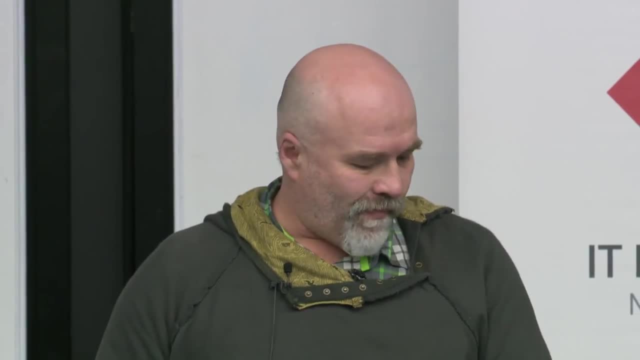 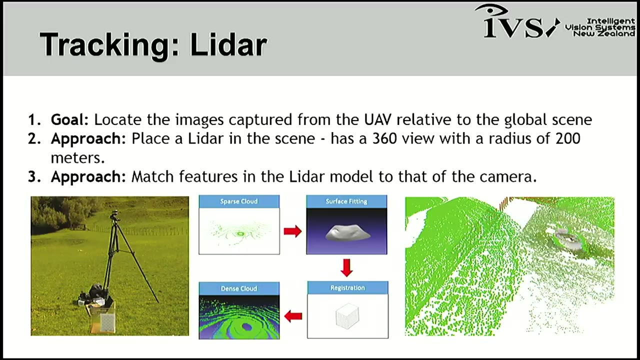 superheroes, right? yeah, well, we do with that. well, it's a good excuse to go in the field and see what we can do with that, because that's more challenging. we try to combine different type of modalities in sensing and that can be challenging because all these equipments must be calibrated. calibration process: 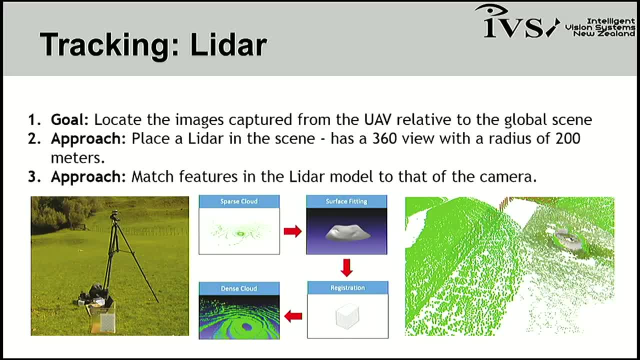 is to relate the world to the image you receive. and you have to say, well, in optical systems, okay, we know how to do that. how do we do that with lidar, okay, we know how to do that. how do we do that with lidar? it's totally different. there's a few laser lines. how do you get that? 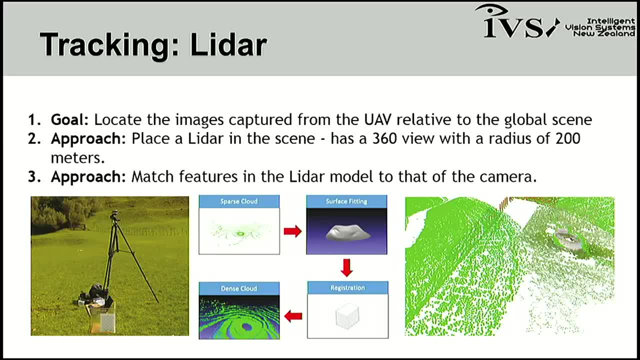 connected. so it's part of the work we do. it's basically a registering cloud of points. what you see here is a farm with basically a drone flight with a camera and some lidar imaging, and we try to put together what you see, which is the set. 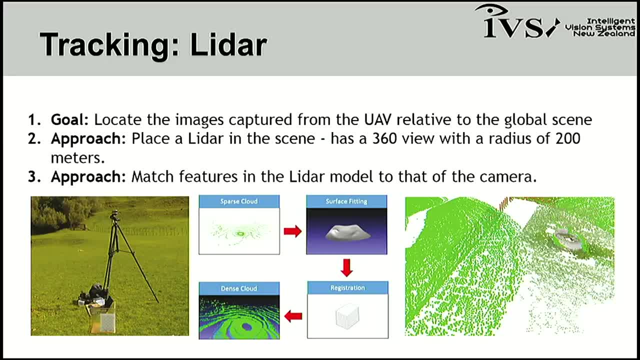 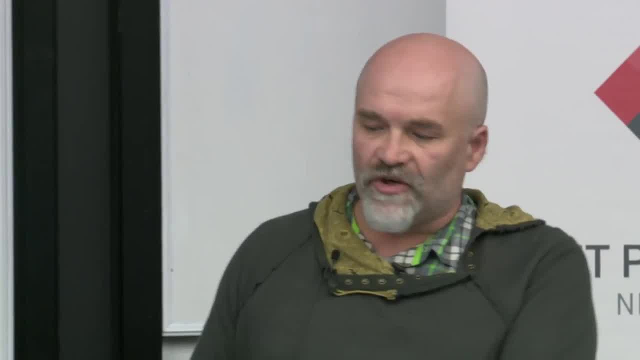 of green points that are lidar, laser lines and the colored ones, actually what you saw from the camera system. so, mapping together these systems, now imagine if you could have. so the problem with lidar: so far they're a bit expensive to work properly, so when you fly them you must ensure that you don't crash- and we do crash a lot, so you don't want to take $10,000 lidar with you to do that too often. but very soon- I hope so it's getting there- we'll be able to fly these combined systems on bigger, better drones. 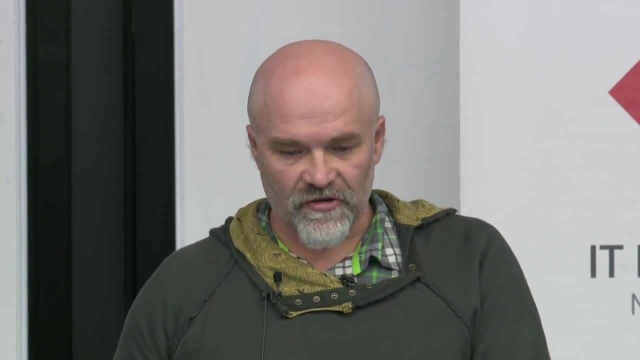 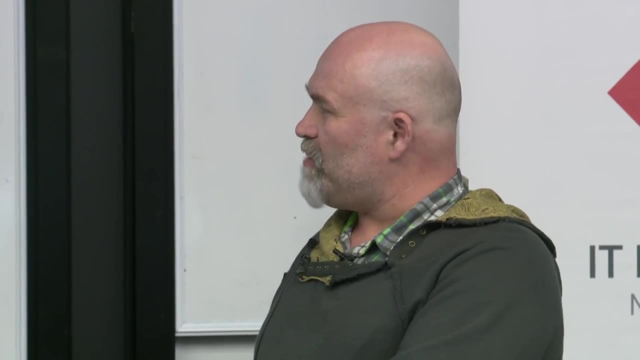 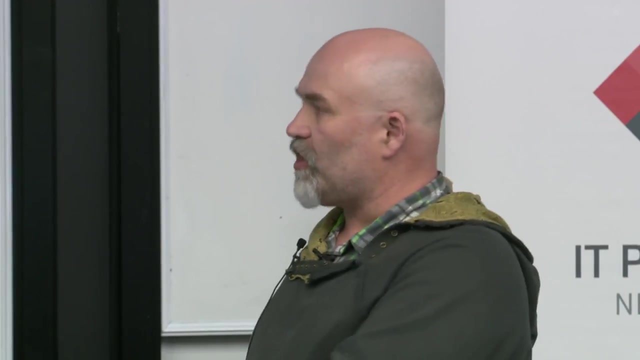 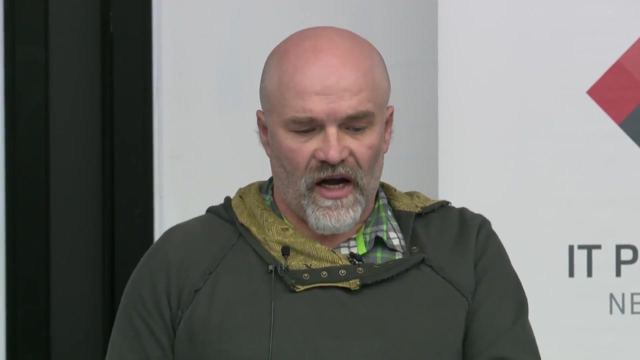 that don't crash. this means Patrice is not flying the drone. it doesn't crash. now we need to return back shortly to exactly what we were trying to say. so is robot vision better than human vision or the contrary? or are they both good in what they do and they're basically doing different things? so a few slides, very 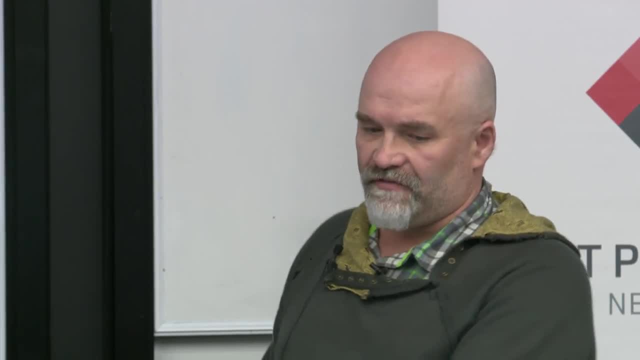 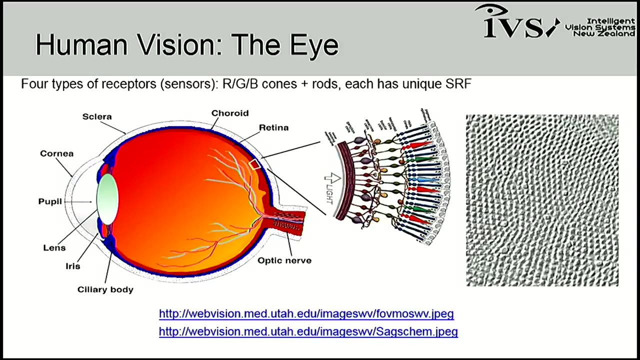 tickle very quick. your eyes have really two type of receptors: sensors. there's RGB cones and there's roads. the cones will look at the color, the roads will look at motion. mostly the TV standards have been modeled a long time ago, in 1931, by the 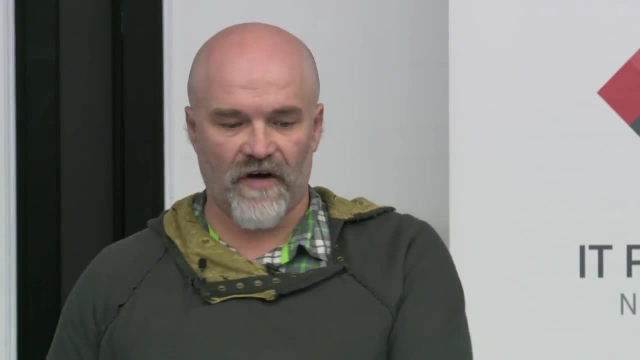 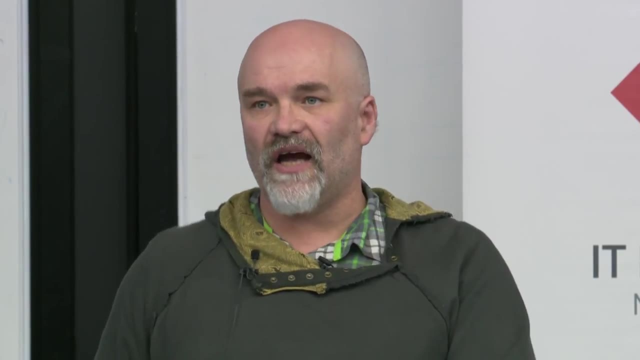 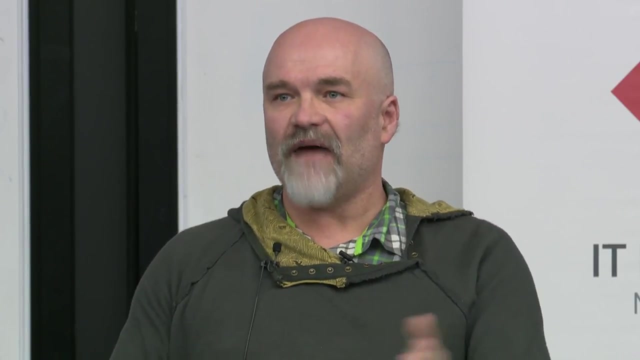 International Commission of electricity, but they were in France, but I was in French and they model, like several color space. they were basically trying to replicate the colors we can see as humans, and with the same type of proportion, because there's no point creating images if they are not adapted. 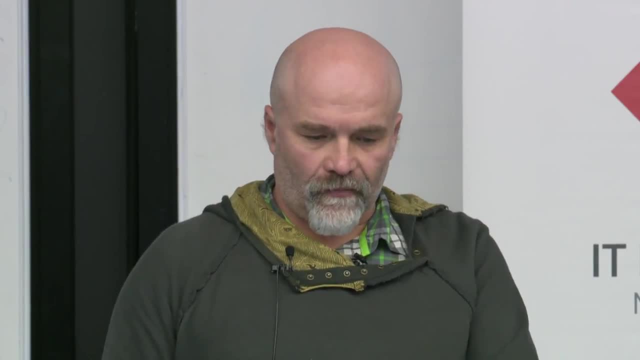 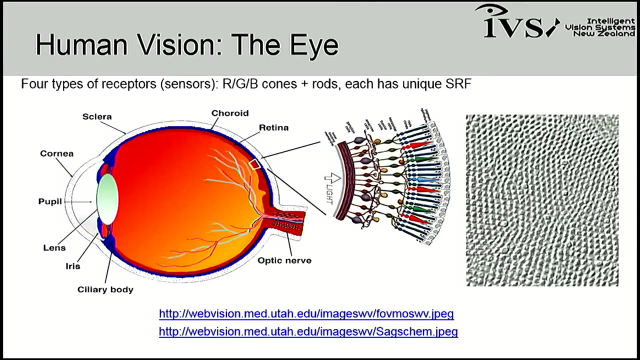 to the human vision. all right, so going further to that, so we have the light entering from one side. do we have a laser somewhere? no, we are not Star Wars proof yet. okay, all right, the light enters from the left, goes through the lens and hits the back of the eye, where 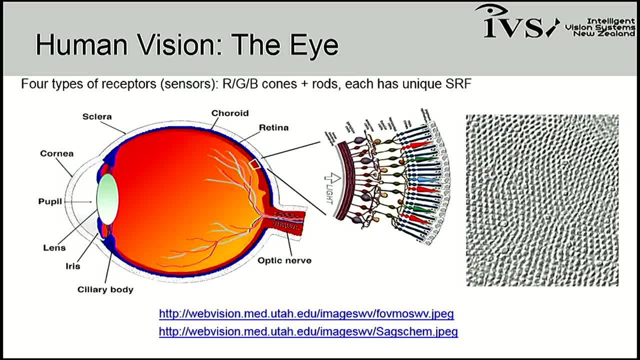 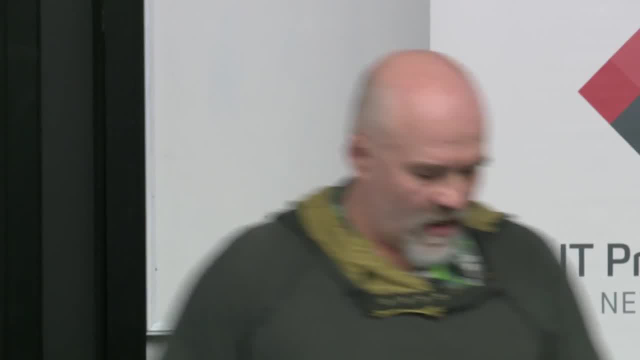 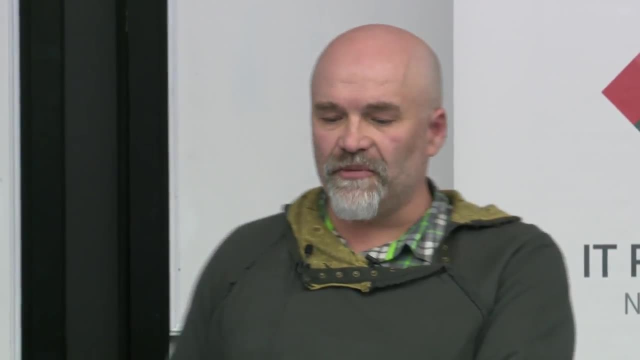 it creates electrical signals, they'll go through several layers of computation and go through a set of neurons, be processed and hopefully create a some interesting patterns that the brain will try to make sense out of it always hitting the wrong one. okay, now the first. if we would look at what's the 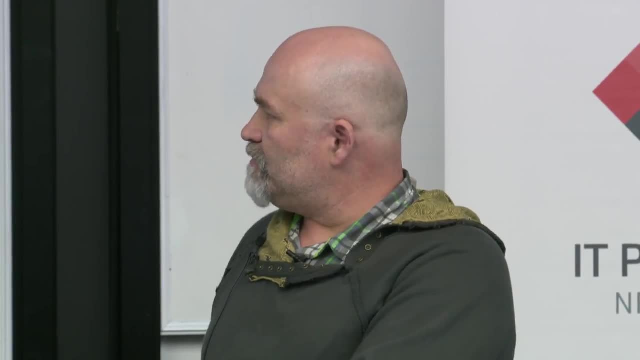 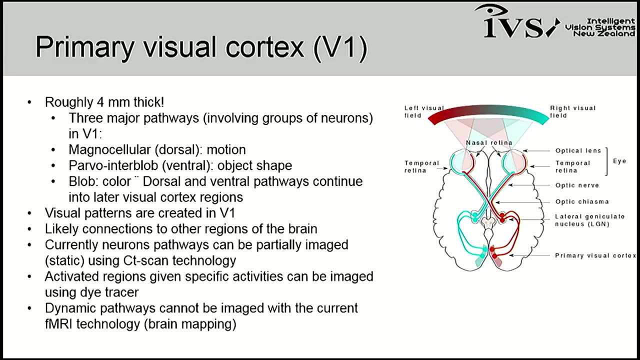 most important what's where are things happening? so I have the chance to work with the group, to have worked or continue to work with the group in Japan, are extremely versed in the visual systems and they're trying to understand the different layers, so we'll not go in details. we have the what's called the 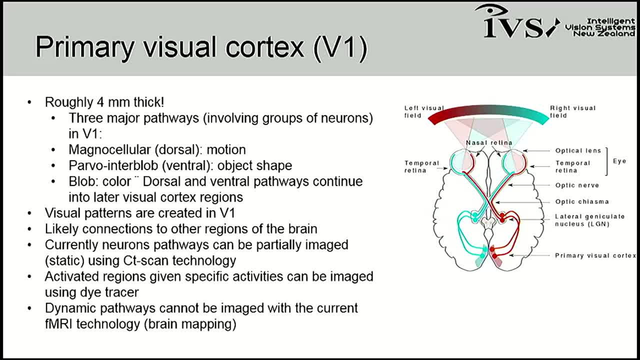 primary visual cortex, which is at the back of your brain actually, and where the nerves- optical nerves- are conducting all the signal, and there will be three type of pathways there and connections that will interfere, mix, and there will be the ones dealing with motion, the one dealing with object shape and the one 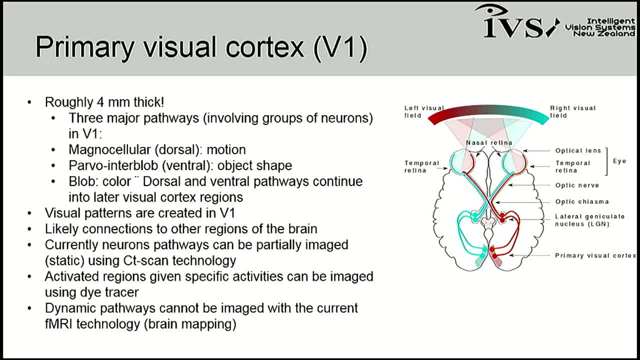 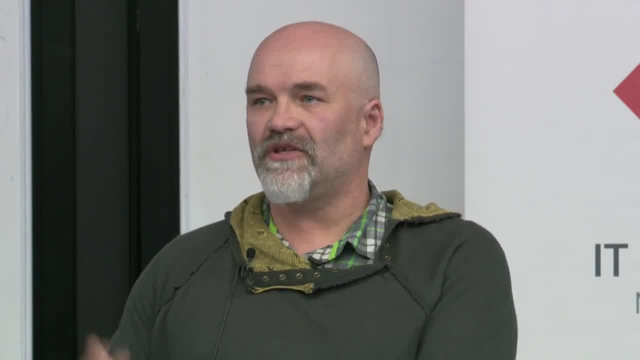 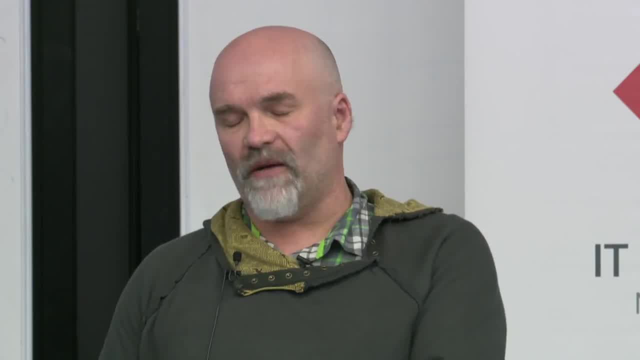 dealing with basically color. now there's some interesting papers dealing with people having brain trauma and see how it affects the way they see the world. it's quite interesting. there's some people that cannot recognize shapes. others- there's more common- do not recognize color, so you can have some. 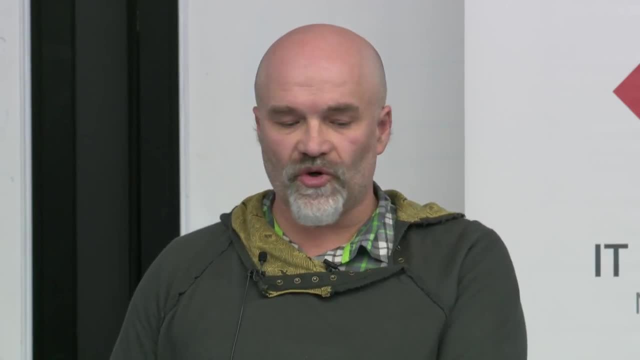 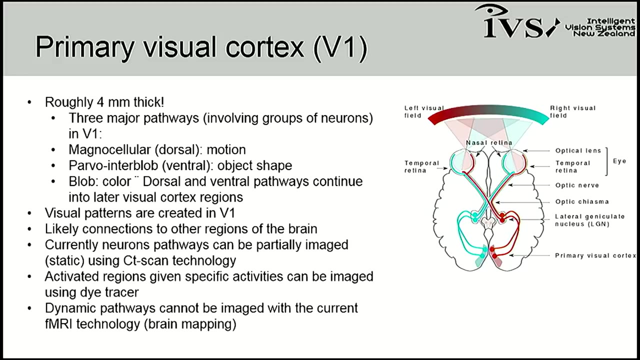 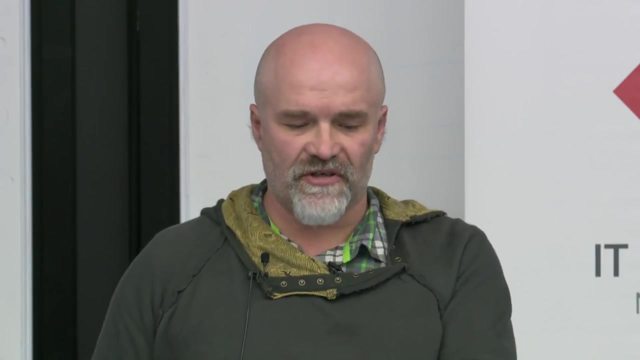 very strange things and also in the primary visual cortex is where you create patterns, visual patterns. there's a fair amount of work around. why do you see patterns? you know, when you close your eyes quickly and you reopen them and it's fairly bright, you can see some patterns in there, but it's the process. 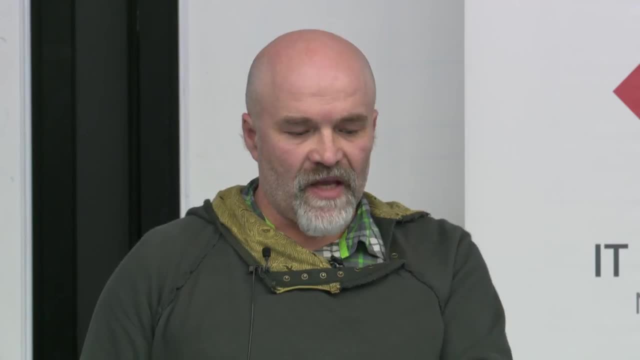 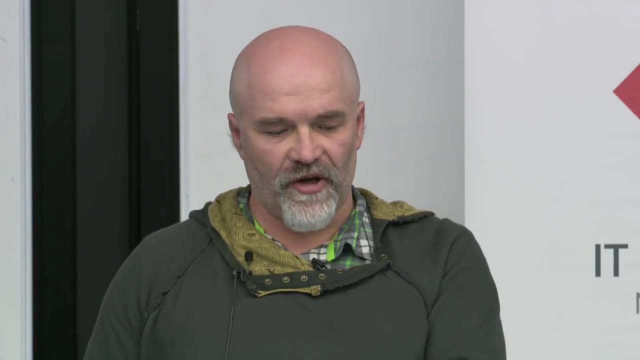 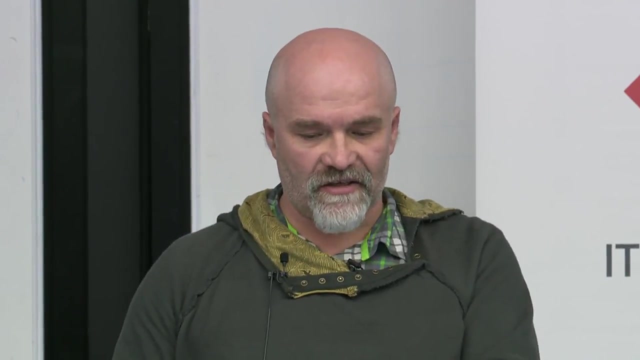 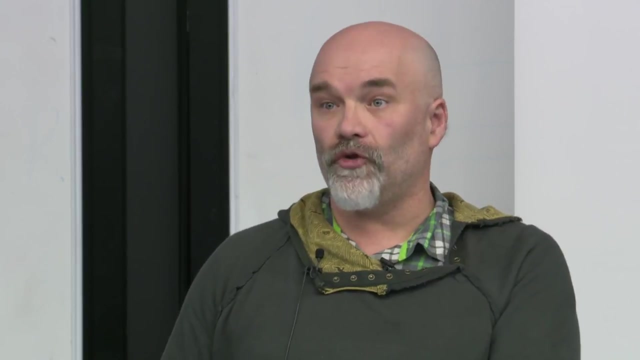 is happening in v1, the primary visual cortex. the problem is you cannot just open the brain and just like see all the the pathways and imaging capabilities we have are not necessarily adequate yet. so, as today, we cannot say we know what's happening in the brain, about vision, we have ideas but we don't know exactly. 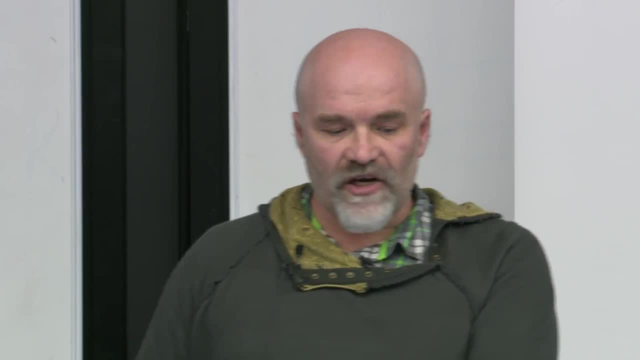 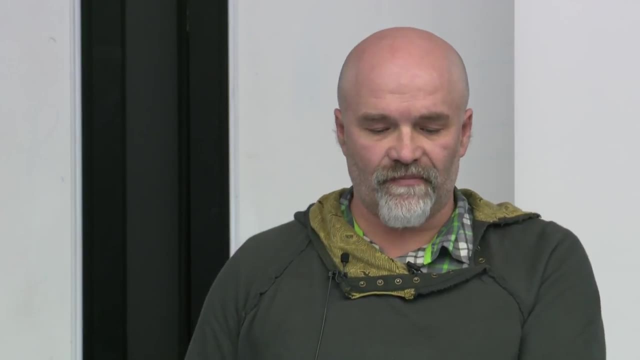 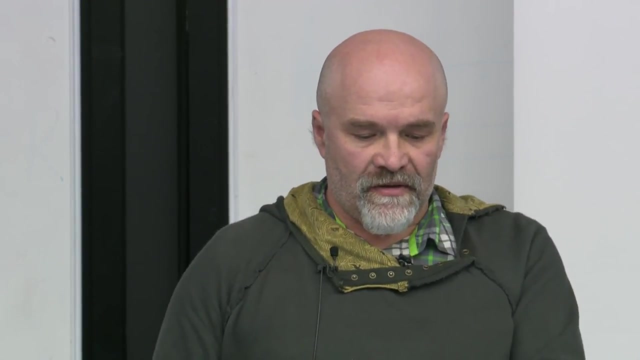 so we do have theories. it's likely connected to other regions of the brain interfering, so what you can do is have pathways using CT scan technology. we might have chance to talk about that. maybe not some regions. when they are activated you can actually see them through fMRI or dye tracer, which means 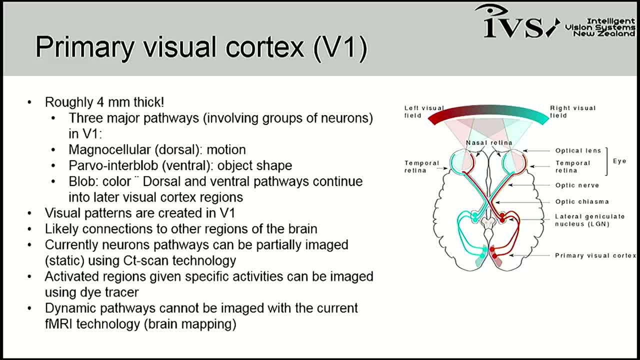 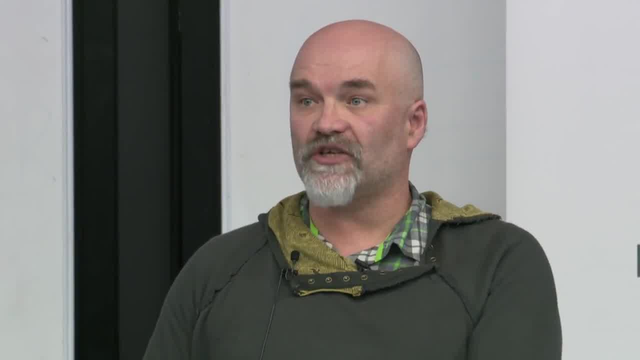 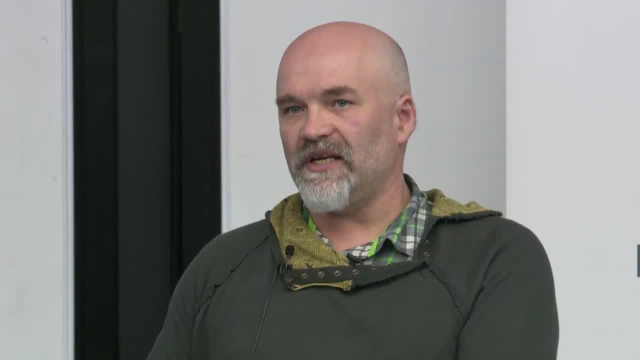 you can see which regions will be activated, but you cannot, Nestle, say that neuron will do this and connect with this, this and that. that's what a brain mapping projects are trying to do at the moment. sadly, they have to use monkeys to try to extract as many brains as they can and try to image that. but hopefully 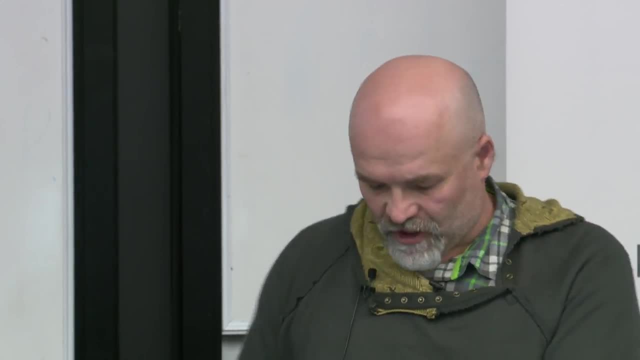 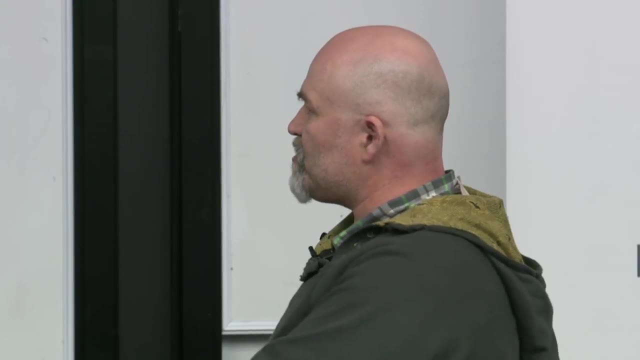 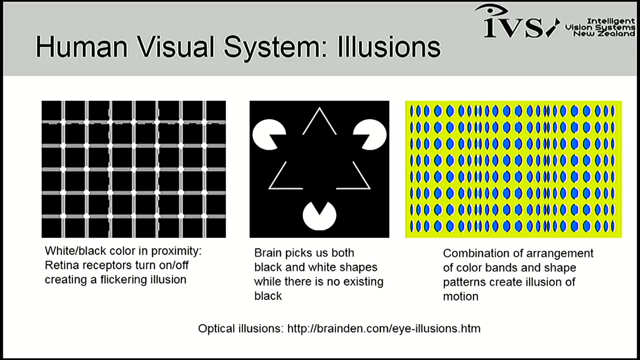 it's for the best. so so far we have ideas we don't know too much. right, some illusions, because it's always great, so everyone should have some. on the first one, if you stare at the blobs in between the lines, you should see them like white and then black, and then they should be flick around. can you see that? 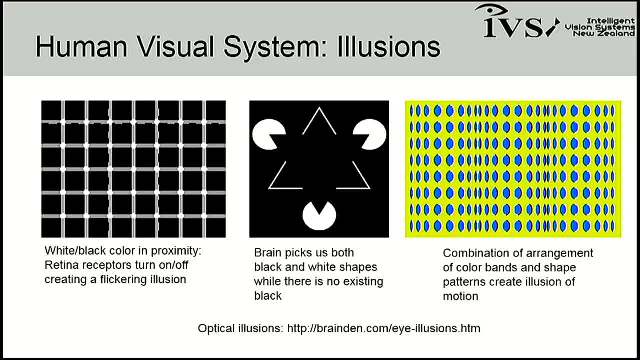 so, apparently, as the white and black colors may switch on and off your receptors, and since they're very close one to another, if you just move slightly your eyes, you can like switch on and off different ones and the dot starts to flicker. is it working on the screen? okay, it's. 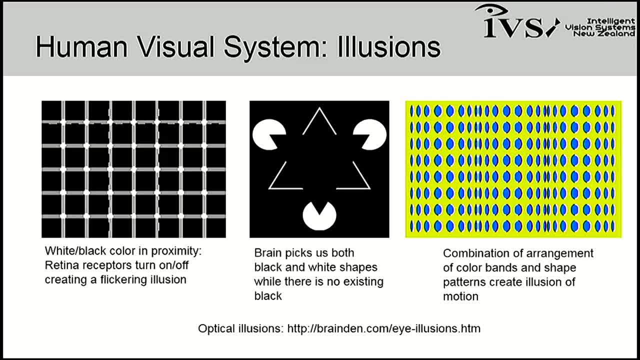 not working for me, something wrong with my brain. the middle one is the one I like the most because I struggle four years with techniques trying to actually extract something out of that. none of the shapes them are complete. you can see, well, actually, the big triangles, they, they don't really exist. yet you can. 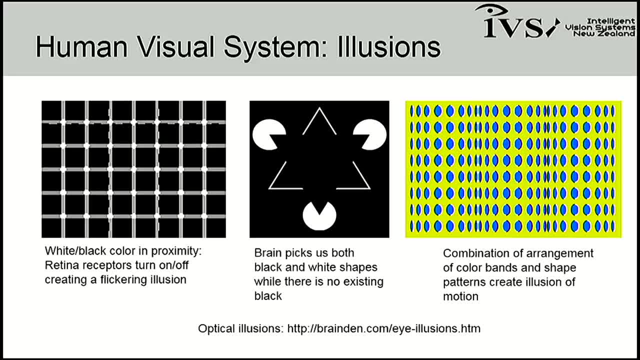 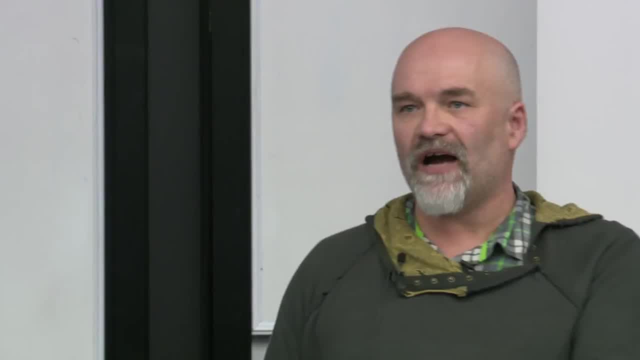 still see the black triangle really really well. do you see it okay? so if you try any techniques in image processing, computer vision, try to extract these triangles. good luck. it's not going to work well, but it tells you a story. it tells you that whether the shapes are black or white, you can see them while 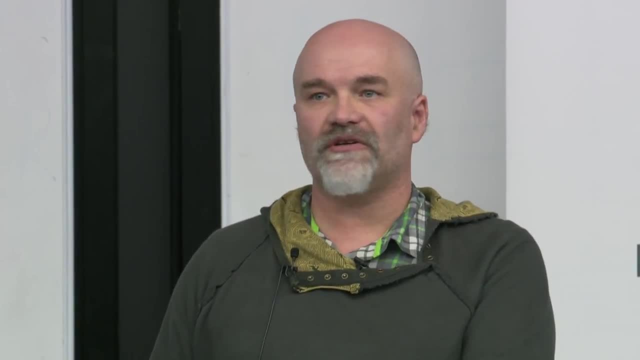 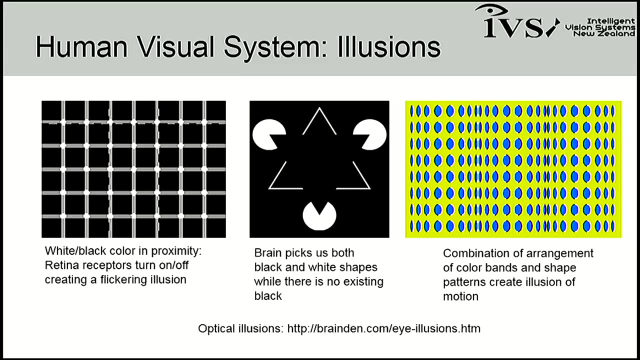 computer vision systems. if it's black, there's no information. you're not going to see anything right. these contours that you see, of that triangle, the black one, do not exist. you form that in your brain. there is no information in the image, making you being certain of that. now the last one. 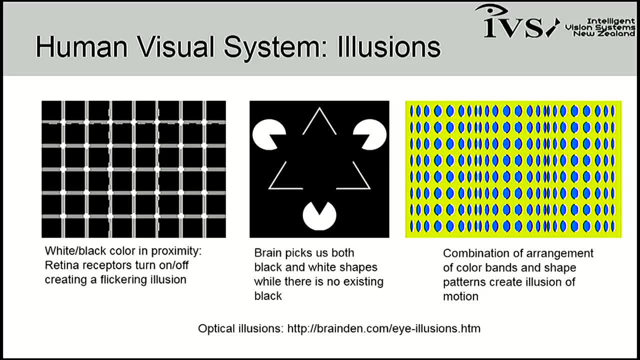 this one is a bit yeah, so you should see the wave of different colors. so there's three different illusions related to the way the different receptors on your brain are connected locally and how they deal with the arrangement of colors and shapes to create an illusion of motion. so there's these switching on and off. 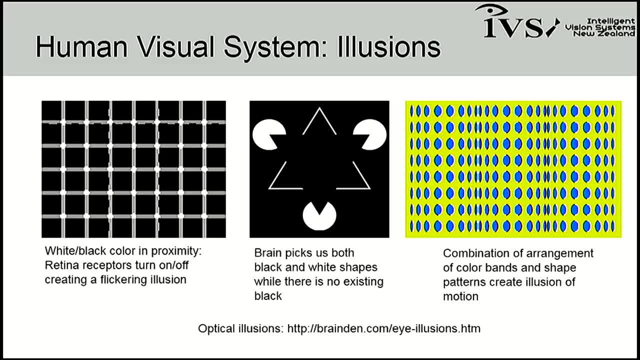 for different colors that are very close one to another. that creates that. I think there's a Japanese specialist of all illusions. there's also that website has got a lot. they do not provide explanations, so you have to do a bit of digging to get around that. robots have their own. 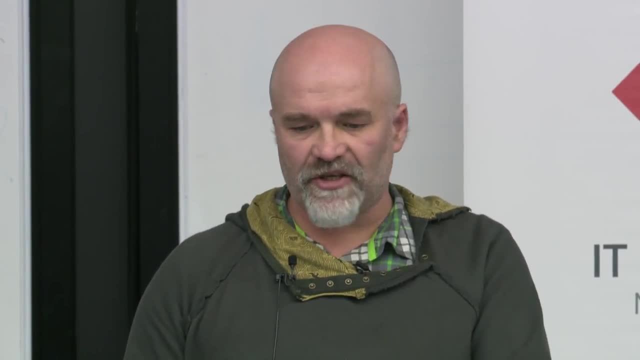 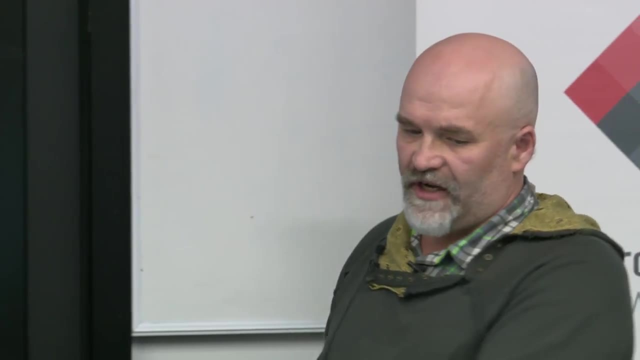 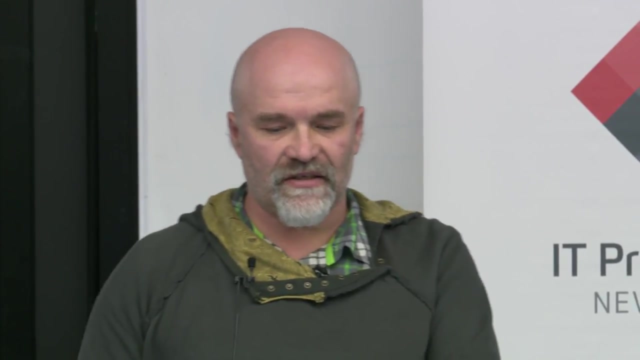 illusions as well, depending on the resolution of the images. but I didn't bring any. all right, let's move on. so I'm all. let's say a lot of things, so we don't fully understand what's happening with the human visual systems. we have some ideas. we have limited color resolution might be. it might be more. 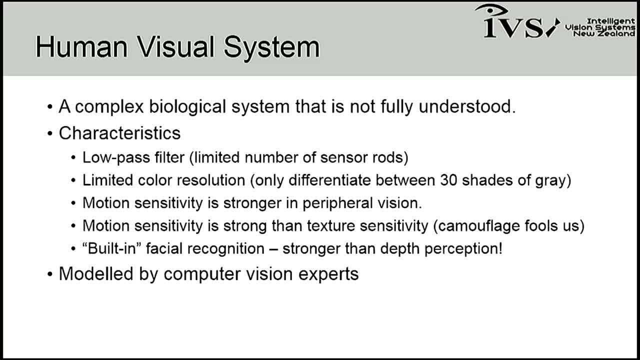 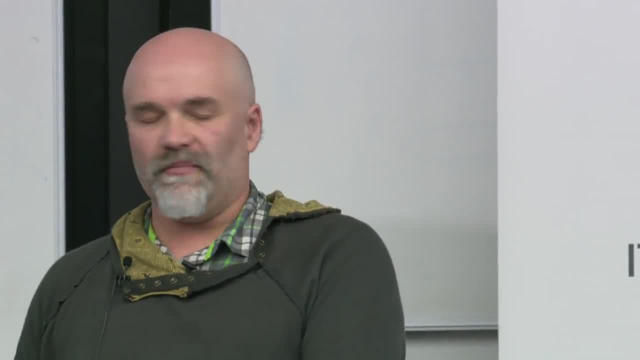 colors, but in terms of shades of gray, you cannot see much more than that. we do have shades. well, we have color meters and gray meters in the lab, which are printed sheets that you can look at, and they have 256 different shades of gray. you cannot see all of them, so that's a good way to test your, your. 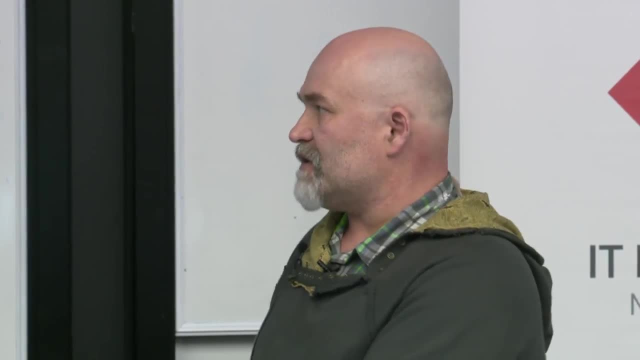 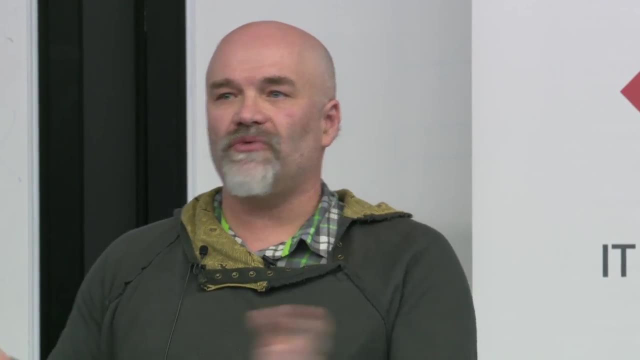 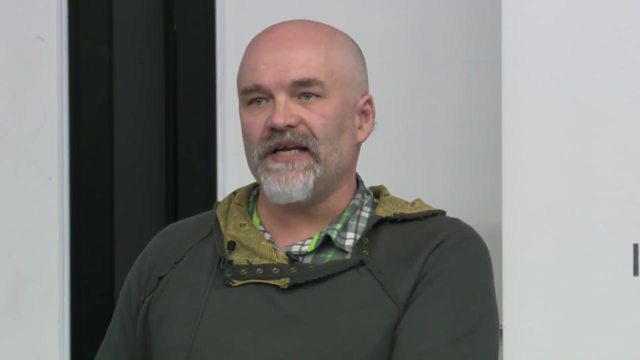 vision. if you think about when you see motion actually at the periphery of your eyes and if you think about it, you now maybe understand, because you know we humans but we were born animals so most animals will have similar capabilities. Often when an animal is looking for a predator. 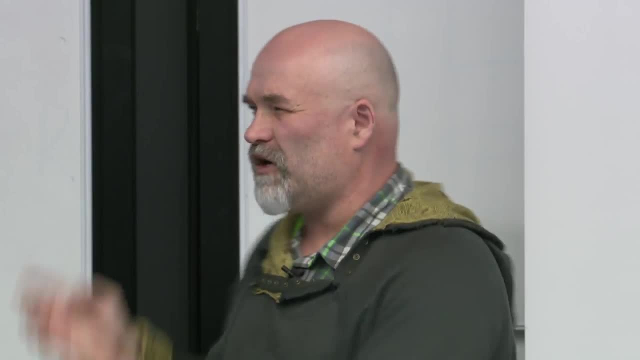 they're not staring in a given direction. so when a bird looks at you, they don't look at you straight like who are you, They look on the side, and they look on the side to try to really get you on the peripheral of their eyes. 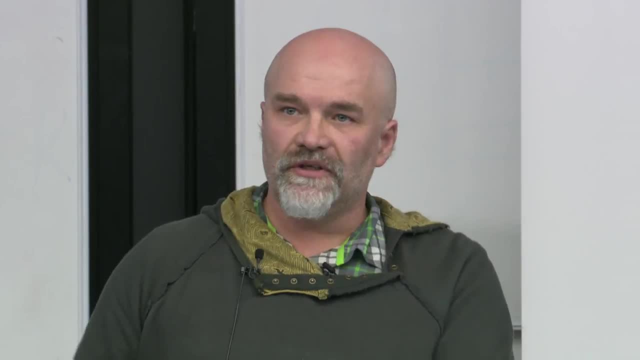 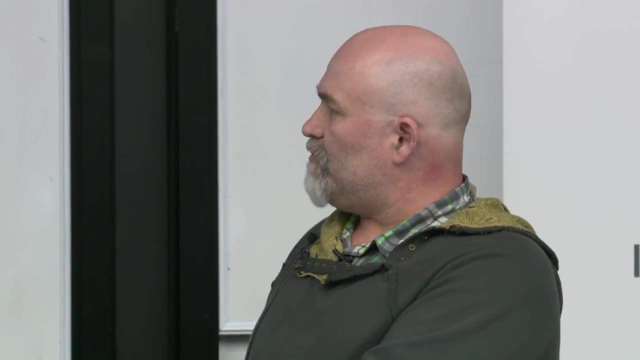 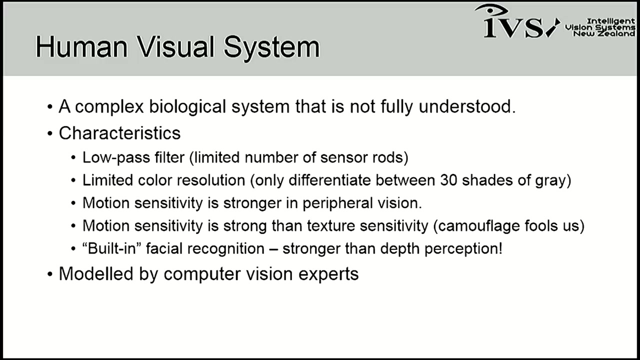 The motion. If you don't move, they won't move. If you make a move, they'll just go. That's coded. So basically, motion is stronger than texture, Maybe because nature never invented an animal that could have strong texture camouflage. 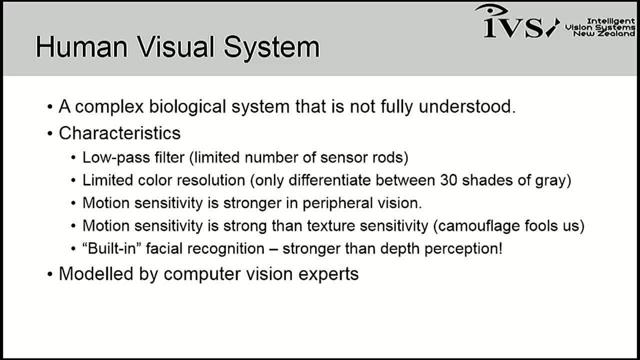 but it could be fast-moving predators. so we had to evolve with the capability to have motion detection rather than texture And something very strange, which is we are social animals. We were built and evolved with the built-in facial recognition, which is pretty strong and stronger than capabilities to detect depth. 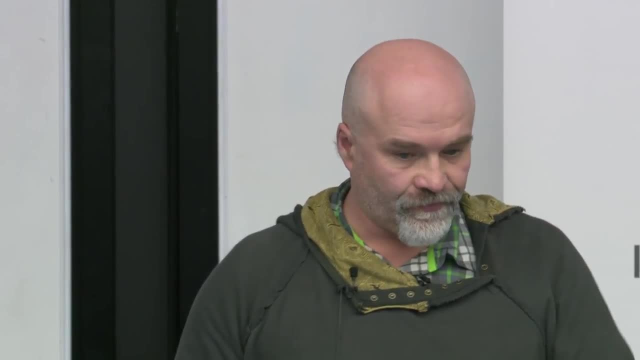 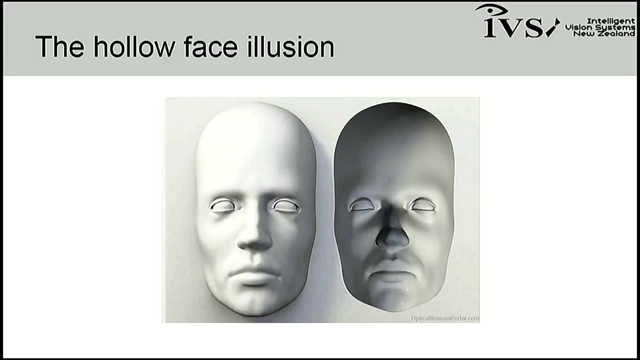 Alright, so an example. So um, you see two faces Here. yes, So everyone sees two faces. That's good, No problem there, Except that if you were to see the depth of the face, one face pops out. 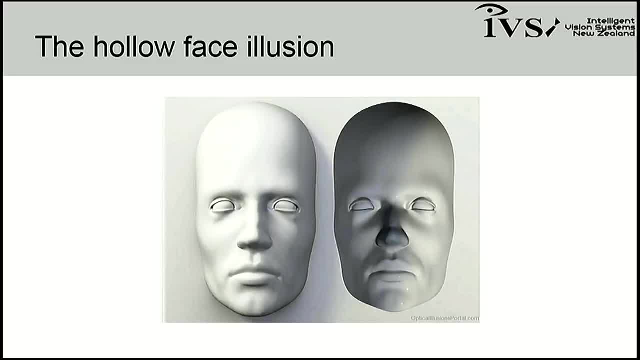 and the other one is inside, Alright. Yet what you see is two faces and not much the fact that one is going inwards and the other one outwards. Alright, And it's basically why it's called the hollow face illusion, So we code it for that. 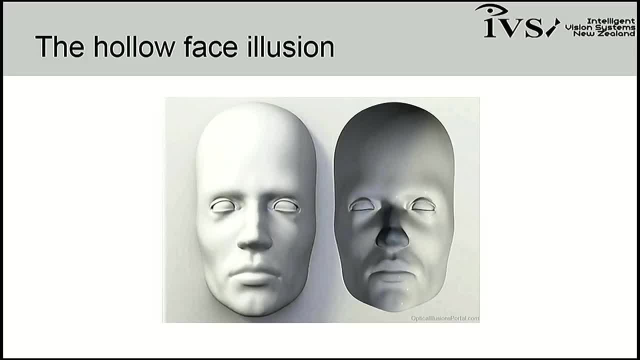 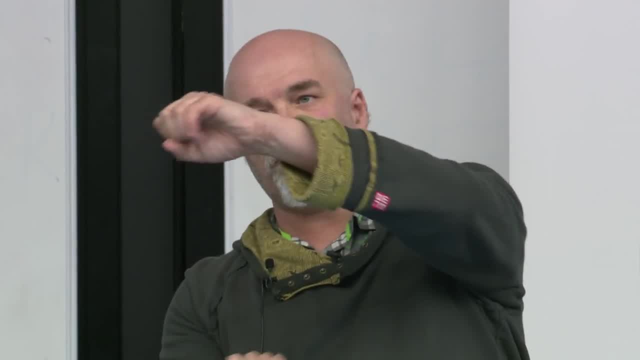 Alright, And it's basically why it's called the hollow face illusion. So we code it for that. Surprisingly, we have a built-in ability to recognize faces, but only in one direction. really, Just the right one. If you take a face, you put it upside down. 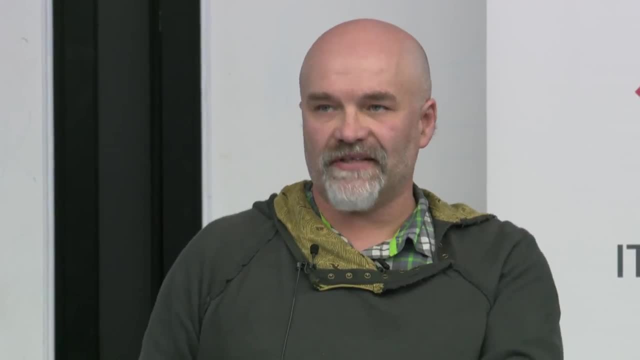 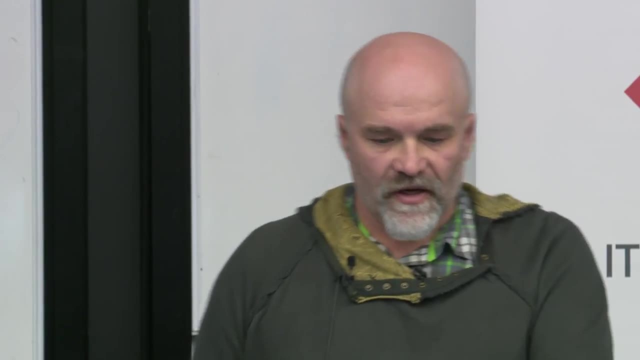 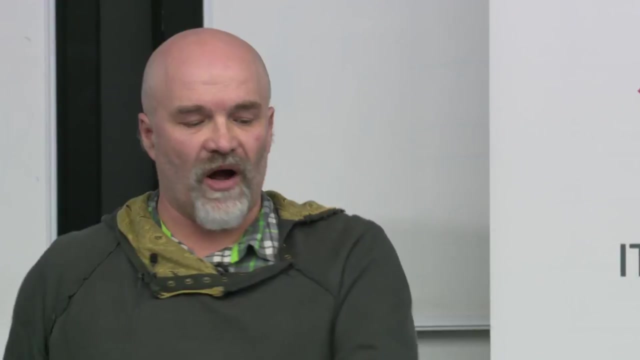 we can't recognize people anymore. So that's pretty strange in some ways, Or it's not Okay. so we like to draw boxes when we do algorithms, because it's one box after another dealing with different problems. It's really good as well, because that's what we do for algorithms. 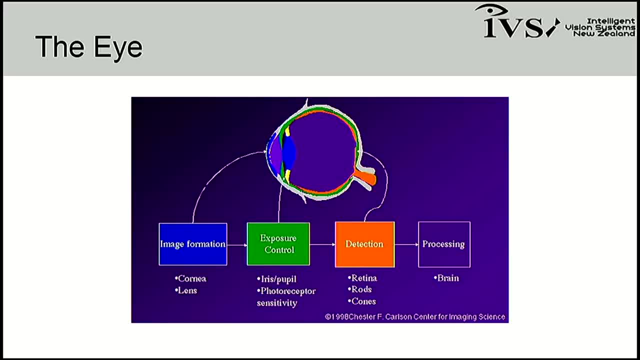 Where do we form the image? What are the problems? So lenses often have distortions and some of us experience later in our lives need to correct distortion of their lenses. There's: how much light would you like to expose? and the human eyes are really beating any robot vision in that. 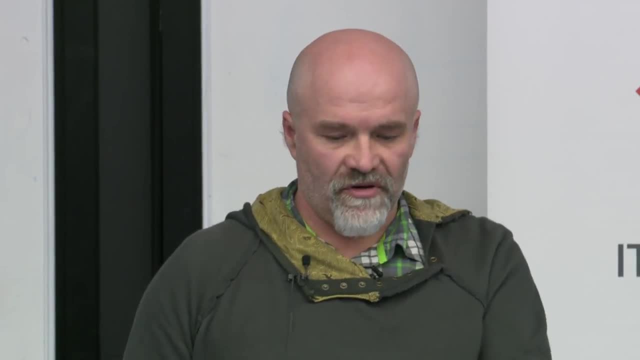 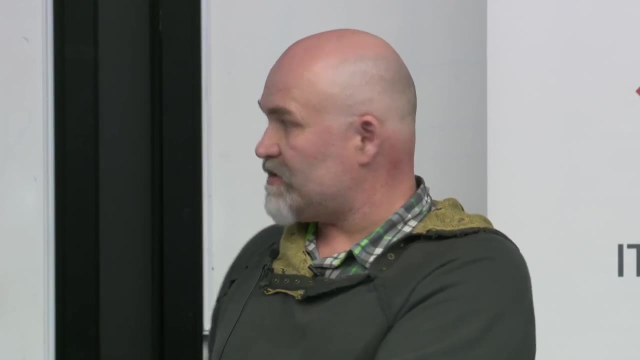 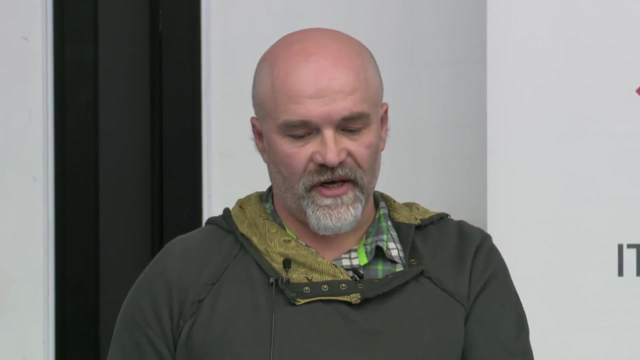 direction, which is we can adapt to the light the amount of light you have in a real environment, much better than cameras, And we can locally adapt, which basically the cameras, most cameras cannot do. They are very expensive. We don't have any At the back, we have a. 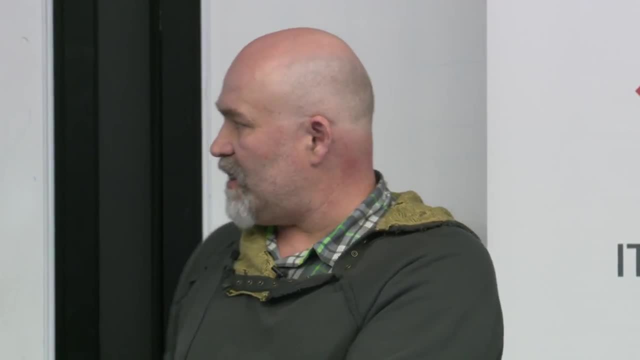 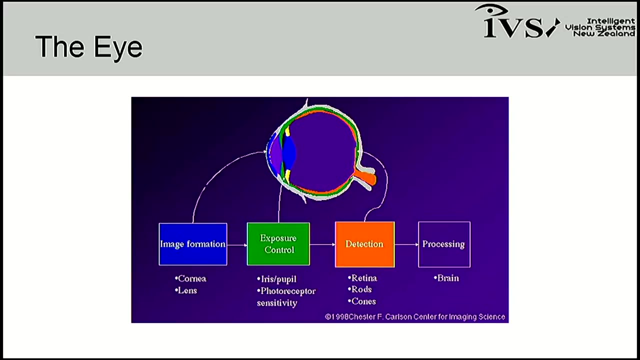 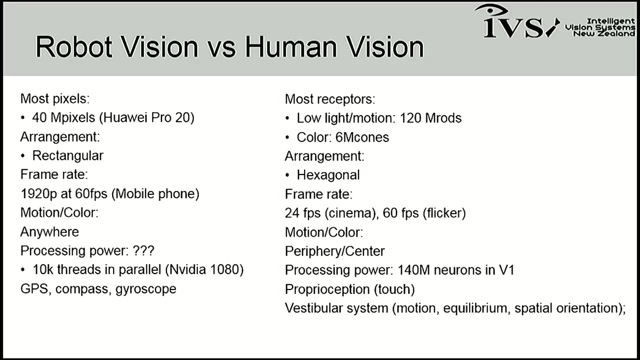 sensor. It's basically how we see the retina, roads and cones and the processing brain. Now we discussed- and it's basically often a challenge and an open discussion- Who beats who. So let's try to see that And then after that I'll talk about other things. So if 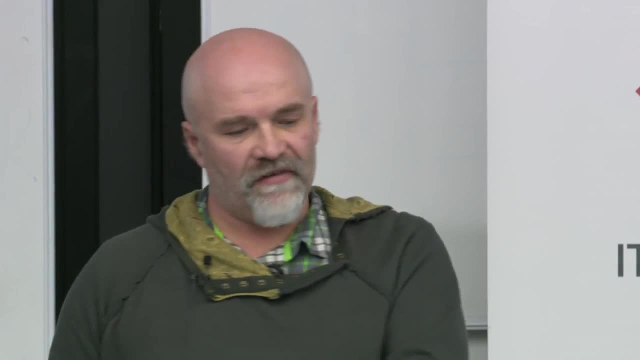 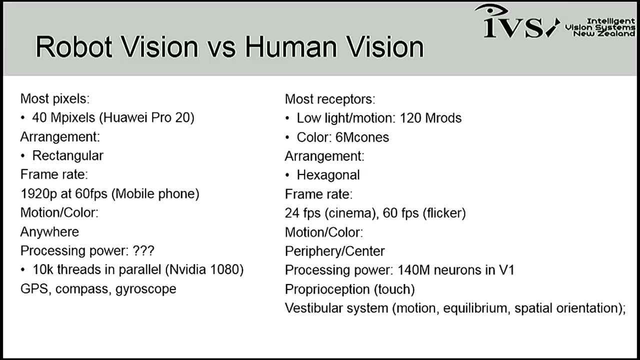 you've had enough, you can go. There might be some wine left, but if you want to stay, it's good as well. Who's got the most pixels? It's good I make someone laugh. That's great. I love that. Most pixels. the Huawei Pro 20, one of the cameras got. 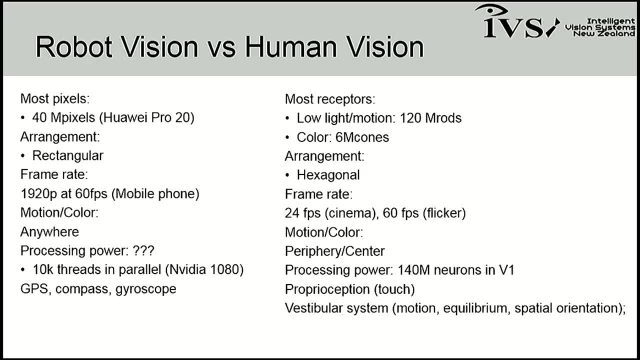 40 megapixels. Don't ask me what for, but that's that And it's on a phone. What about our? for the low light and motion we have a lot under 20 millions, but for color we have only six millions. beaten for at least color. Arrangement of cells for. 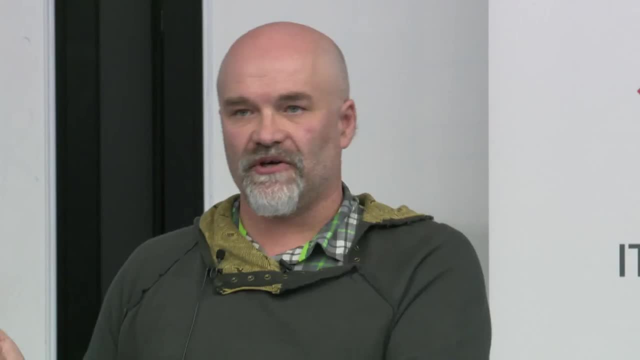 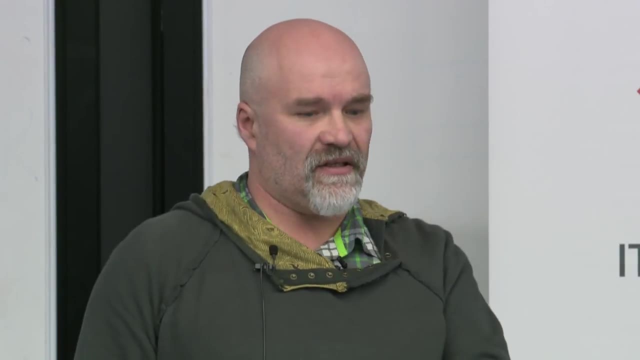 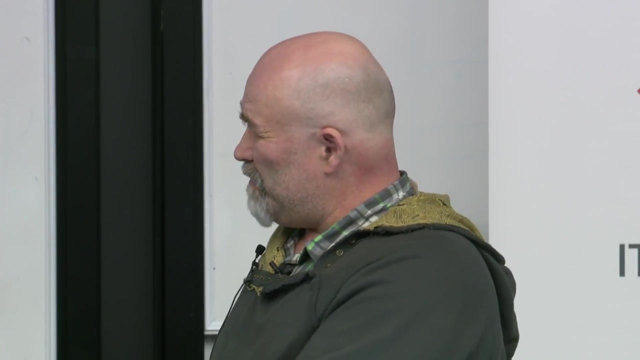 cameras. as rectangular, you will have pixels after pixels in rows and columns. there was a bit of fooling around with hexagonal distribution but in terms of making that in electronic pattern that was not successful. but the mathematical description of images with hexagonal patterns is extremely nice, because all 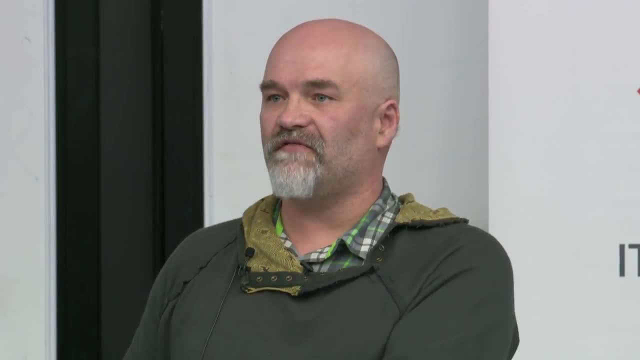 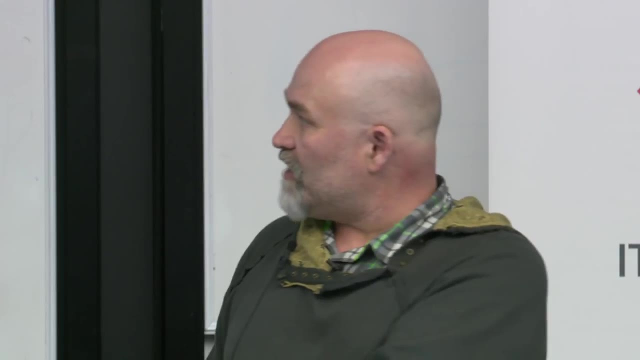 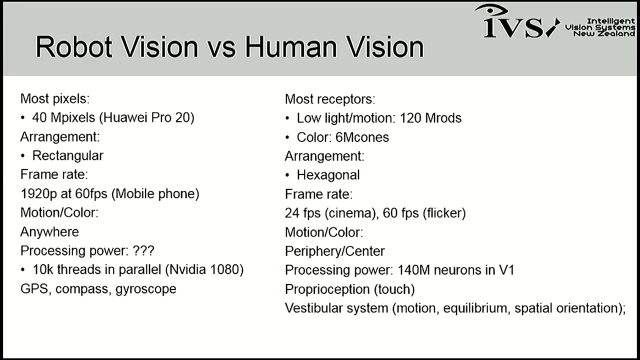 pixels are at the same distance one from another. it makes things very simple. The arrangement in the eyes is hexagonal. you'll have different cells for different colors, all arranged in that way. What about frame rate? Mobile phone will do easily. 19-20. 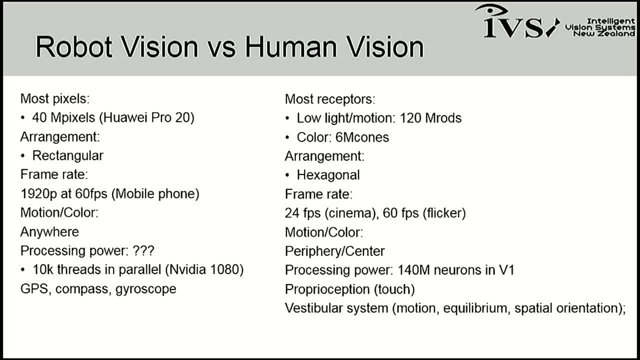 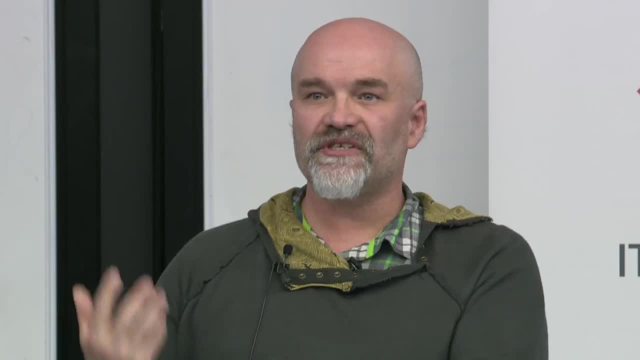 P, so it's 19-20 by 1080, by 1280, sorry, at 60 frames per second. For the eyes it's a bit different. it depends exactly what you're doing. 24 frames per second will be the movies. If you have a flickering phenomenon, it disappears like we don't. 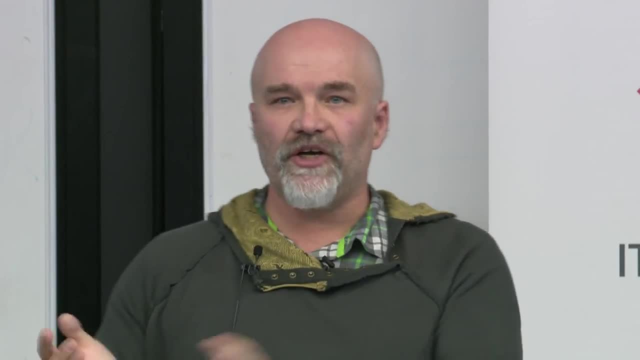 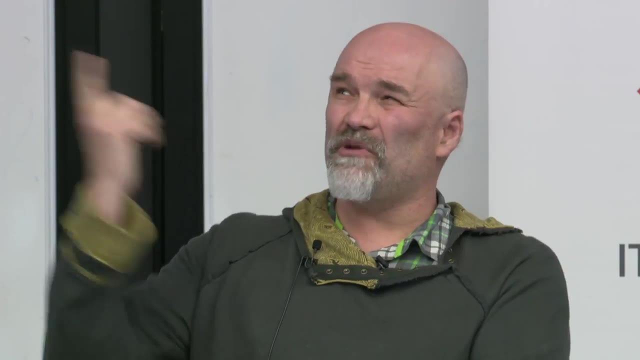 see it blends in from 60 frames per second and we are not all equal with that. some people are more- how can I say you can be more disrupted with some of these lights when they start not working with their flickering, and some people will be able to detect that. 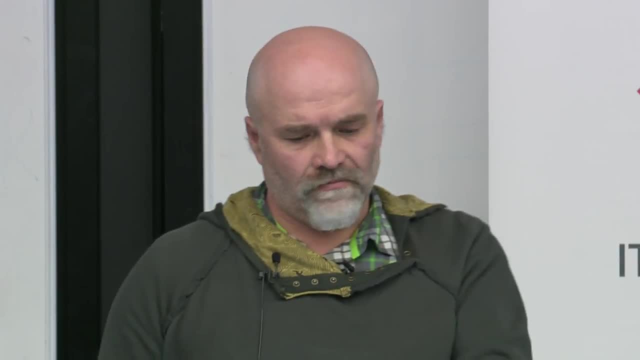 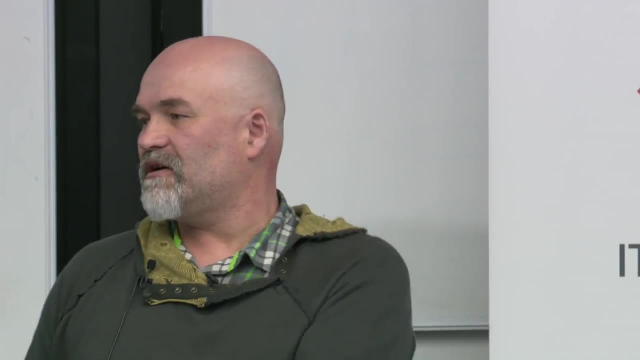 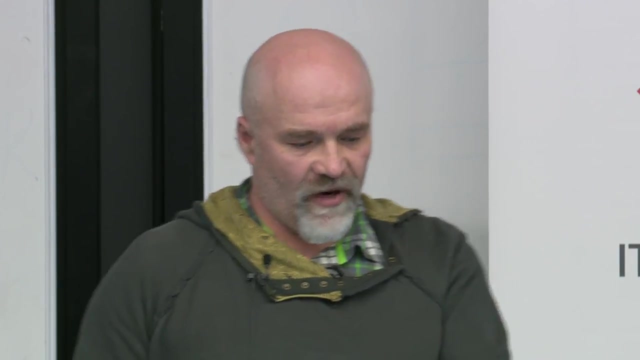 and others will not see it. so we are not all equal there. Japanese anime may have more than 24 frames per second. gamers will say you need to have up to 120 frames per second. but gamers are not humans anymore. I used to be a gamer, I know all about it. 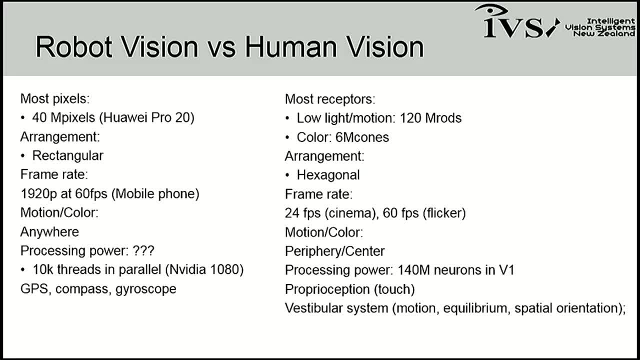 What about motion and color? Well, for the camera it's everywhere. because it's not on the camera, You need to have a processor. you can play with that on any pixels and of pixels. for the eyes, the motion is really the periphery and the color is the center. all right, 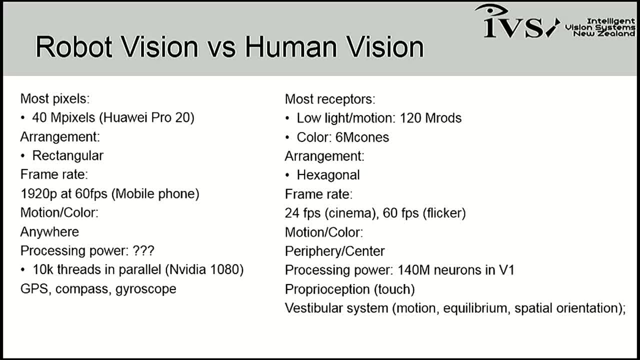 so it's really about that. what about the processing power? let's look at the brain. just on the primary cortex there's 140 million neurons. all right, what about the most the most powerful pile processing card you can buy for yourself or your son when he says it's for work? 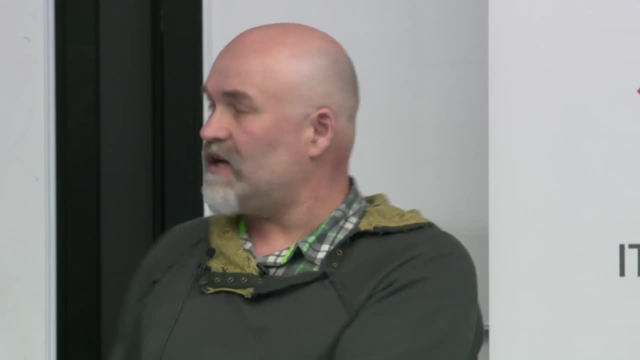 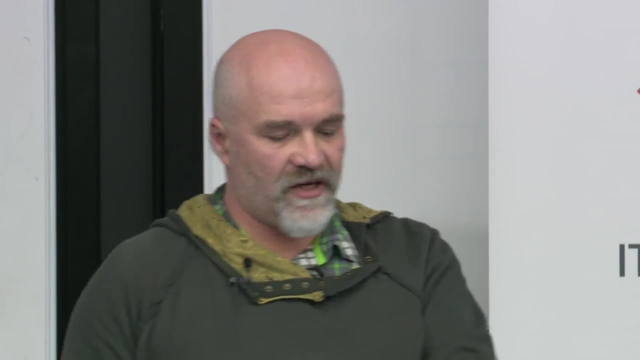 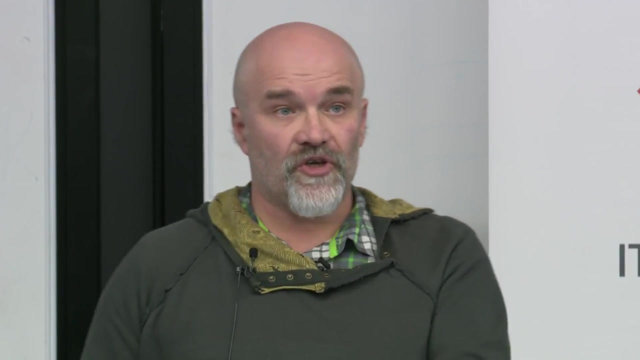 it's actually for gaming. don't get fooled, it's an nvidia 1080 ti. you can do 10 000 threads in parallel, so 10 000 operations, or set of operations, in parallel. so you see, the brain behind our vision and human vision is not just the eye, it's also the brain, it's definitely still. 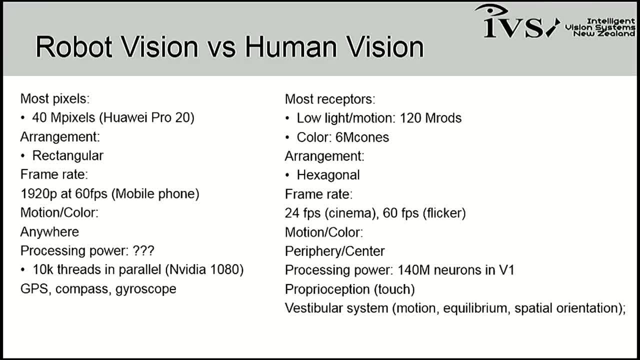 better there, and that's why we're still beating machines and robots when it comes to understanding the world around us. we don't have enough yet, some people might say. but hold on, it's not enough. we don't just see. we exist, and if you take a human, 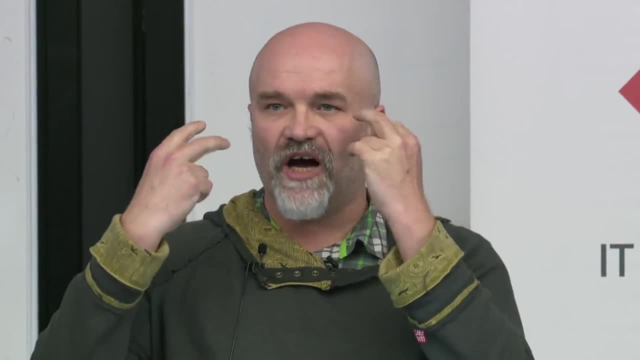 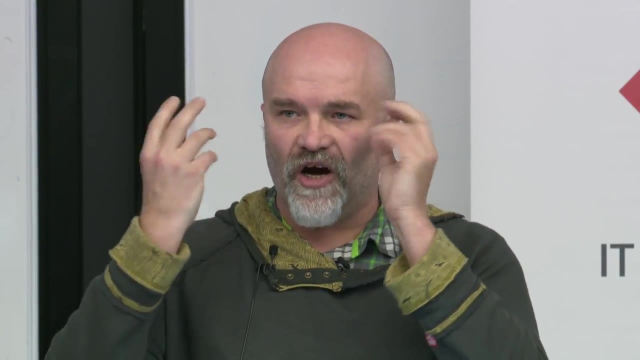 so that's an experiment that's been done. if you take a human and block the eyes with some drug-induced um phenomenon, so you block the eyes, you become blind. your eyes have to move all the time a bit if you're in a room and you lose capability for touch. 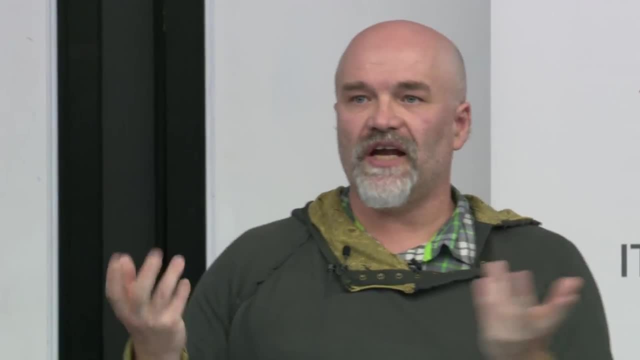 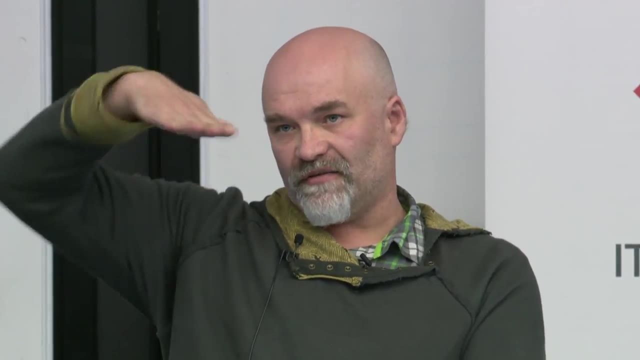 special orientation, you totally lose an understanding of the, of the surroundings. it's why in most planes you will have a way to know if you are upside down or the right way, because sometimes you don't know, your body doesn't tell, doesn't give you the right information. 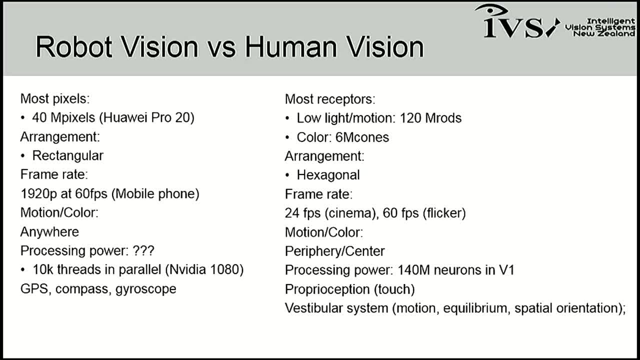 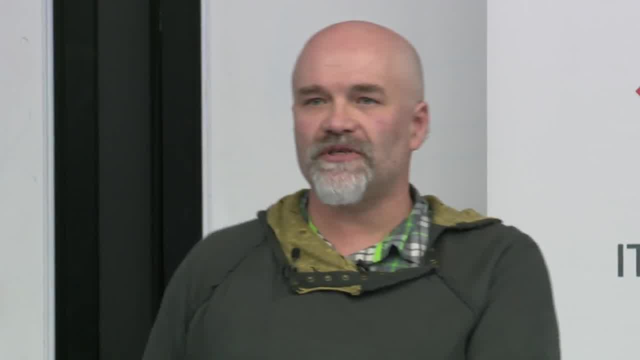 so, humans, we do all that. we need the touch. we play with motion, equilibrium and special orientation. hold on cameras, phone too. we have a gps, we have a compass, we have a gyroscope. so we're not too far there. we have the tools for that. we're missing a bit of processing power capabilities. 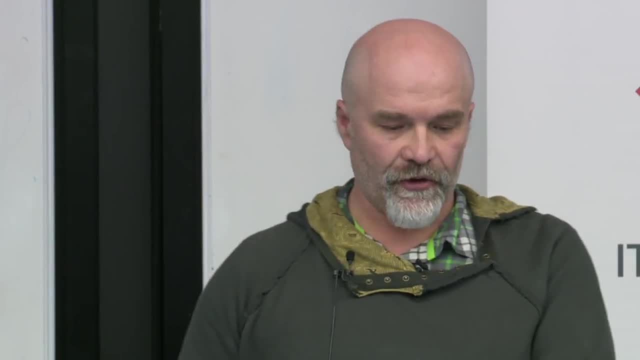 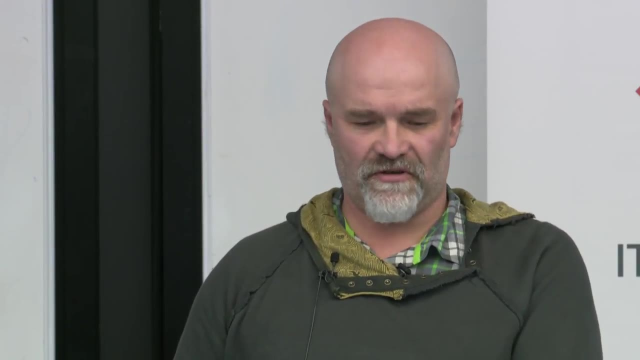 if you ask me a question later about that, a number of years we might need, i don't know, but i think we still have time to relax. we're not there yet, so stop reading these articles in museum herald about the robots beating the humans. it's just trying to force you to buy the paper. um, right now what? 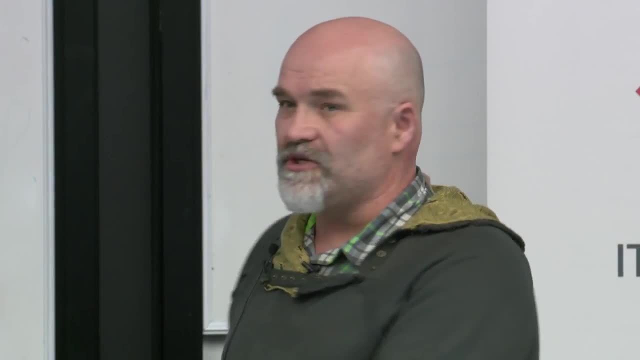 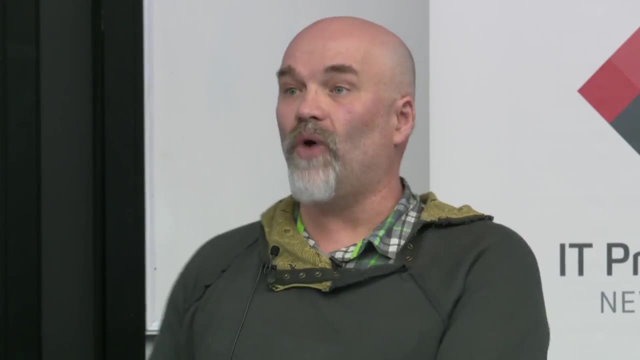 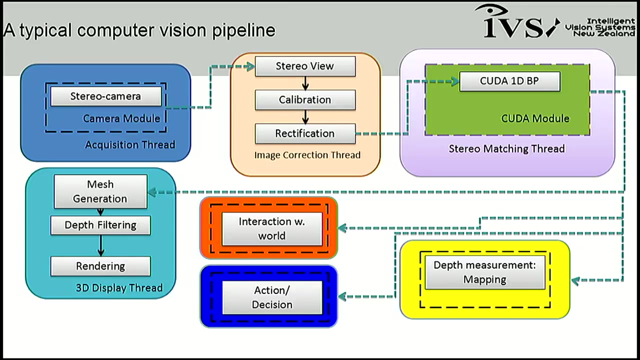 i would like to show you now is: what do we do with what we have right now? what are we capable to do? are we better than humans? are we different? can we do stuff that humans cannot do, and why? um, so i have to put a slide or two that looks like we're doing science right. so, um, this is a typical. 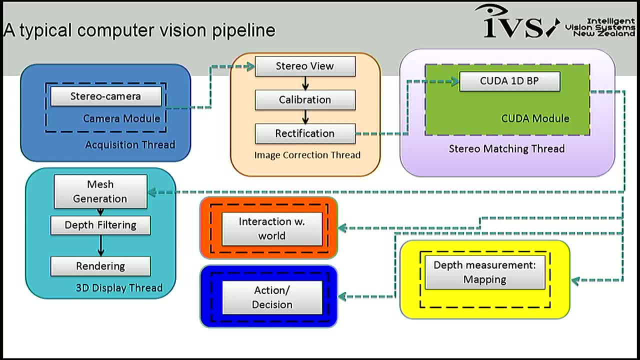 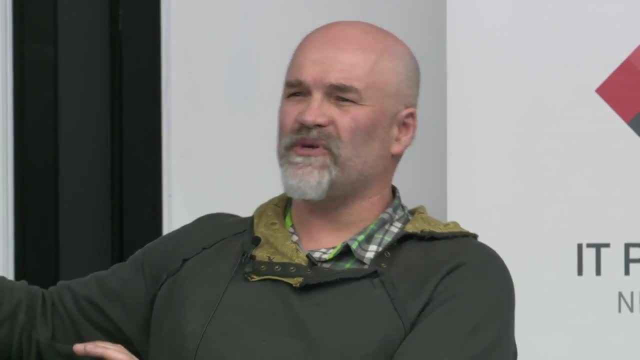 pipeline for us and different blocks relate to different parts that we discussed already. now i'll need a camera, or a pair of cameras, or more than two, to acquire some data. i need to fit that into my system. they'll calibrate that system, say: um, i saw that, but how is the world represented? 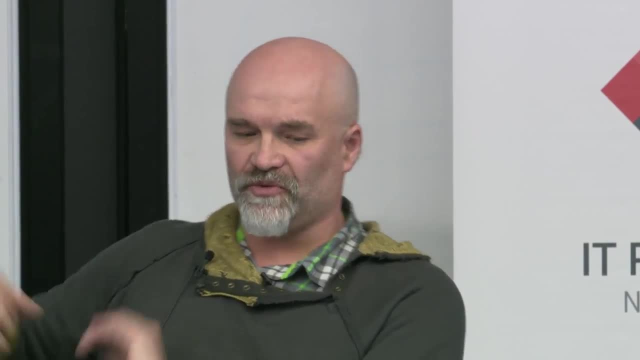 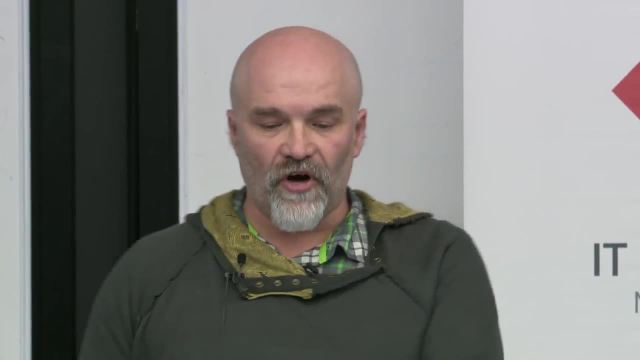 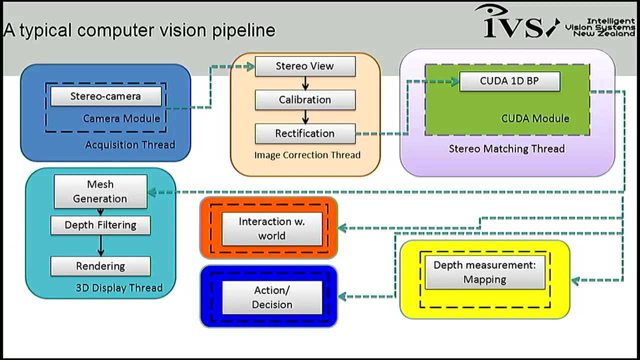 okay, i need an object that will help me kind of make a picture relation between these two. They'll deal with geometrical transform capabilities of the cameras in terms of pixels, focal lengths. Then we need a powerful system that'll just compute all that data nice and clean. So the way to go these days is: 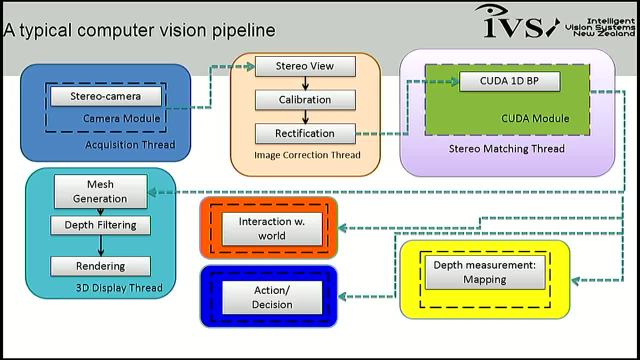 to use a specific programming language, parallel processing and some algorithms that we have developed in-house in some cases, And once you have done that, you like a nice representation So you can have a 3D display thread and we'll see some of that. I think we have a demo later on around here, If you want to. 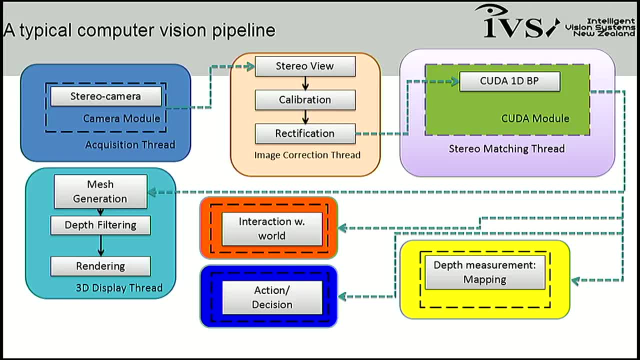 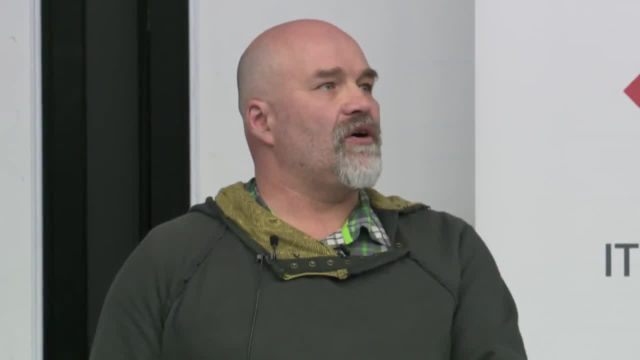 interact with the world. we do have boxes, we have action decision and we have some mapping. So I'll try to show you a bit of applications on each of these. I need to track town. okay, it's up there 7.. When do I stop? I have 250 slides. I can last. 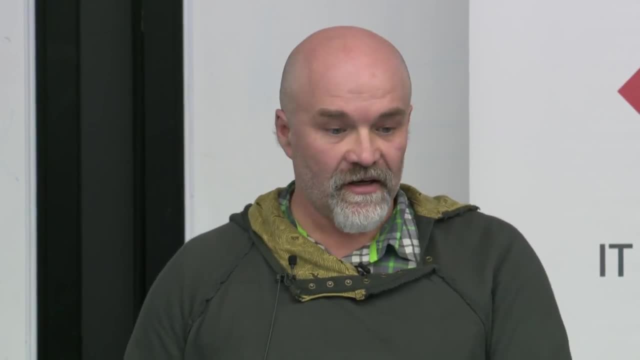 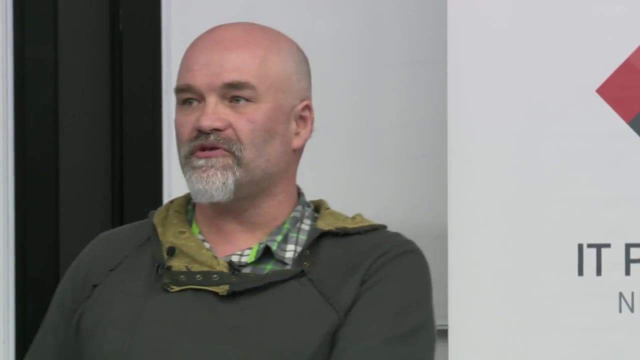 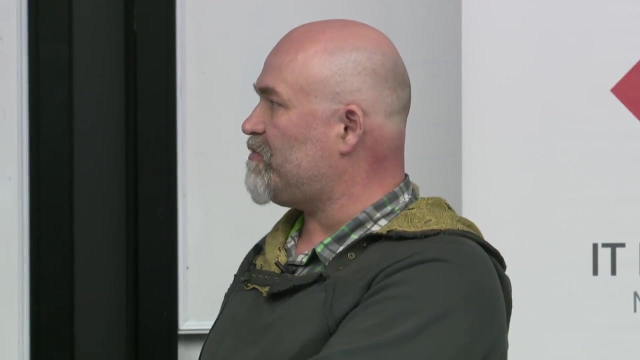 another 10 hours. Okay, 5 then. Right, I like the zoo. so the day I thought I could get a free entrance to the zoo doing computer vision, I said yes, let's go, let's take all the students. And that's what we did. we took our systems to the zoo and said we could maybe. 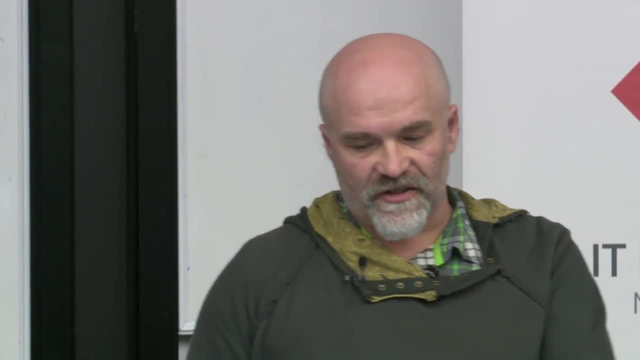 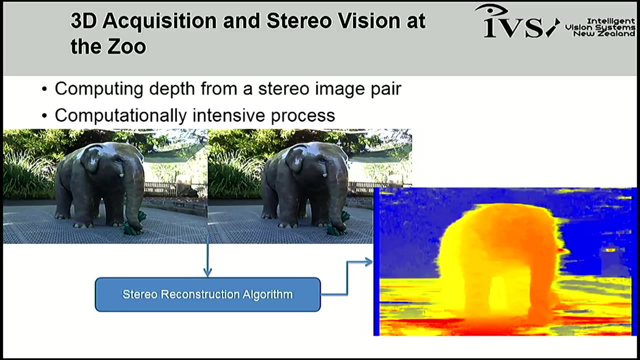 install some systems for you in some of the enclosure. So we brought our cameras a while ago and we started with the animals that don't cause us any trouble, that is, the ones that are not moving. that's a statue, So that was the easiest. 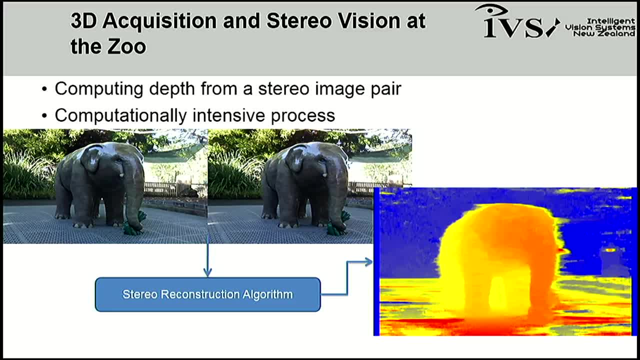 one. So we took two images and applied a bit of our stereo reconstruction systems and created what we call a disparity map, which is color coded: The closer the redder, the further away the bluer, alright. and disparity is inversely proportional to distance. We can do a small experiment with fingers later to 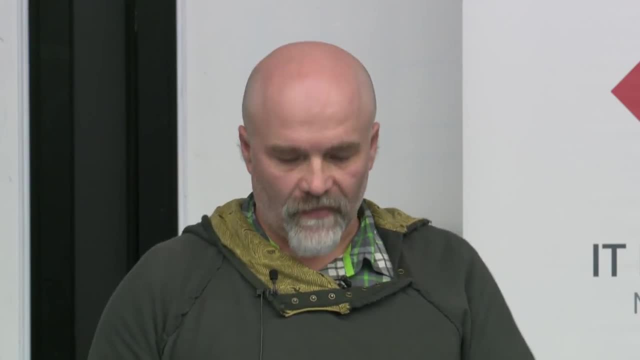 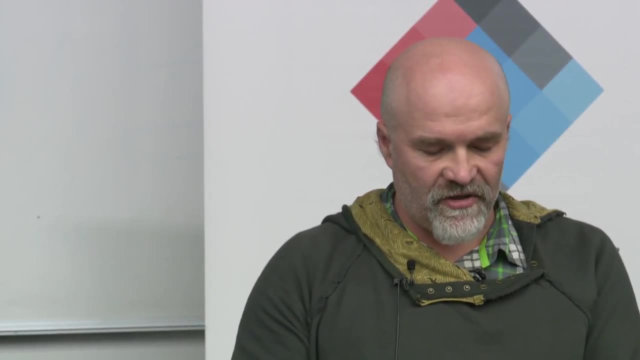 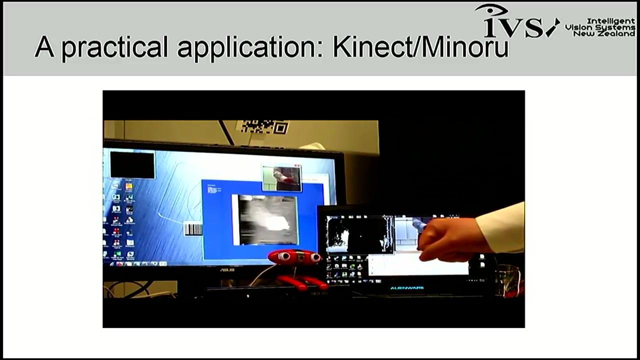 understand that. we'll see if we have time Now I would like to show you an application of that. I have quite a few videos, so I might try to show you a few of them. So that's weedwild back. Alcatel is very interested in equipping houses. 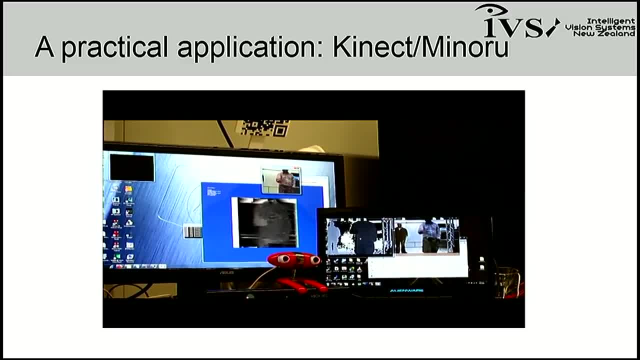 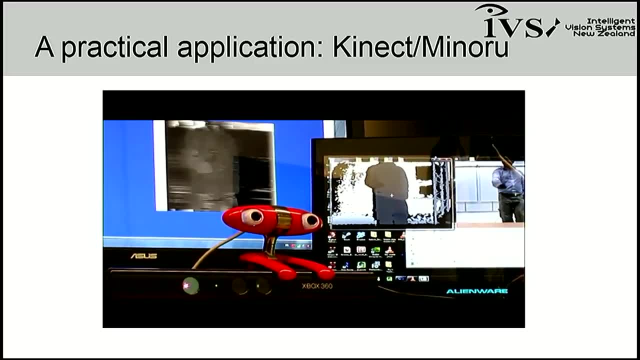 with systems that actually can monitor everything and create 3D objects on the goal and create the 3D environment. The systems by then don't have capabilities to see a few meters away and close by. So what we say, hold on, we use that nice. 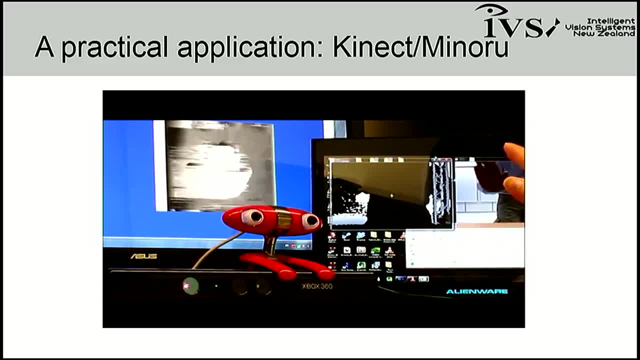 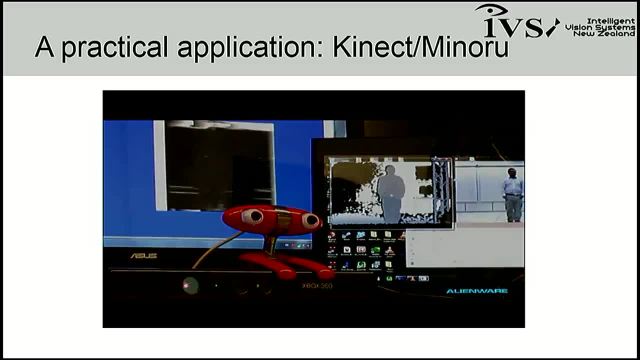 friendly red stereo camera that looks like a tiny robot that was called Minoru, and that camera just cuts out all the images I can see very well, very close, So let's use it. It's the image on the left. It's a display of 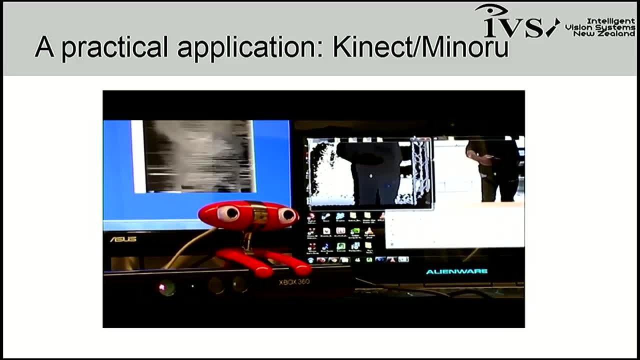 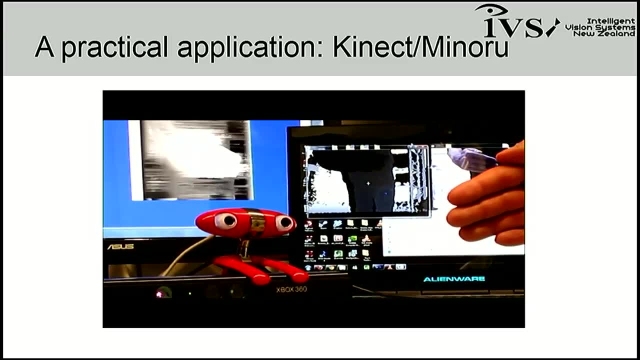 distances of objects. When it becomes all white, it means it's too close. Now the system below is a Kinect. It's an active infrared structure, lighting system, Project lights. look at the deformation. creates a 3D map out of it. 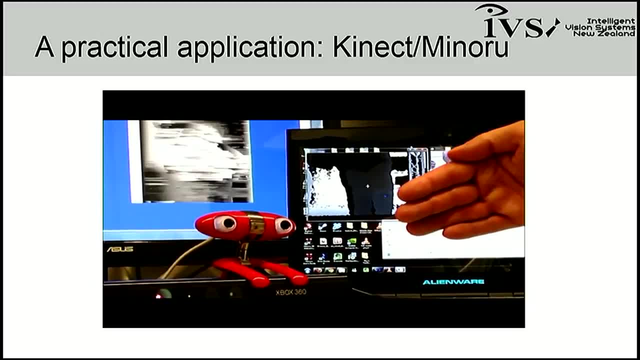 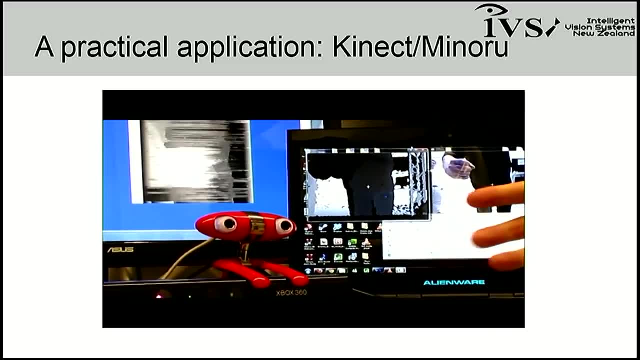 So, basically, the mineral would see very close by if you wanted to interact with the hands, and the Xbox would look at the environment. So we demonstrated to Alcatel that we could use both at the same time. All right, and that was working out of a laptop. 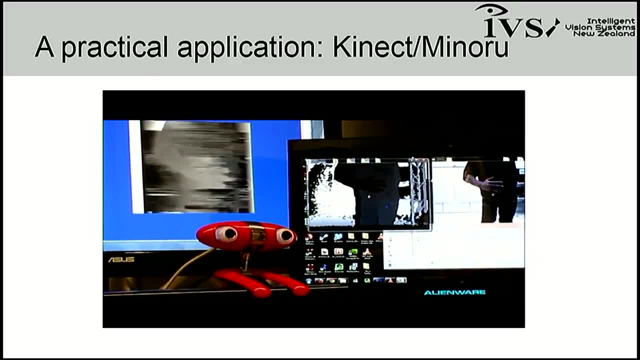 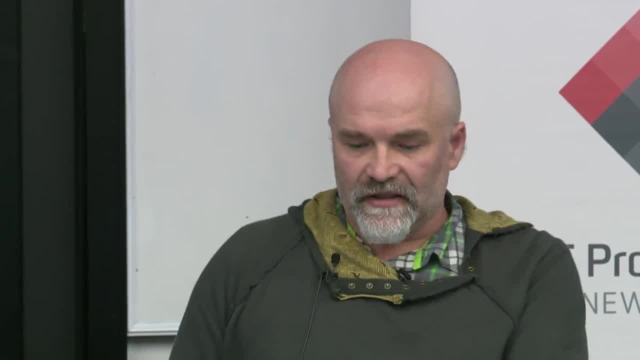 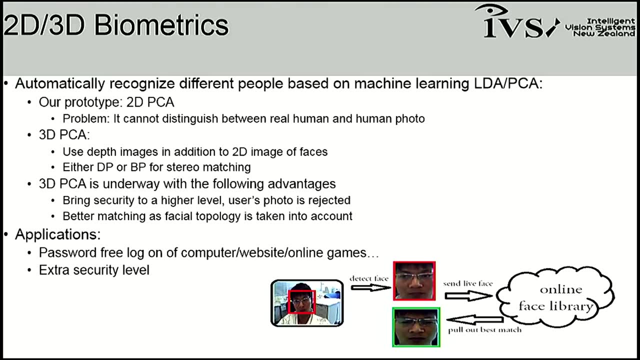 with a GPU a couple of years ago. So another application which I really like, and that's why I'm showing it today, it's face recognition. So I thought, okay, well, we have a system now We can control webcams from a remote computer, So we can attach two cameras. 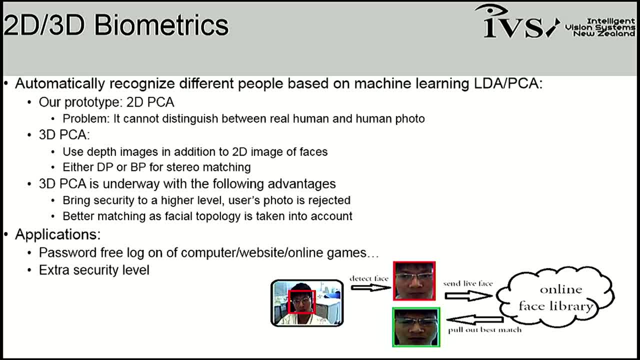 We can do a lot of calibration of the cameras to make sure we have the proper data to create 3D. And then let's make a remote face recognition system. Whenever you enter a website you could be face recognized and that would stop problems. So banks were interested, uni sources were interested. a lot of people were actually keen. 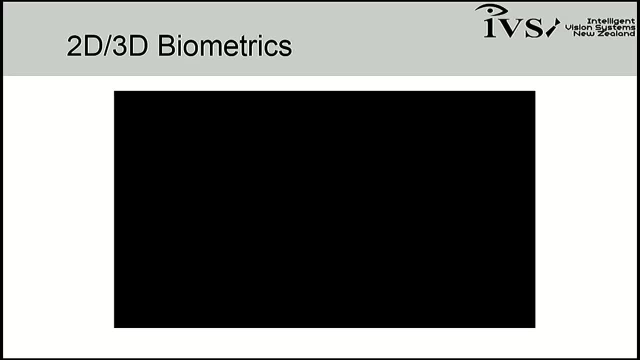 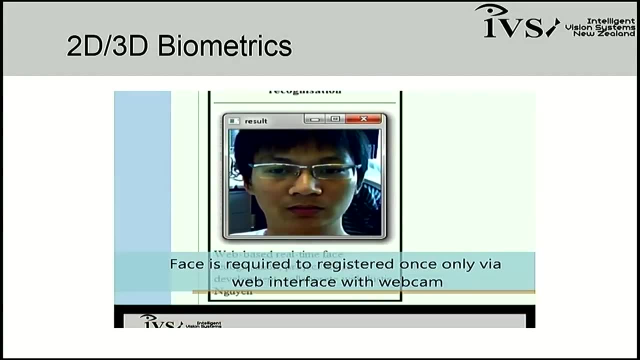 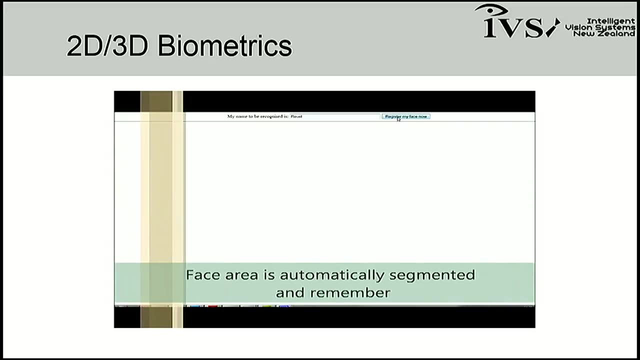 So you likely realize this is a few years before the phone starting to do that. The system was extremely simple. It's basically you enter a website and that's Min one of our ex-friendly lecturers And a set of faces will be acquired. 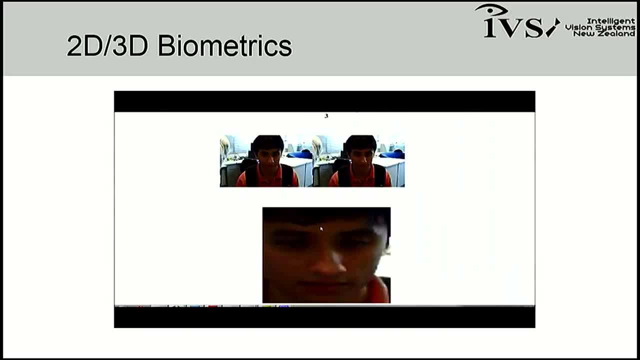 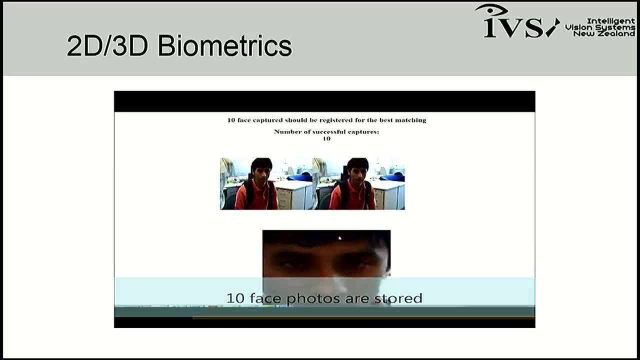 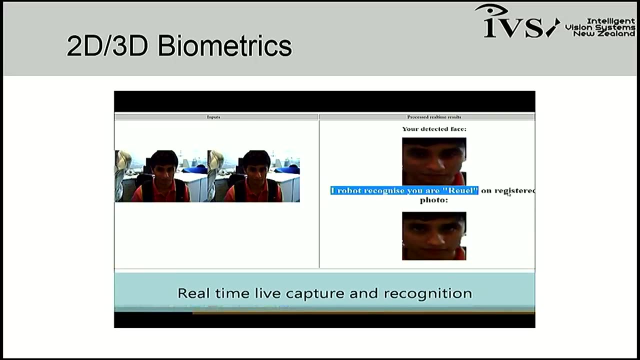 You just move around. it counts up to 10, recognizes your faces on the go, add to the database processes, extract meaningful information and then test it against that model anytime you try to enter. So that's a live detection. All right, you enter your name and here you go. So 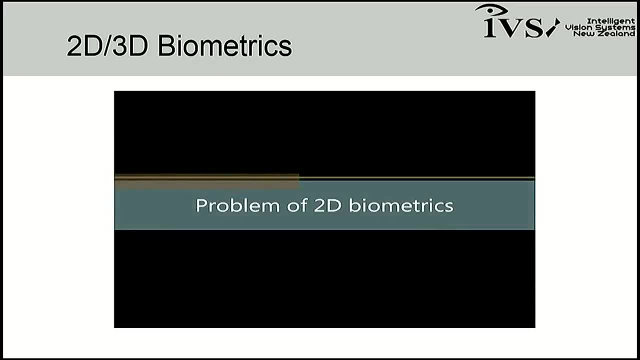 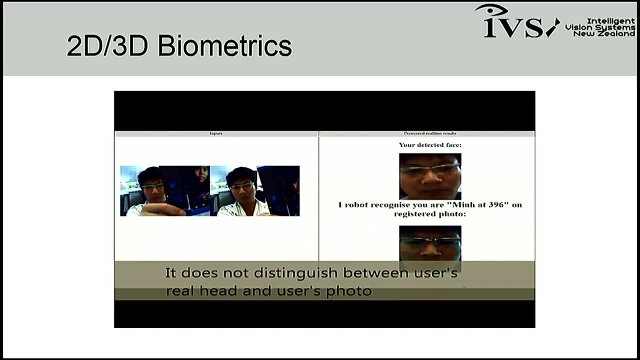 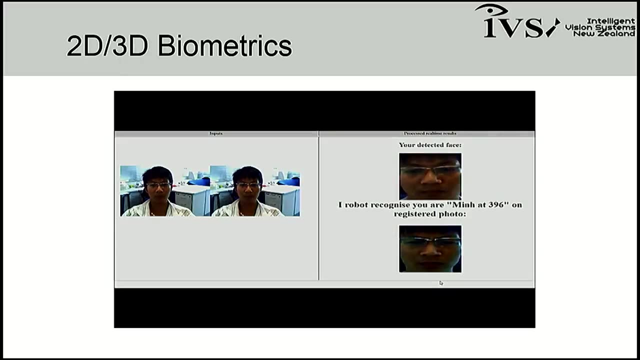 this is a friendly mannequin. It's always recognized. But an obvious problem with 2D face recognition is, if you have that yearbook from three years ago, that's the girl from the yearbook, so it's basically still recognized as a human. why it's still a 2D system. So what they have done since and 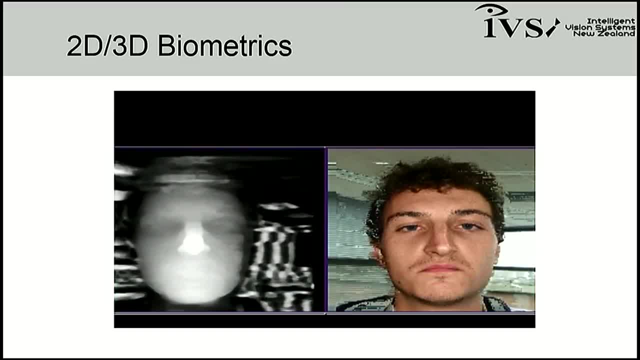 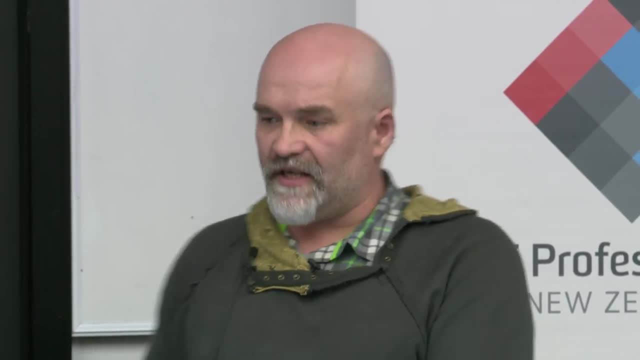 I hope that the current face recognition on the mobile phones use it. You use 3D information. You basically use the way your face varies in depth To embed a code. systems Right. So these are two applications of It's and it's. 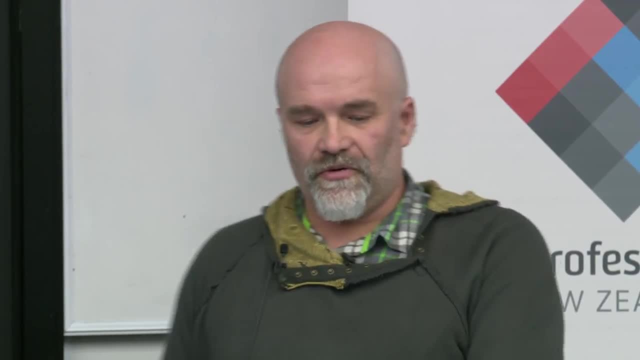 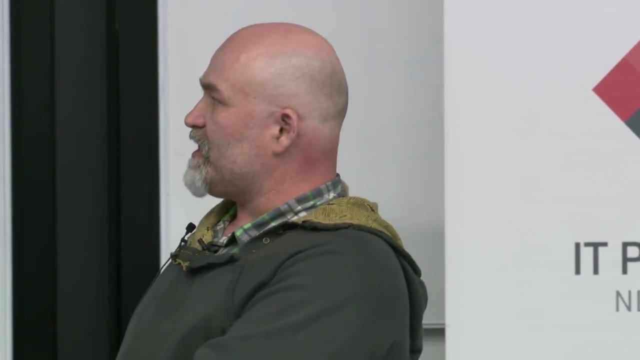 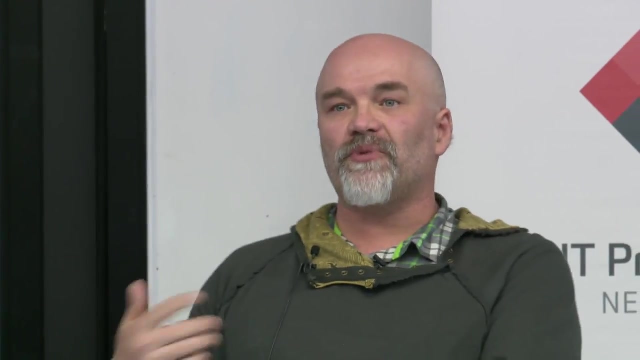 Okay, am I finished? All right, Let's look at the evolution of computer vision techniques, because what you saw is actually derived from techniques that were first invented in the 1990s, Struggled with the computers being limited and became into fashion. 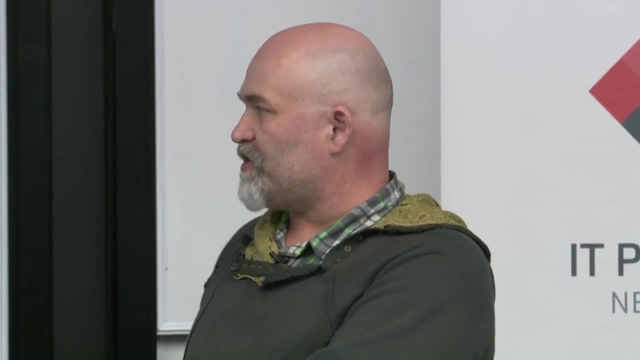 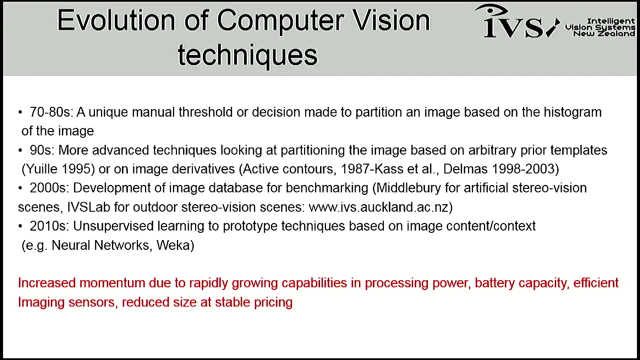 In the early 2000s in all Internet processors because of more and more powerful computers, And now it's on your mobile phone. It's as fast as the era is going In the 70s and 80s, where everything was cool and fun. you could use very simple techniques to describe images. 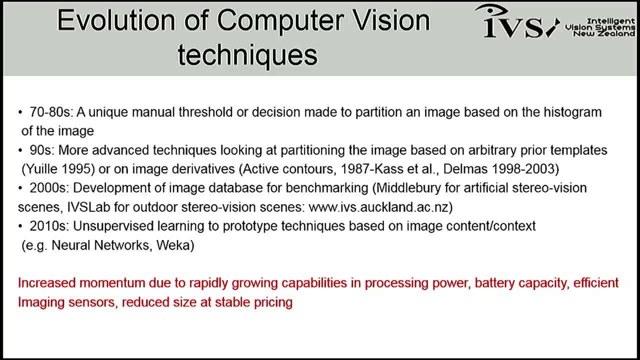 There was not many cameras. that was limited to labs, not many things happening. All was working fine. Then, the in the 1990s, you could have cards you could bring into a computer that were costing a lot of money But you could acquire data from the street. 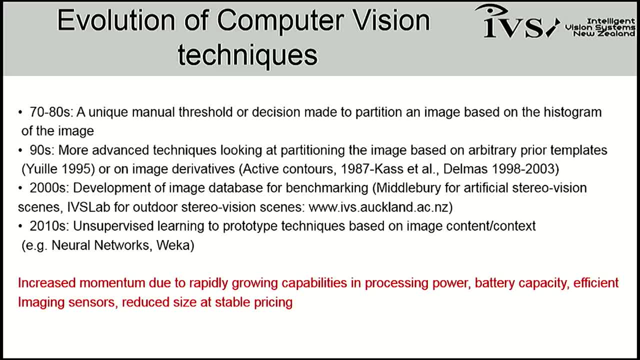 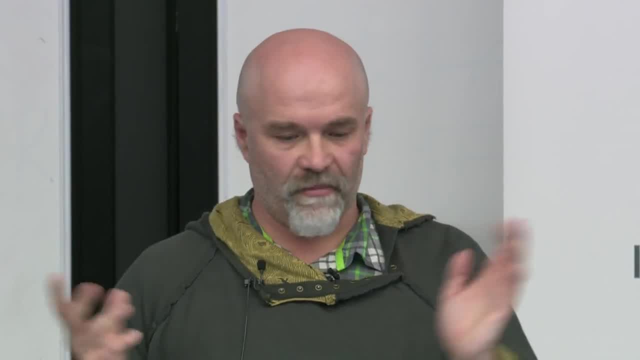 And basically look at processes. So to try to extract these triangles we discussed before, there would be these techniques that would be derived. I worked on that during my PhD. I don't work on these ones anymore. It means that they either didn't work well or I was really really bad, or both of them, Who knows? 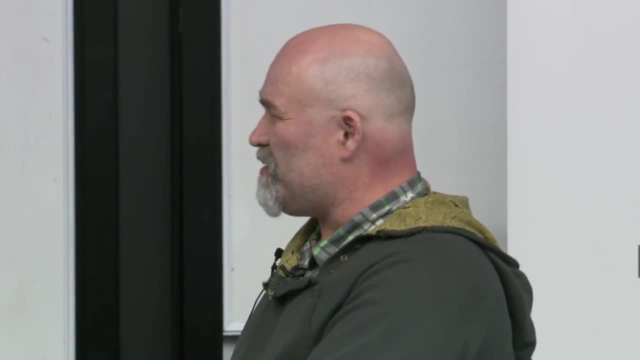 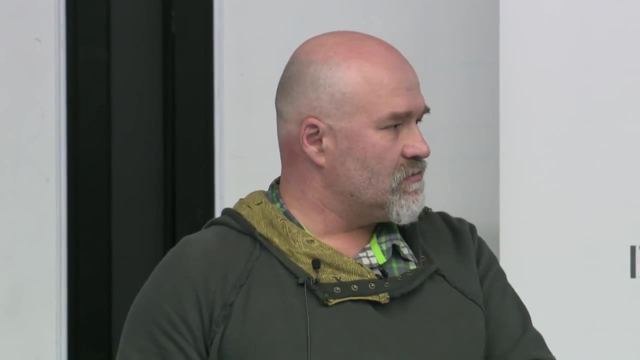 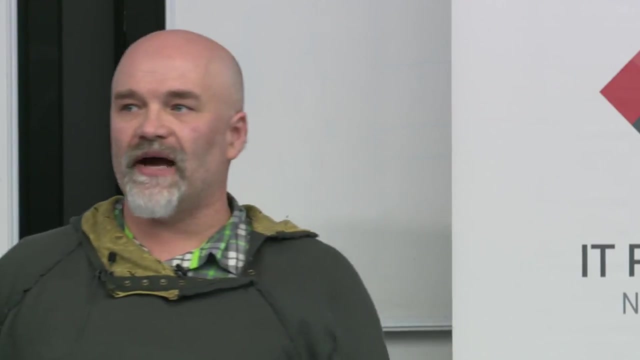 So basically, most of these techniques only work with images in control environment, which is medical imaging, Mostly with yogi, You would likely, maybe agree with me, Maybe. And what happened in the 2000s? cameras became more permanent, More and more cameras, more people able to share that stuff through the internet, So databases for benchmarking became permanent and 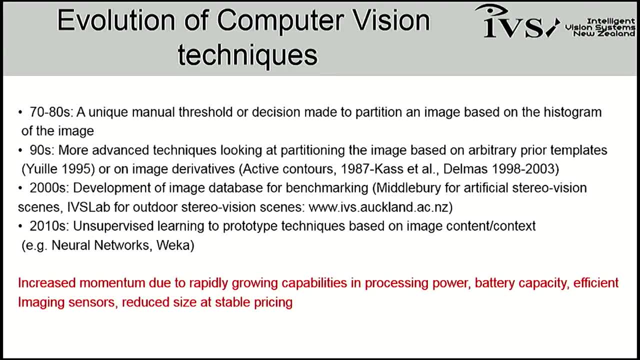 artificial stereo vision scenes and still powerful- A paper in 2001, Middlebury, who still used by a lot of people as the benchmark, And we have our own database of stereo vision scenes that we have acquired from a. And we have our own database of stereo vision scenes that we have acquired from a. 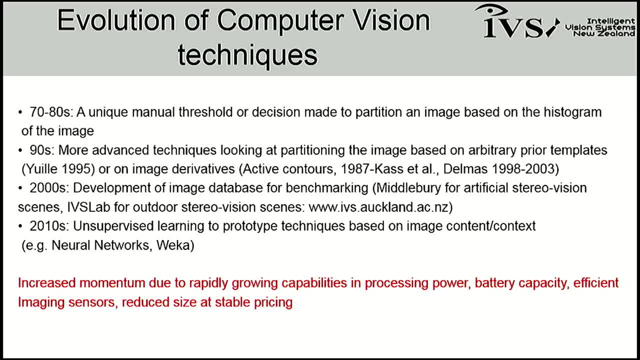 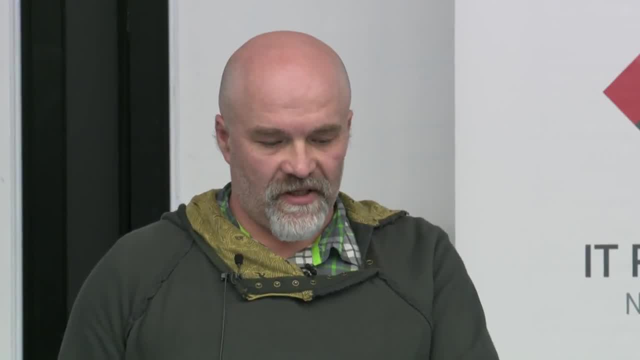 for the last 10 years, I think we have about almost 4,000 different scenes online and these days, everyone is so happy-go-lucky with neural networks they forgot everything else and say, oh, I don't know what to do. let's apply neural networks, it will solve everything, and then I can have a coffee, come back and 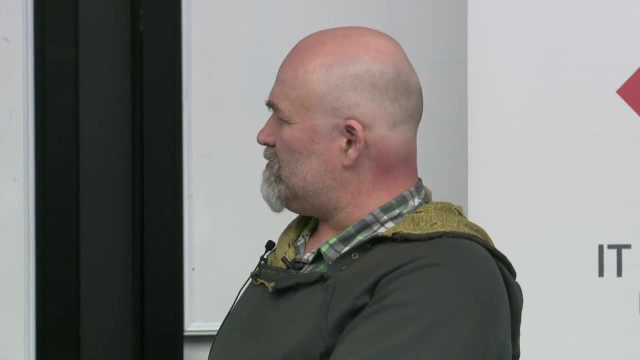 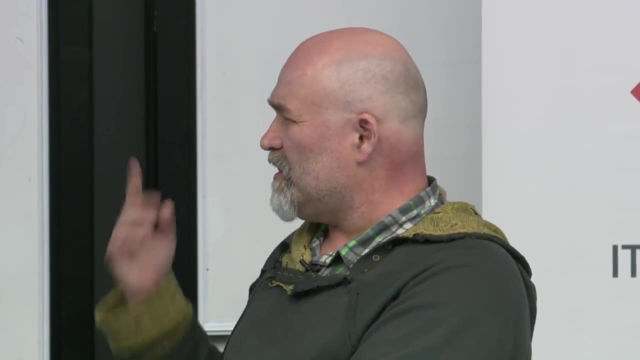 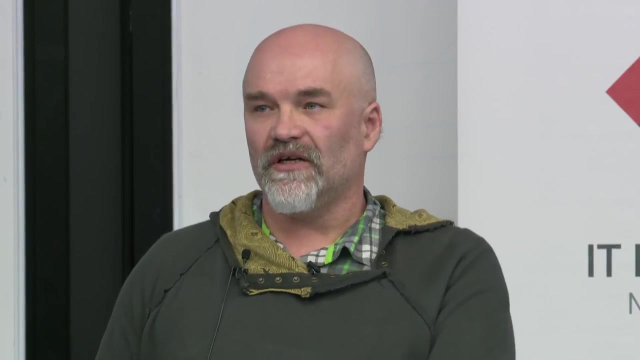 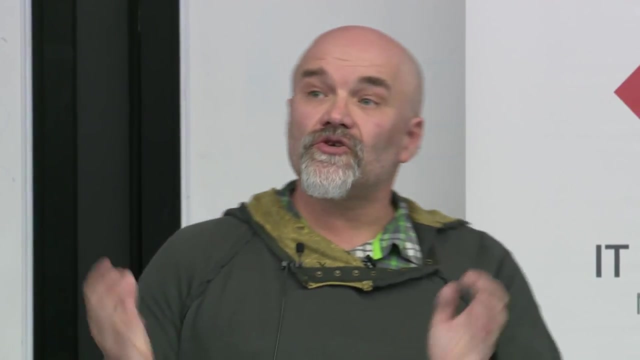 try again until it works. so the great change is really what I could see through time. is this increased momentum to fast-growing capabilities in processing power, but for applications outdoors, battery capacity. this is a game changing. it's lighter, more powerful imaging sensors. they're getting cheaper and lighter and smaller. this is why we can do what I'm about to present now. now. 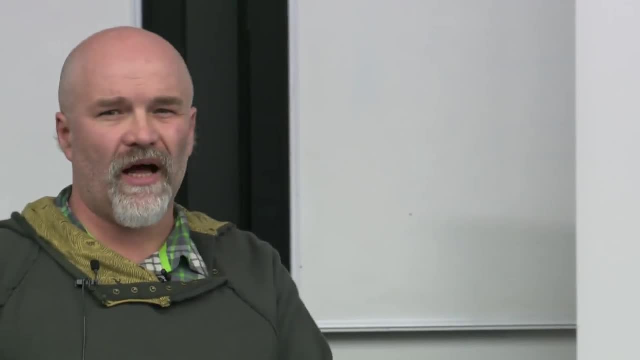 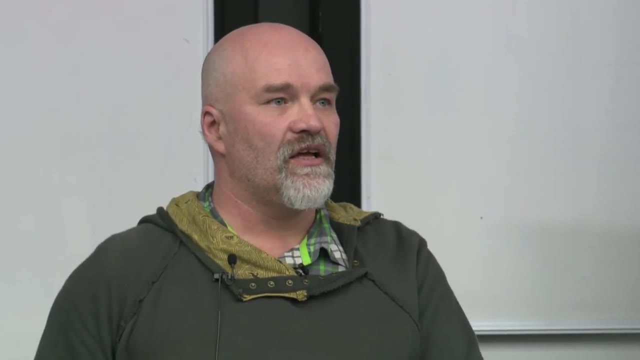 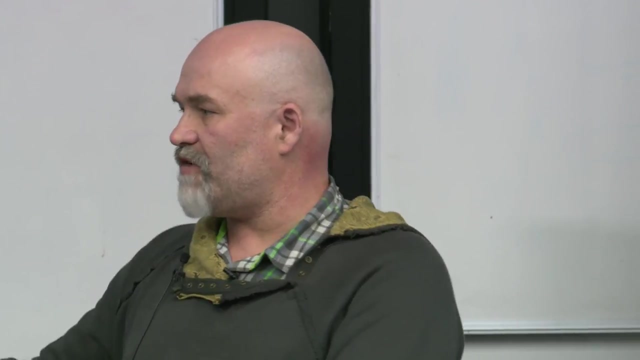 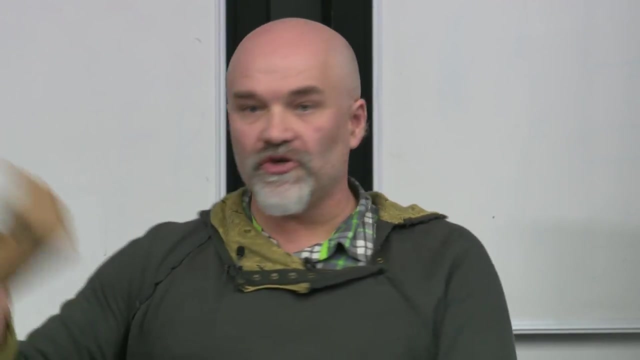 we may or may not do. the next one: who installed the mobile application in there? we have boxes here. if you want to try your VR, you should click on what it's called VR demo. alright, the mirror, Trevor. whoever wants one, please bring them back at the end. you don't just trash them away. so these are the Google Cardboard. 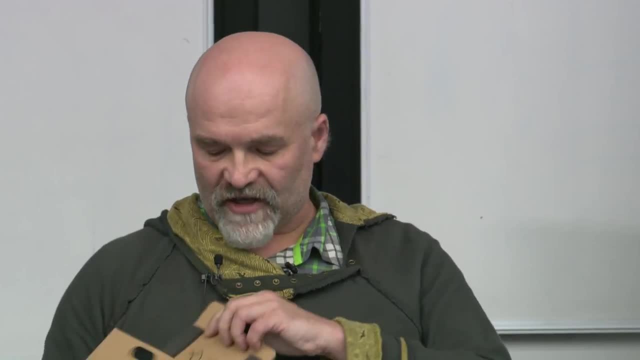 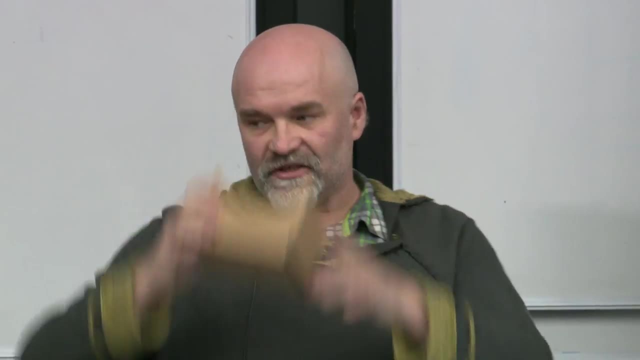 you can use your normal phone. you place your phone inside and you click on the right button before you put it in and look in there and the right direction, it's better and you will see a bit of VR. so, anyone- there's a few people here- yeah, you can. 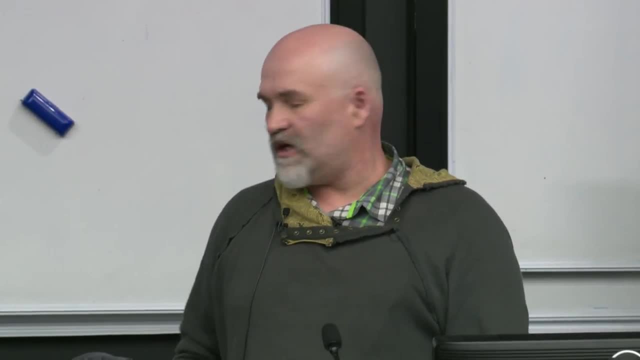 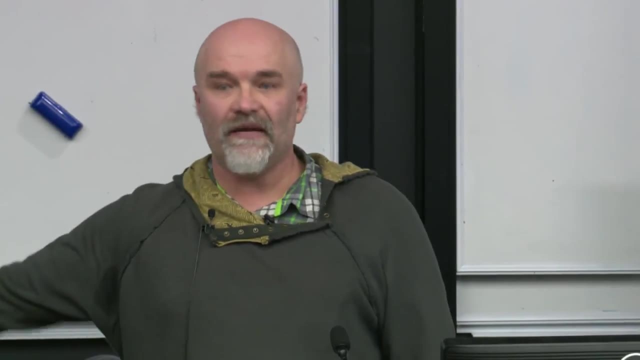 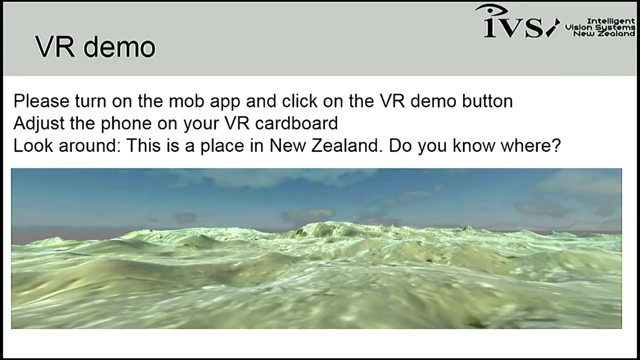 get in there and if you want to switch on that one, yeah, yeah, thank you. so you can pass that one on. there's the phone, alright. so we'll do a tiny game. which is where am I? so that's a game. so we are in New Zealand and 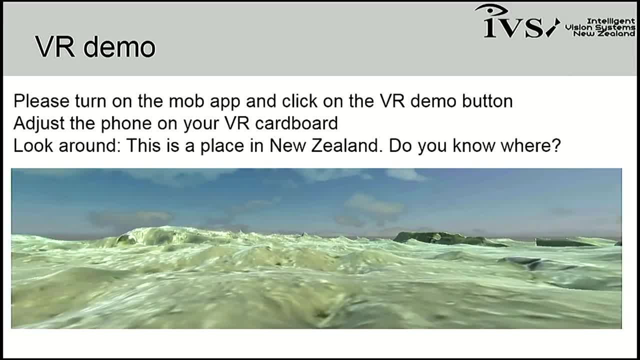 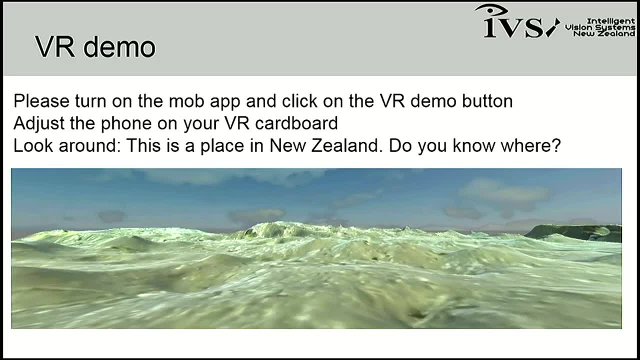 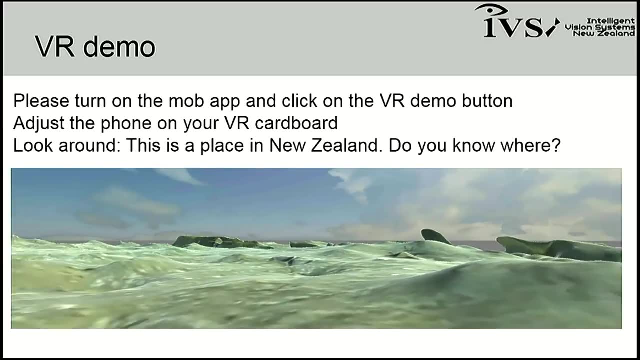 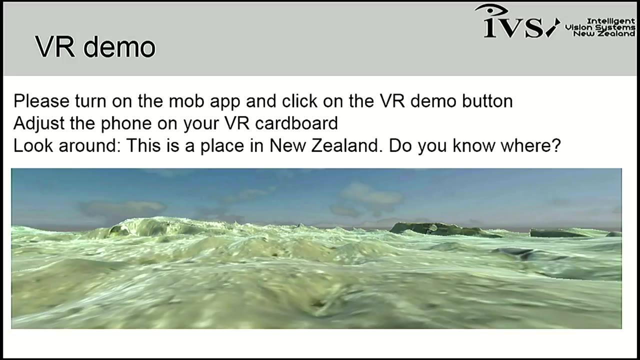 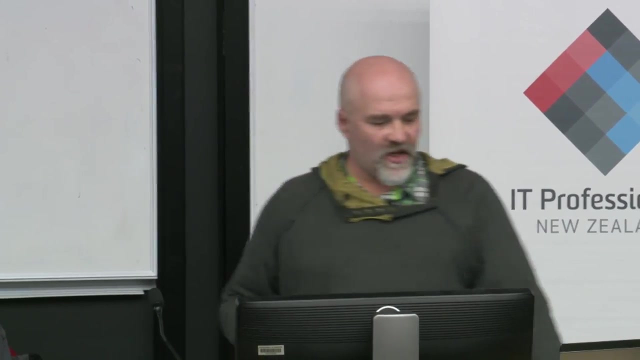 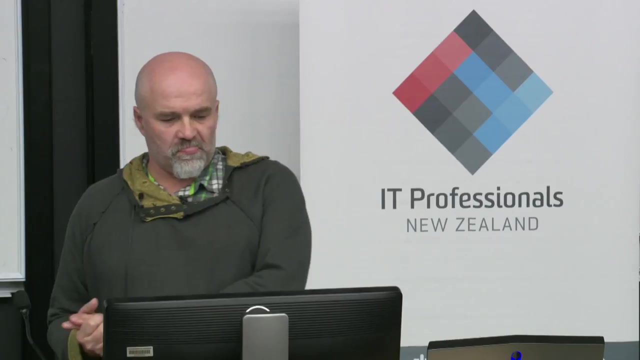 So we are in New Zealand and I can move it around. so it's a real place in New Zealand, right? anyone has got an idea that mountain South Island looks a bit like the South Island. no, who votes for South Island? yeah, North Island. it's not very clear, right? so there's a. 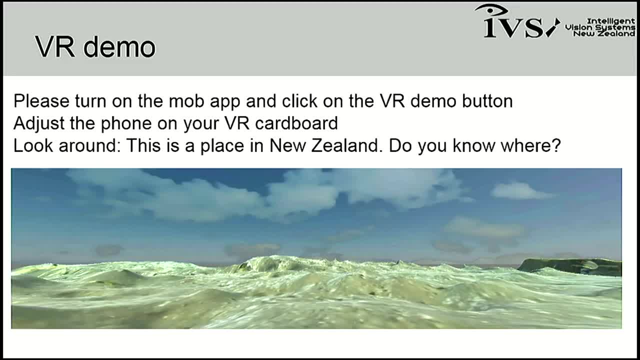 strange pipeline that seems to run around, and some of the video, if you look at it right. so while people are trying to get their VR working, and if people have the VR, you can look at other VR models. so you don't need to listen to me anymore, it's, it's a way to. 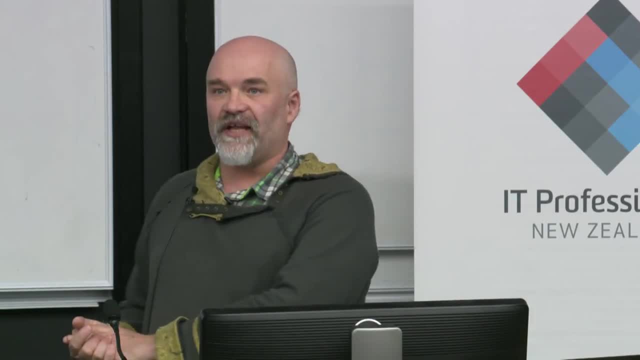 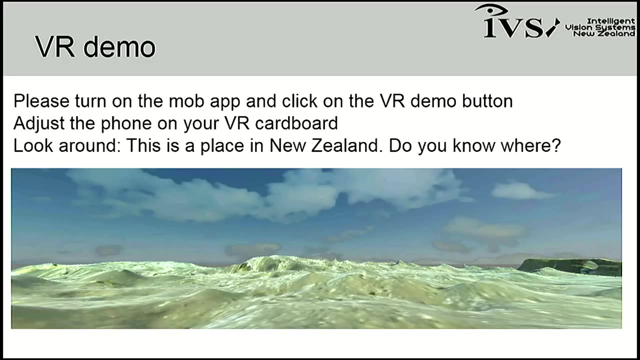 keep you interested. well, I'll tell you where that is. the tallest mountain there is about one centimeter, it's at a beach and it's basically worm burrows on in this jury, but it's data we acquire there. we managed to map the area in 3d and 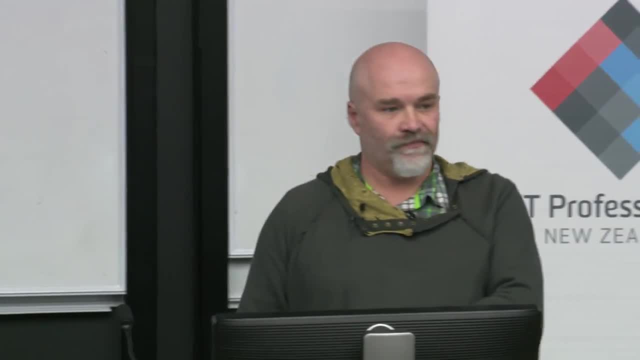 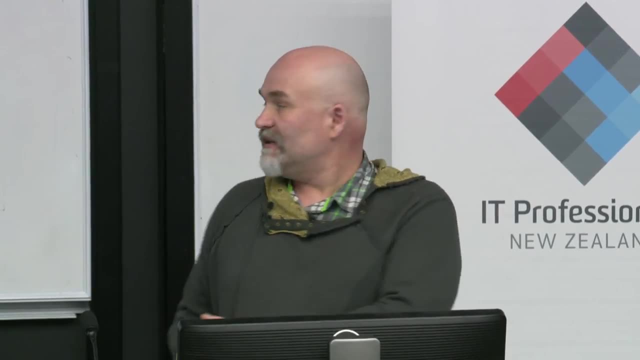 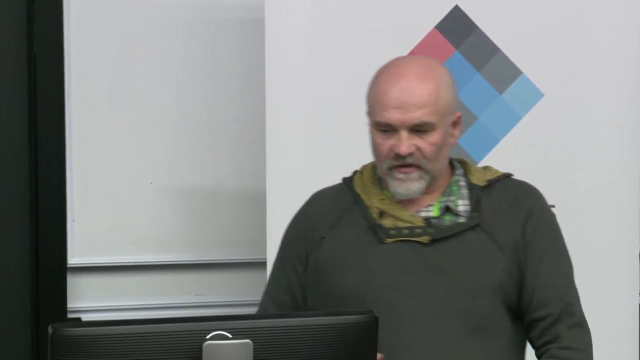 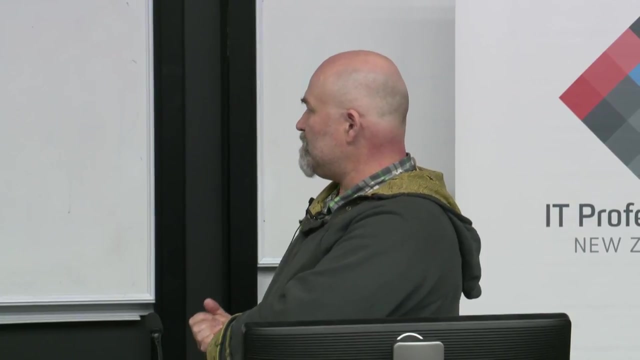 basically we reconstructing that for marine science, all right, so if you don't have your bearing right, you don't know anymore what you're looking at, really okay, so let's see how we did that, right. so this is not. I imagine we're not allowed to fly in Auckland- the problem. 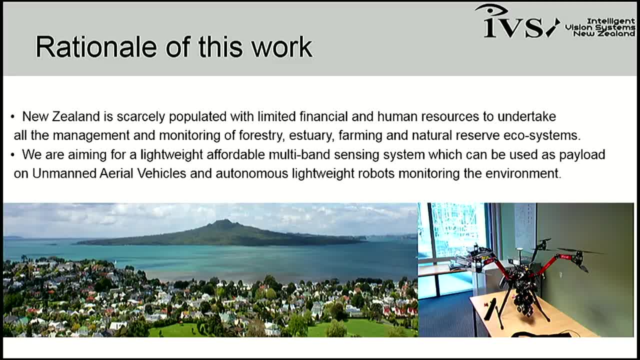 with New Zealanders is not enough people for that specific application. there's enough people for other things, but you don't have usually the resources to undertake all the management and monitoring of forestry history, function and natural reserve ecosystems at all times. and that's where robot vision 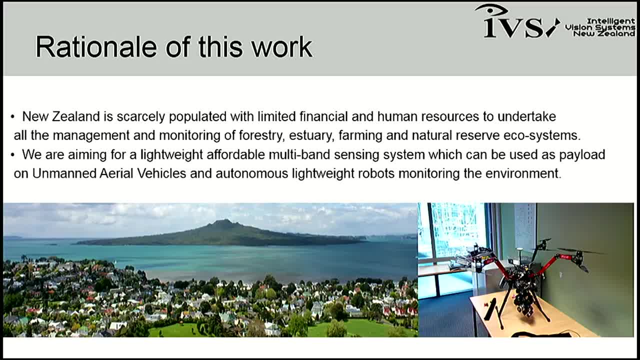 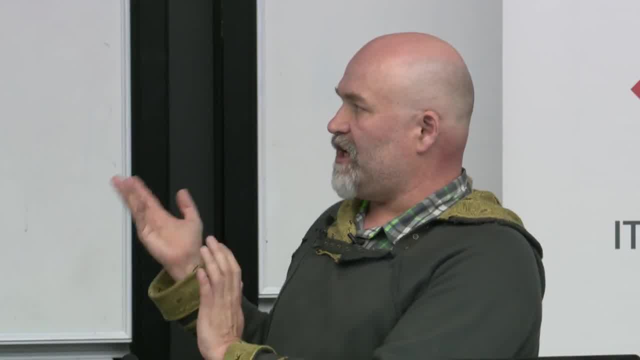 computer vision can be better than humans. A human has got only two legs, two eyes, two hands. We cannot be at two places at the same time. The same system, ported in many drones and rovers, can do that at the same times in many places in. 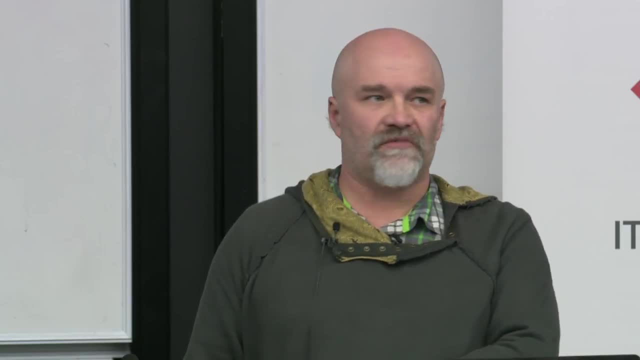 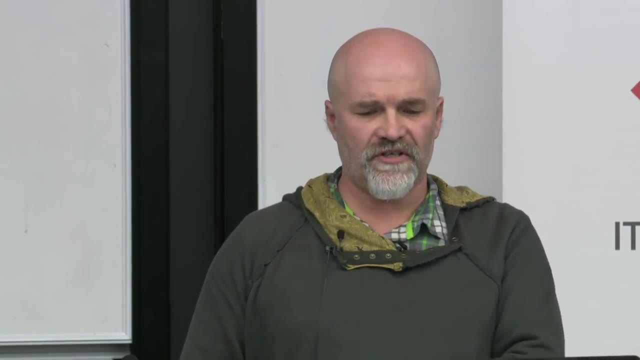 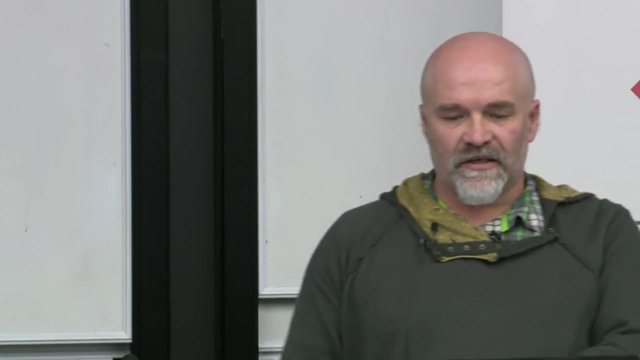 New Zealand. To educate a robot you need a couple of months from the programmer and a couple of days to get it ready. For a human it's 20,, 30 years. It's costly. So it's okay to lose robots, less okay to lose humans. With that in mind, we were 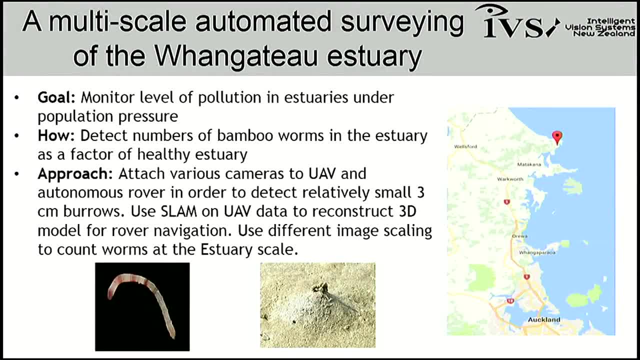 interested in going in what we would call a challenging environment. It's challenging. it's by the beach, away from the traffic. It's a bit windy but often sunny, and that's the Whangator Estuary, which is what you saw in that video before. And 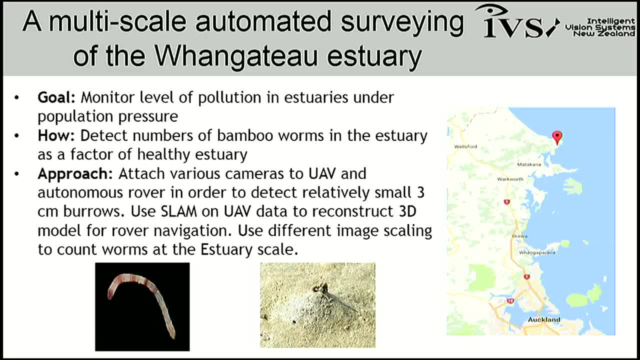 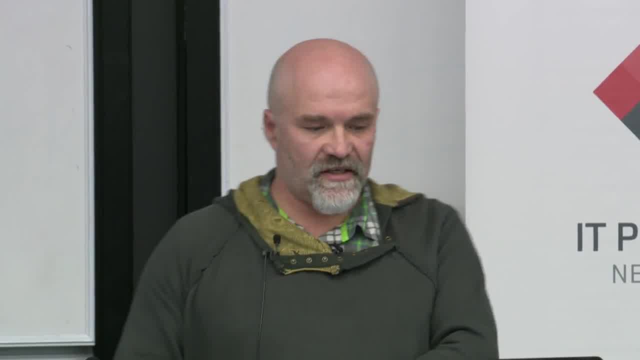 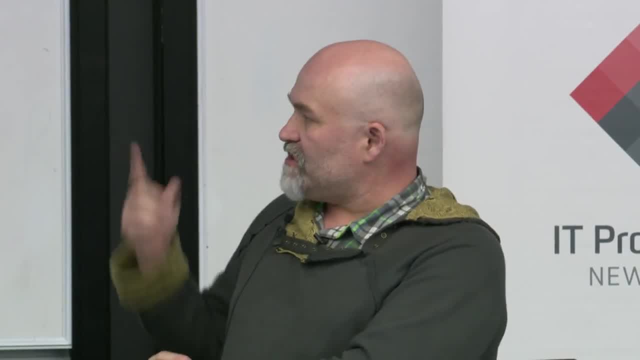 what happens there is that the people at Lee Marine Science Campus. they realized that the level of pollution in the estuaries is in their population pressure, especially there, And basically the number may increase or decrease based on the water quality And the bamboo worms that you can see on the left. they're actually quite important in 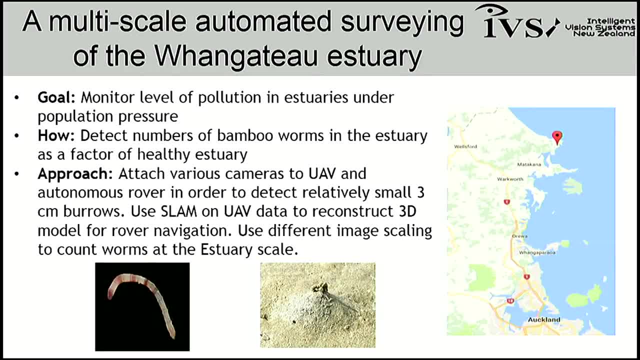 an healthy estuary. They will filter sediments to survive and they will eject sand. And you can recognize where they are and when they're active with that tiny mountain. I'll show you a couple of examples: the Great Lakes water, since there's some. 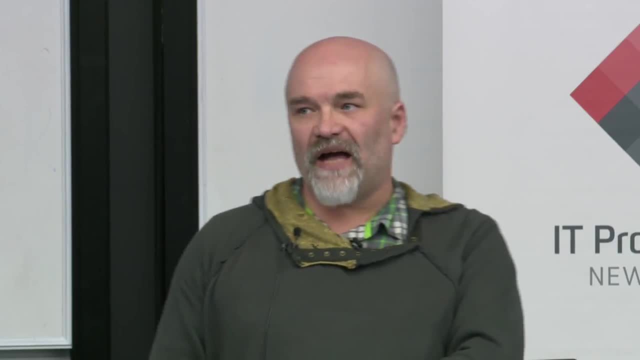 of itダー and the soldiers who are there now, but you can see that the water quality is not enough. So we decided to do a couple of rounds of what we call a drone-a, drone-a, drone-a-drone And, where you can see, there there's a couple of 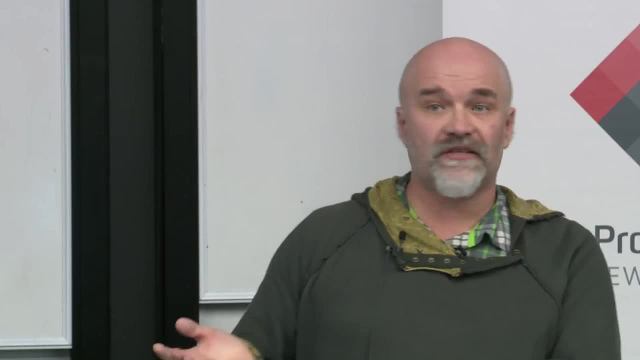 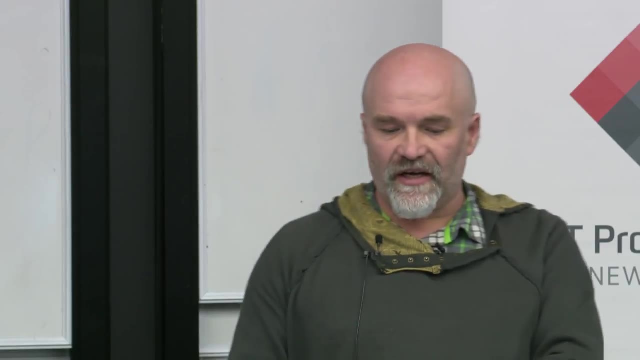 different, different SLPs that you can see here. So if you look at the right here, you need to be able to fly different conditions, different time and to be ready at all time. So what we decided is: we have the capabilities these days. 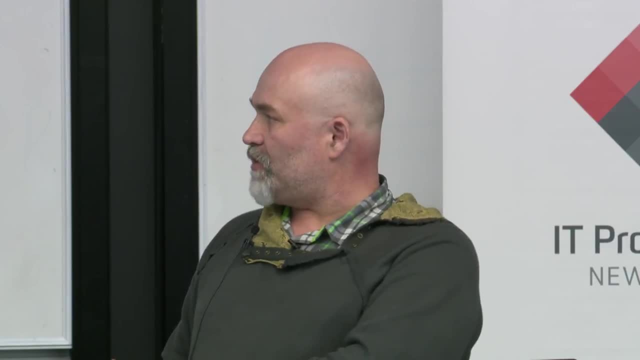 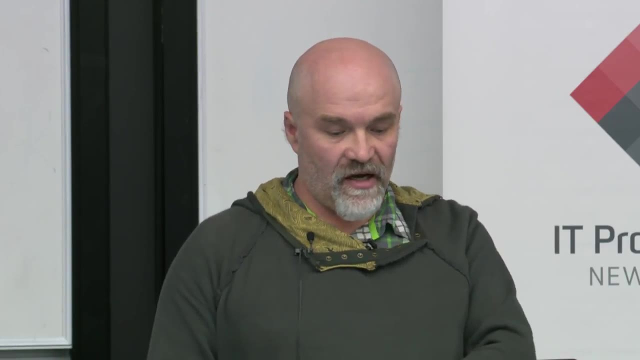 to fly these systems in order to detect these burrows. It uses a lot of manpower to set this up, so the whole team who's here- and I'll give you their names at the end- basically often going there. we'll be back there in two weeks. 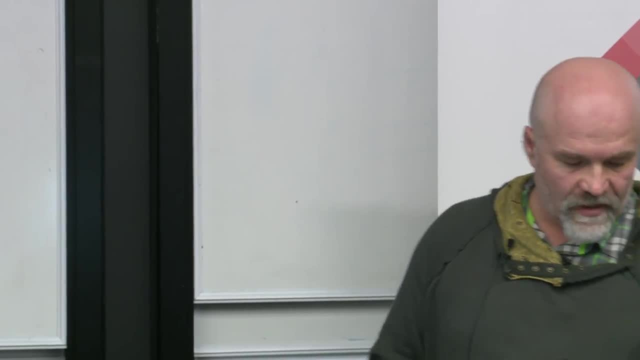 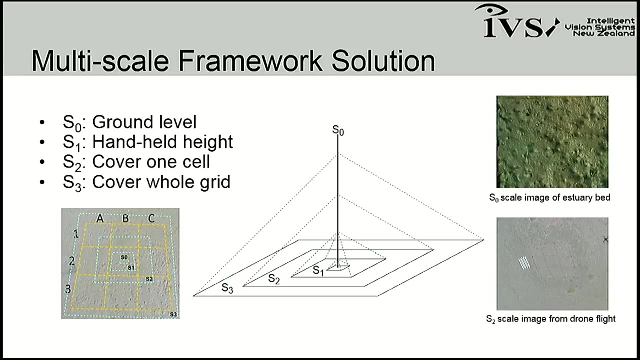 and we'll see how we try to solve the problem. We decided that we couldn't go in one scale. You cannot expect to fly at 100 meter altitude and see a burrow which is a centimeter deep. That doesn't work. You need to be very close by. 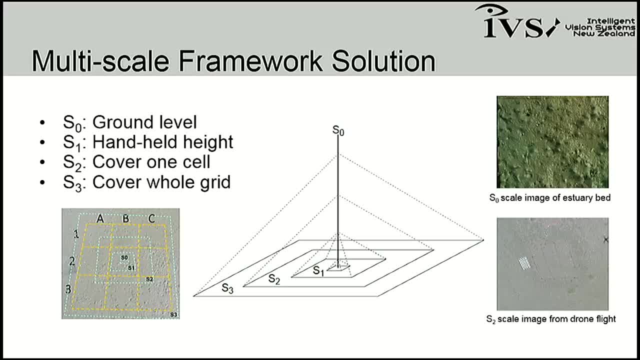 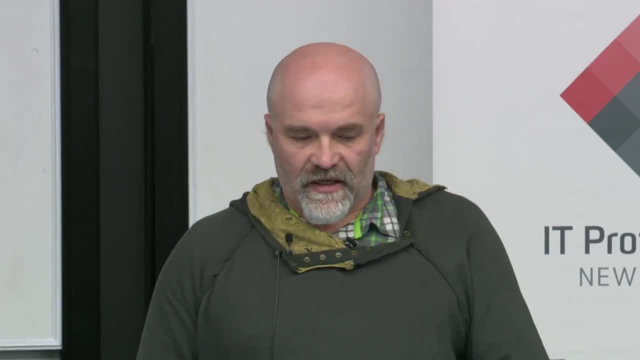 But we would like to scale the whole thing, the scale of the estuary. so we decided on the multi-scale scale framework, with different systems, mapping a different scale and bringing everything all together. so a fair amount of capabilities all together. Now, what we said as well is that we can create. 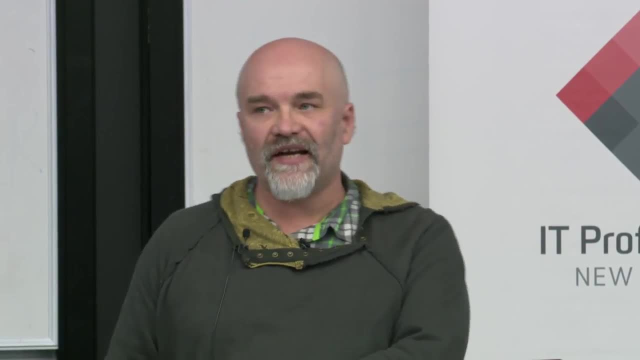 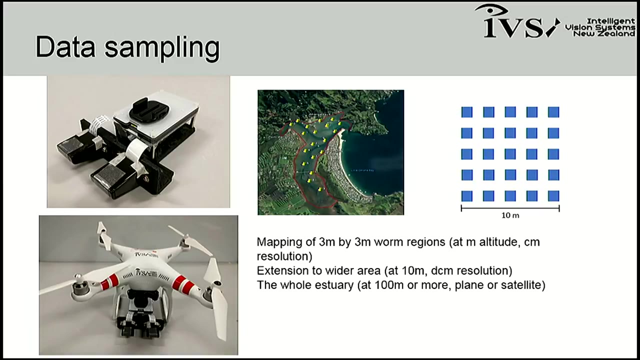 these days our vision systems that is light and capable to fly for hours. The image on the top there has been created by James Cooper, one of the PhD students here, and some 3D printed parts, and basically puts two cameras together. 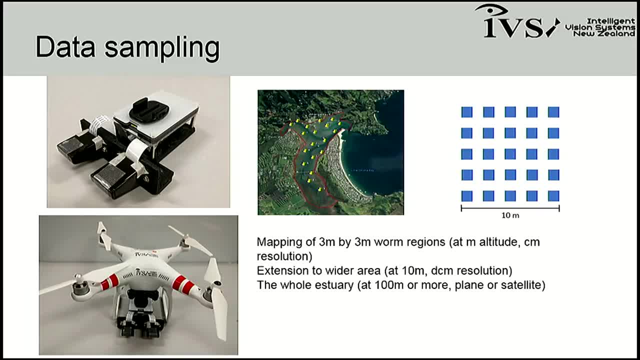 There's a mobile cell in there and there's a Raspberry Pi which is capable to emulate more or less the same power of your phone- power of your phone- and we attach that to your drone. so what I like to do with whatever I buy, I destroy them and I put them back together. Sometimes it works. 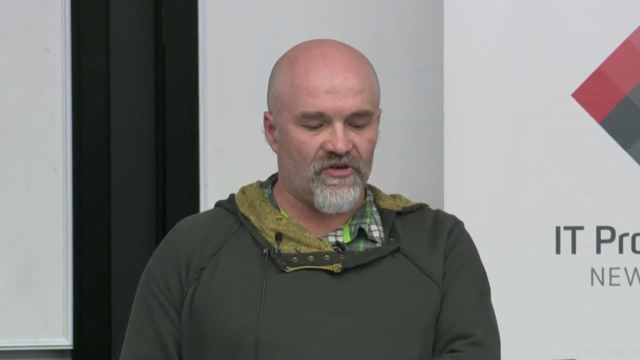 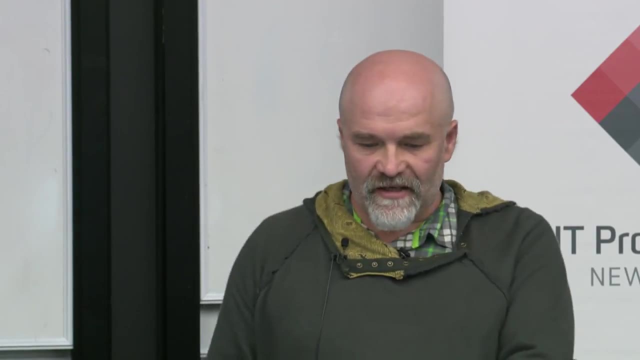 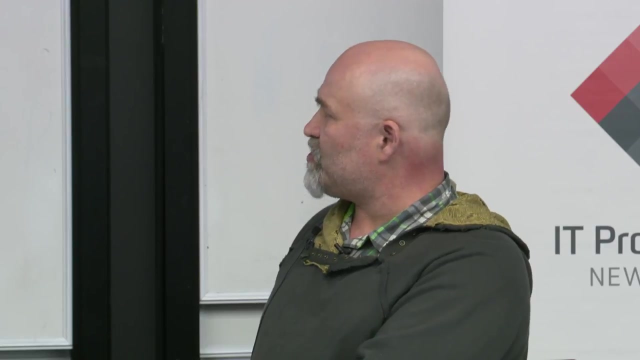 sometimes it doesn't work so I buy more. but we did that with these drones. they we took the cameras, they provide us away and install our own systems and, of course, the image on the right has been provided by our science. and I said that's our sampling points: the yellow ones, the estuary is in red and we would. 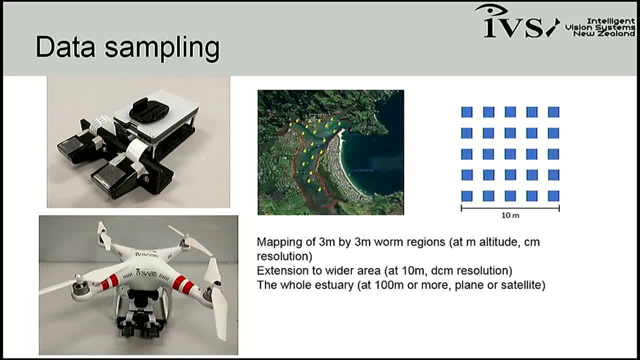 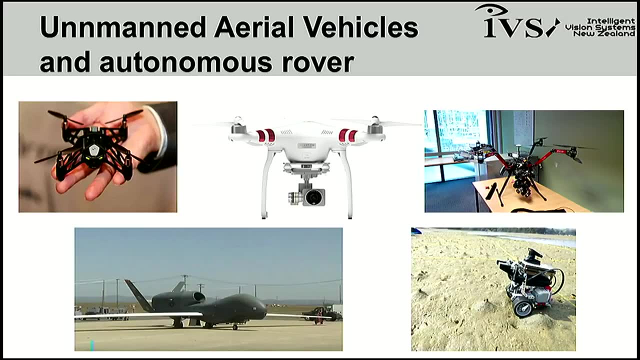 like to map areas of three meters by three meters at a meter altitude for a centimeter resolution. that's why we decided would work and we want to extend up to the whole estuary, all right. so flying at different altitudes, that's the scaling. So we went there and we had a few equipments. so basically, these are. 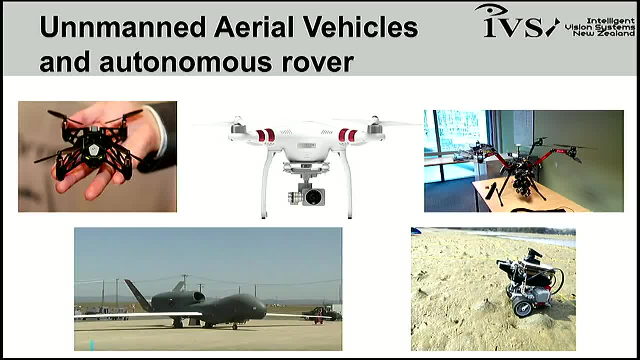 all our equipment except the bottom left one. there's- Robert never wanted to get me one, it's called a Predator. it's four million dollars with the pilot. I really try. Robert said no, has some advantages. also carries a bomb to destroy these difficult situations where you have, you know, like a possum, for example, placed. 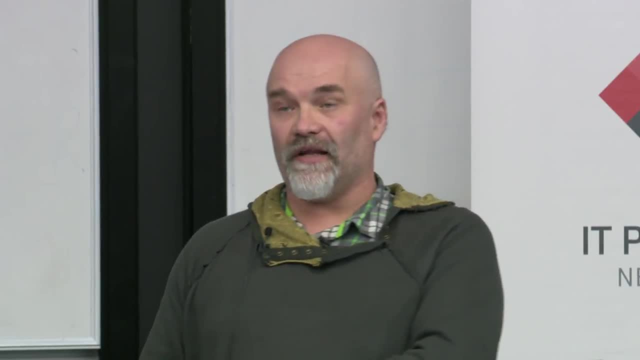 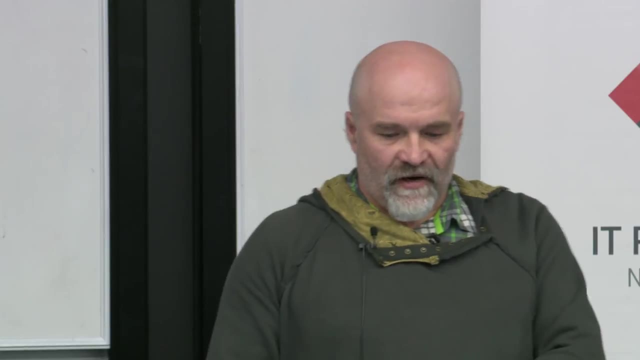 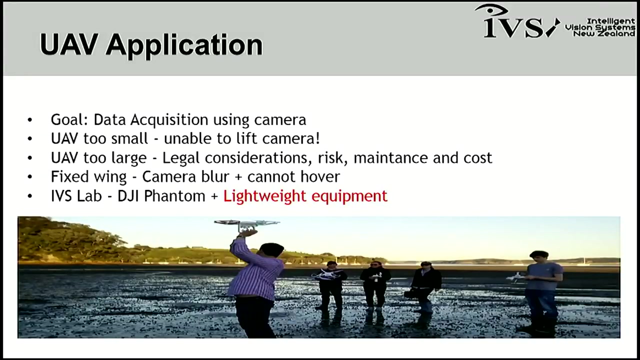 strategically somewhere. No, we couldn't get it, so too bad, we did with what we had Right. so that's us trying to fly these machines. as you can see, the take off technique is very, very advanced. They need one individual in charge of health and safety to take that turn. 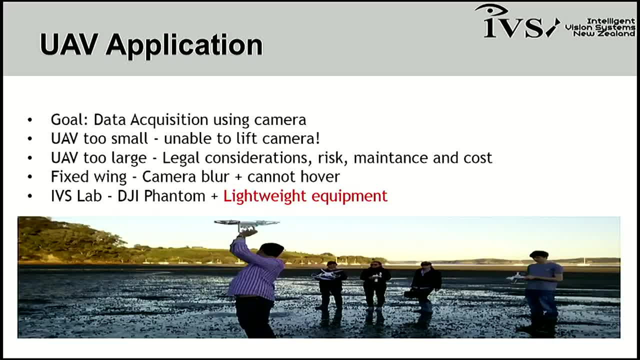 basically our goal is: we want to use cameras, we want to fly these cameras, we want to have these cameras on the rover. If the weapons are too small, it won't leave the cameras. The setup we use is about half a kilo and if it's windy with 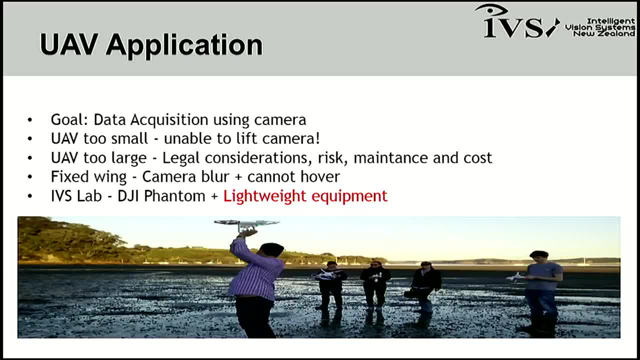 difficult conditions which we have experienced there. it's going to be difficult If the UAV is too large and we experience that- then you need different licenses to fly it. fly you have risks because when you put your hands where you shouldn't there is a consequence. there the cost of maintenance is pretty high and the drone 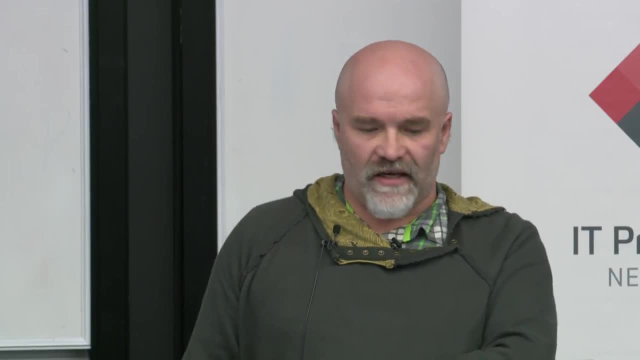 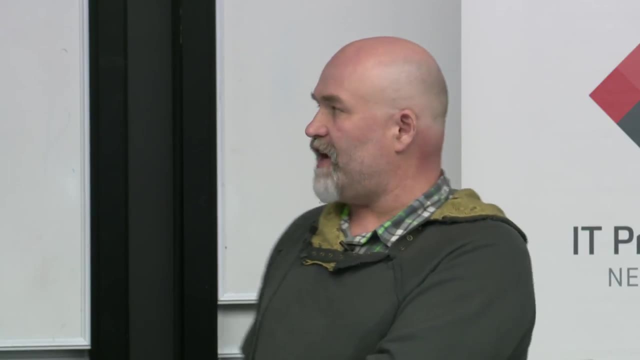 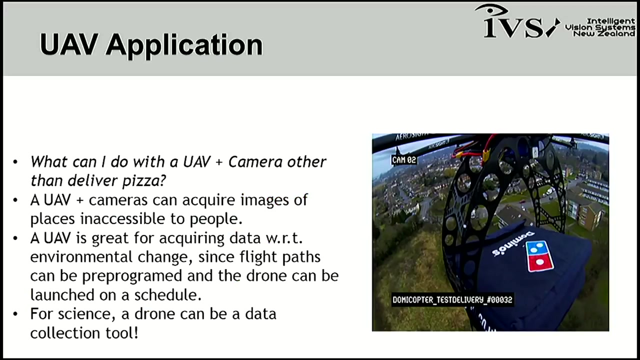 cost a lot of money, fixed wing. we considered that as too fast, so they will become our blur- cannot over above the areas where you entrust it, so we use some of TGI phantom- that was the two one by then- and super lightweight in-house created equipment. now, this is not a drone and we don't do dominoes, but you. 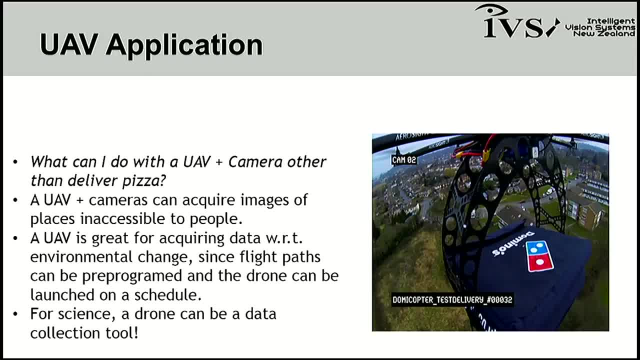 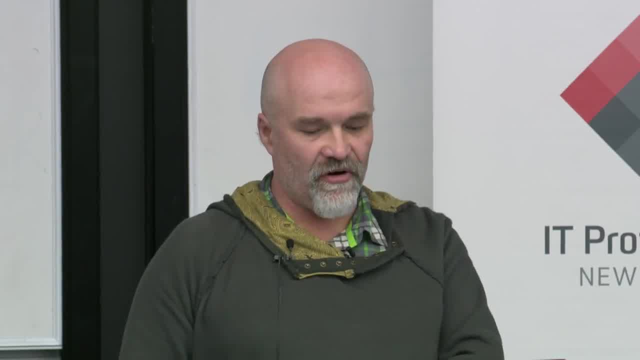 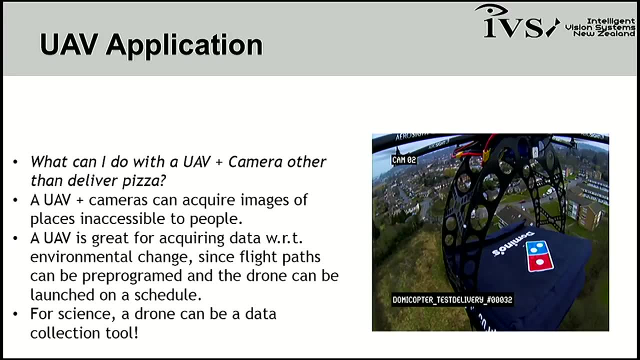 could just do that, and that's what they claim. they can do the three minutes you sure. okay, before questions: all right, that's going to be tough, right, and we'll try to go faster. okay, so we won't join. so we can go somewhere. we cannot go. 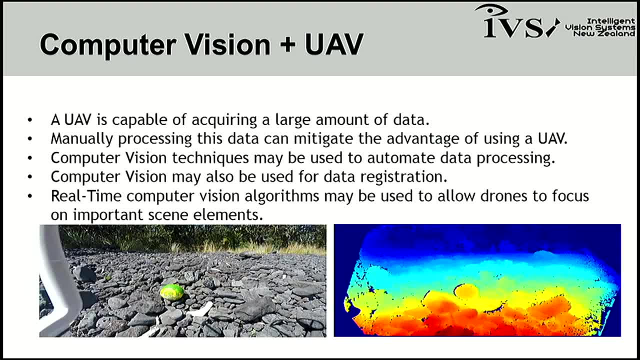 anywhere else, and definitely not for pizza. our first test is: we went to a rengi total and basically we're able to map different areas and what you can see if you look on the right image, which is a disparity image that gives you distances from the drone, the ball is also. 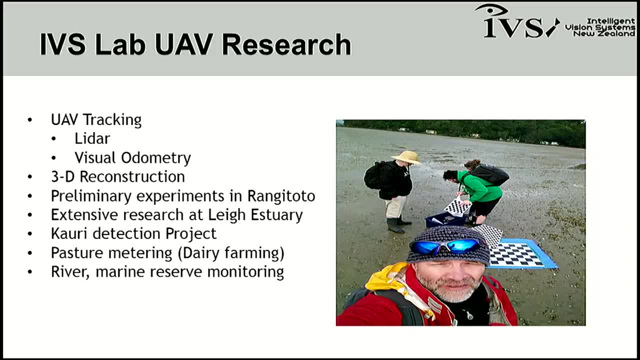 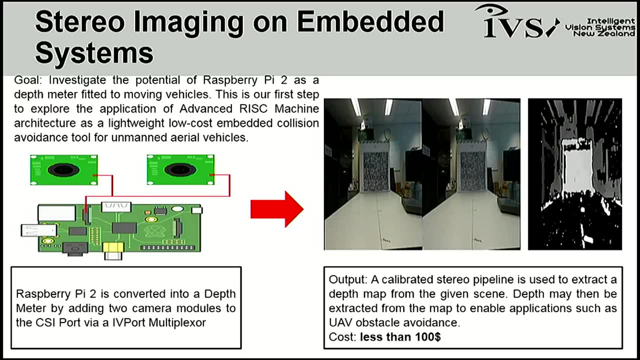 recognizable in that. so we ran some tests and started working on different projects without drones and cameras, and especially at Lee. I'd like to show you interesting things. it might take more than five minutes, all right. so this is the systems we created. we tested them indoor: two small 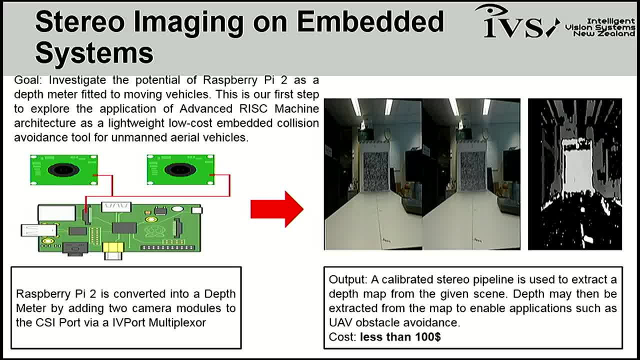 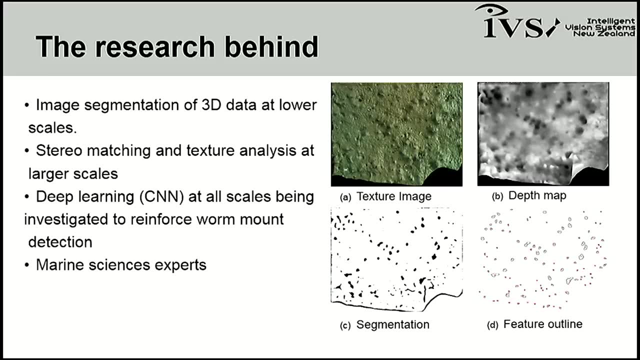 cameras, a Raspberry Pi. actually, we are on level three now a Raspberry Pi. we can acquire simultaneous video streams and it costs less than $100, which means if we break one, we get another one. all right, the research behind different levels of processing at the image level, at the texture level, at the disparity. 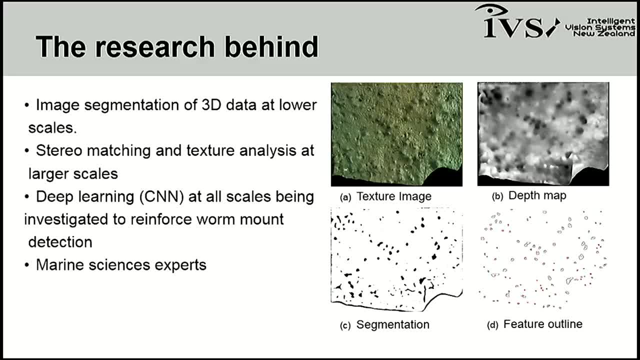 level and when we cannot solve a problem at the image level and the texture level, at the disparity level, and when we cannot solve a problem. when we cannot solve a problem, we say, oh well, maybe deep learning will help a bit. so it worked in some ways. we got a bit. 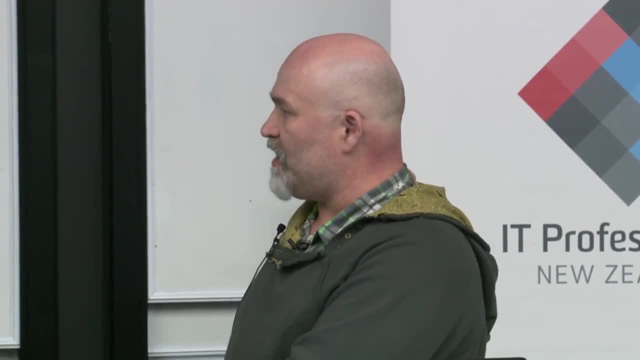 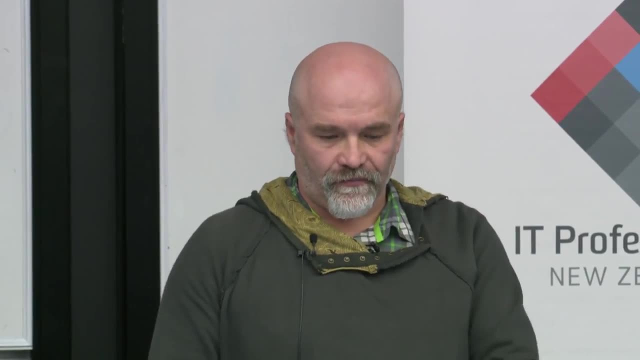 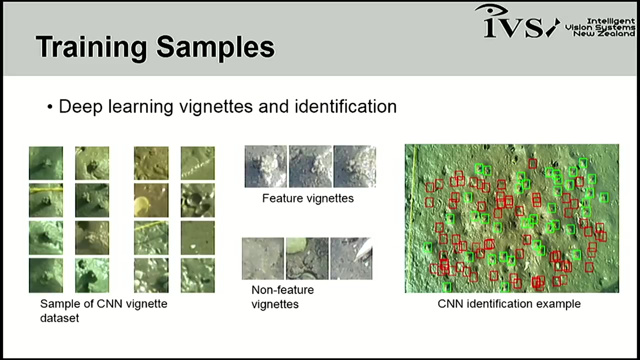 better outputs. we also have the chance to have marine science experts that will tell us what is the gold standard, where is the ground truth? what is a worm, what is not a worm? how do we deal with that a workflow? i think we don't need to detail that. this is some of our conventional 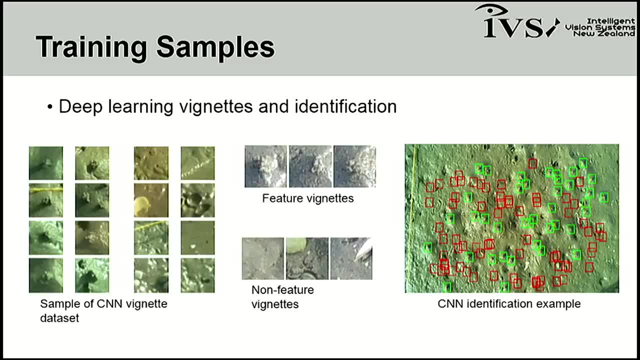 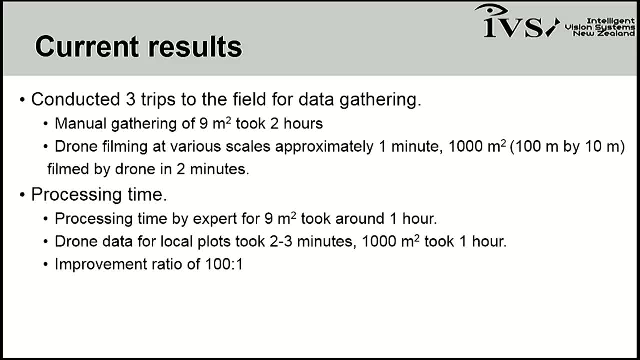 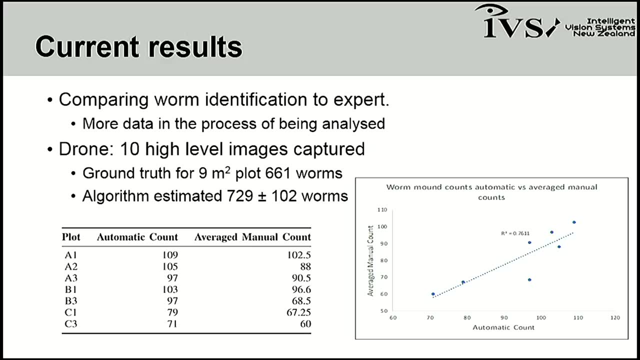 neural networks, data sets what is worms and what is not worms and identification in different colors. what's important is, i would like to show you some of our trends over several of our trips. we have a correlation of about 76 to 81. i remember. it's just correlation. 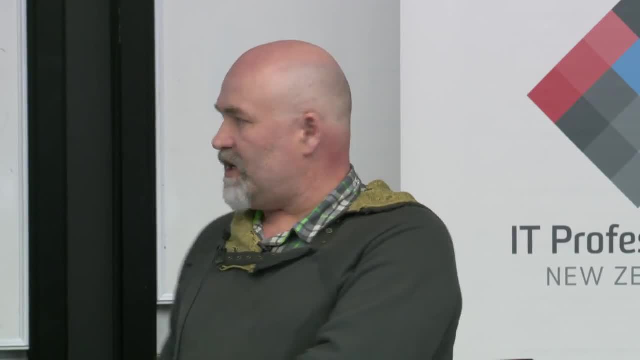 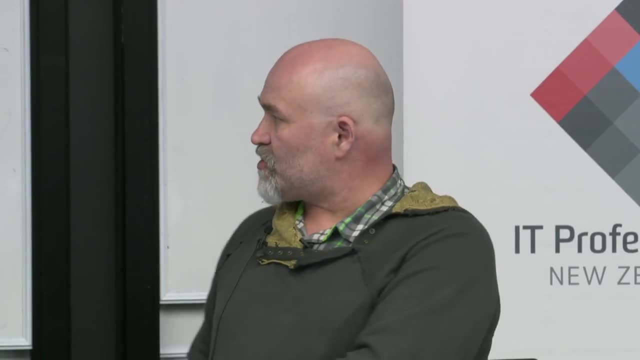 there's no. that's the problem with deep learning is, yes, you can say these data is correlated, looks like a worm mount. that's as much as you can say. and the there's no scientific um demonstration of this output. now, this is my take with neural network. 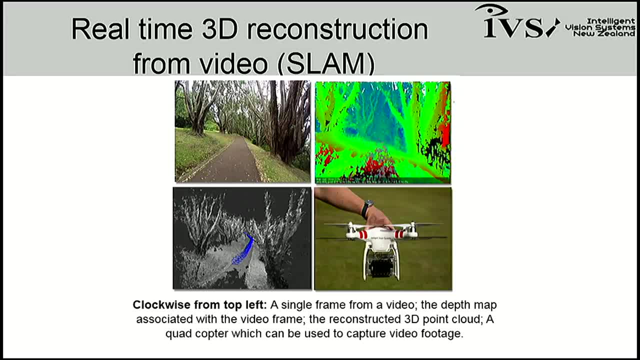 all right, um, the techniques we use is slam. i'll try to go very quickly with that. i. what i'll do, yogi, is i'll go up to the mexican pyramids video and then we can stop. okay, all right. um, so what we use for mapping is called slam, which is so much in this location, and 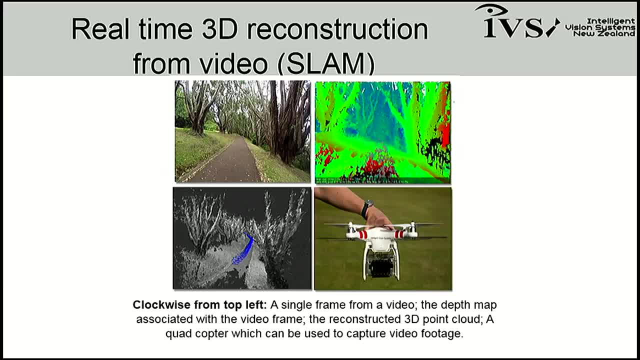 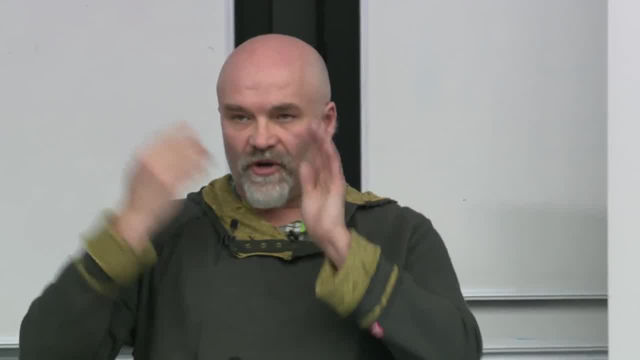 localization and mapping is when you don't have two cameras, you can. basically, a video is just a set of images. when you have two eyes, you see a point from two different perspectives, but when you have a video and you move, it's the same. you can see the same thing. 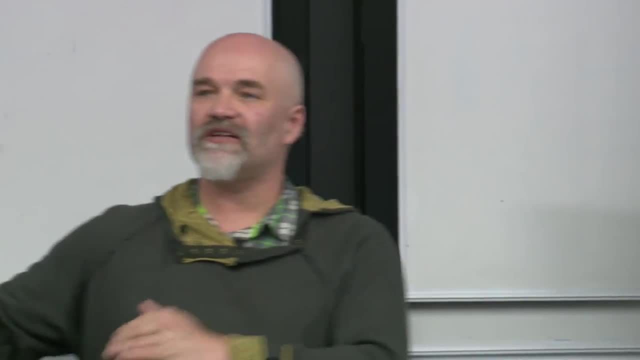 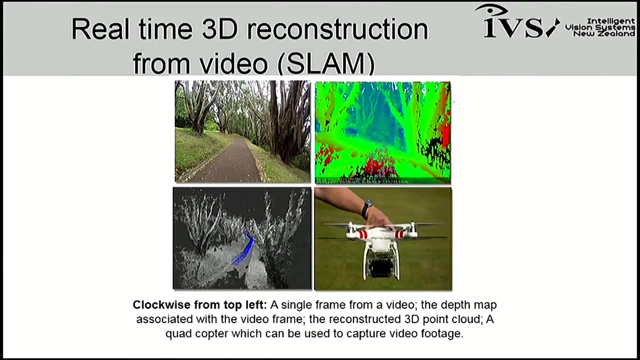 from two different perspectives. if you can sample that, you can create some 3d systems with just one camera. of course, if you have two cameras you can still use slam. you can reinforce your results, make them less susceptible to position drift and movements that basically impair the results. so this: 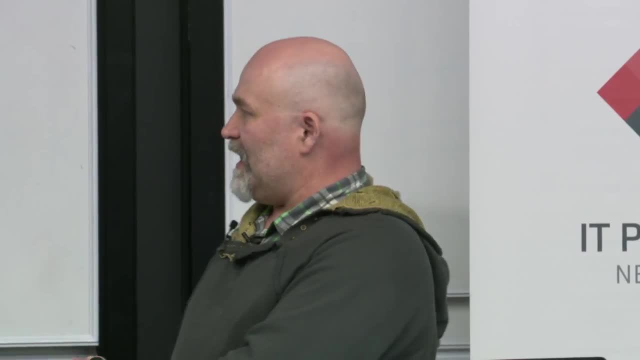 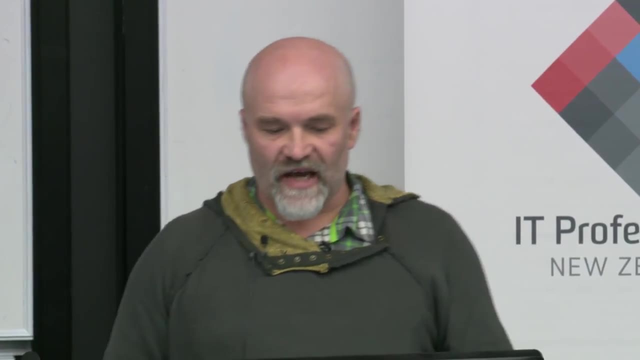 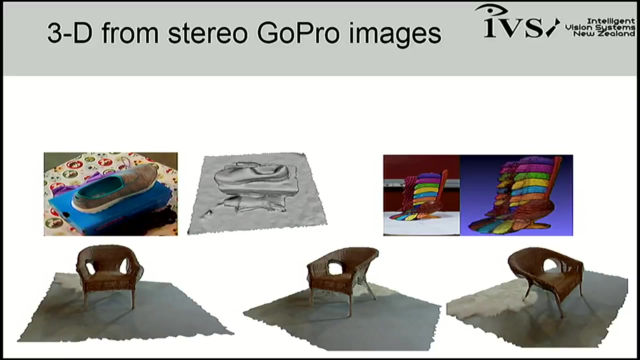 actually this is me walking in the domain and acquiring the data and pretending i was flying that drone, but it's just carrying it because we couldn't do that. but the output is the same. we have a full map of the domain trees. we have tried it on different set of data, both in new zealand and. 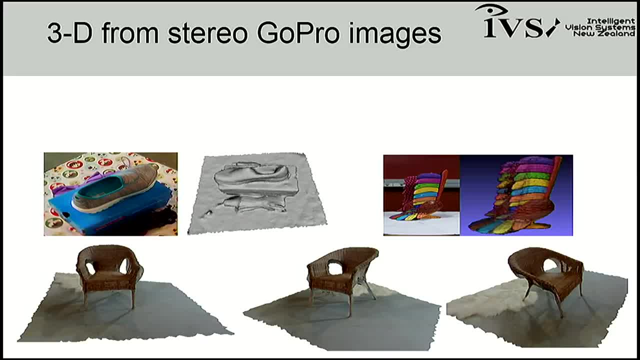 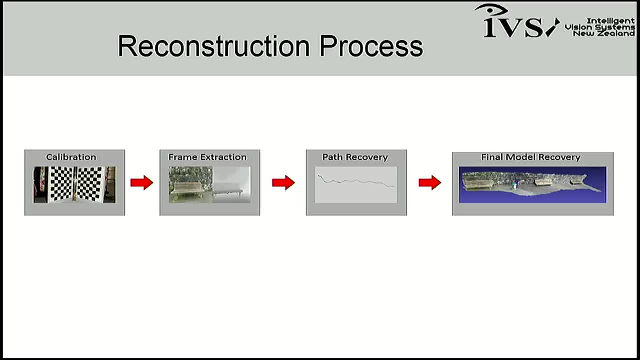 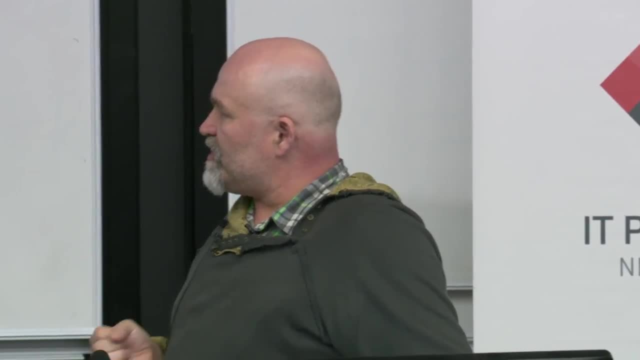 overseas. i think the mobile app has got the owl available as a 3d model you can play with. basically also, you have the bench model. just go from needing to calibrating your cameras, pick up frames, produce disparity maps 3d, recover a path along, correct that improve. 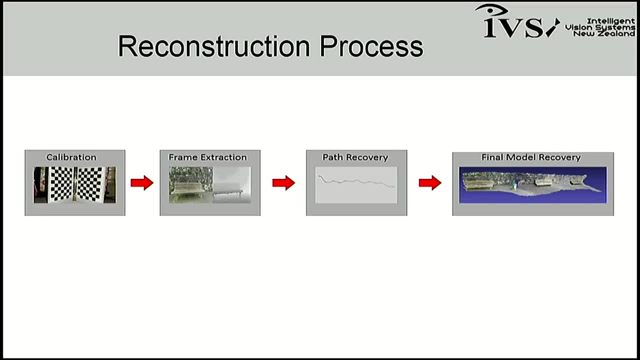 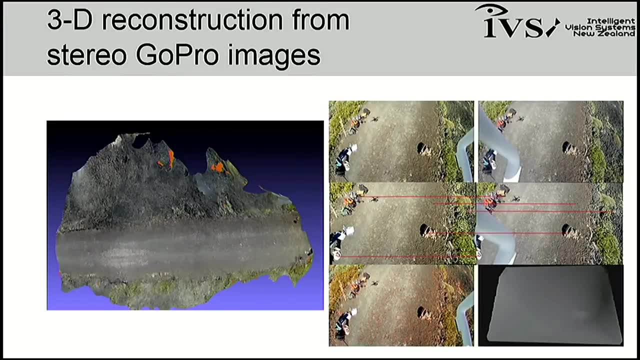 and create that 3d bench. that's a bench from one of the the wall of the ancient garnison at the university right um, if we have a few minutes, we'll go quickly through that. this was in rangitoto where we managed to follow the path and after some adventures we'll be 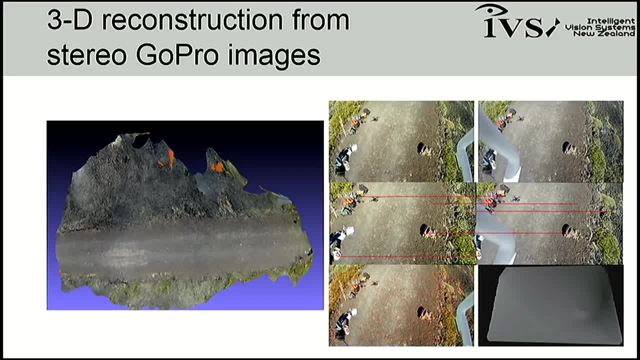 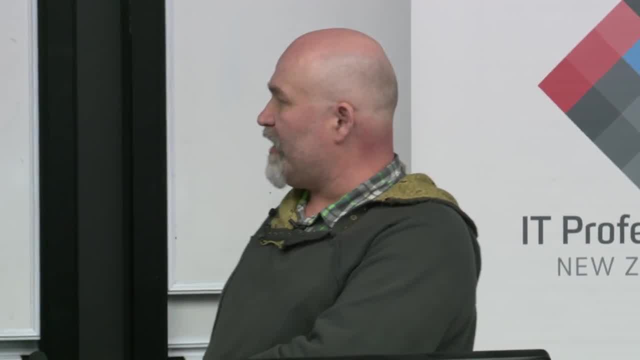 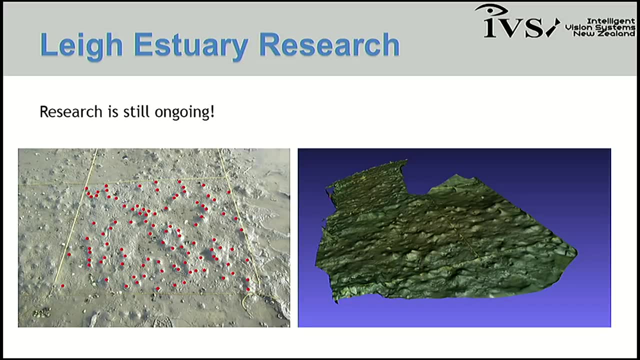 using some blades in the bush, we still managed to get some data eventually. yes, that was fun. the research at least still ongoing. we're going frequently to try to reinforce our data. uni services is entrusted because councils are entrusted, so we need to push that to commercial level, where mihailo has will be in charge, since it's part of his phd. 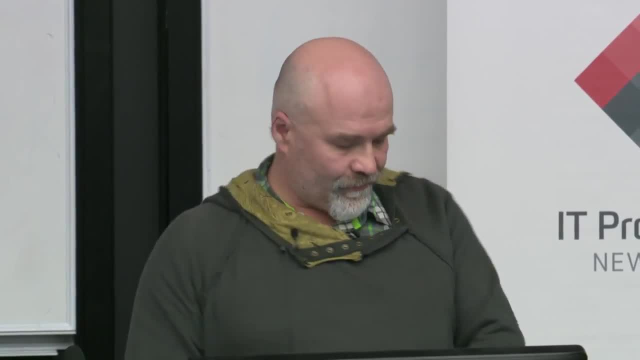 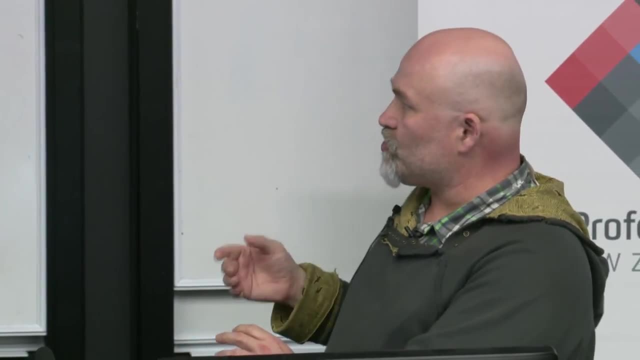 on the right side you can see a 3d model of that sampling. so i'm going to show you the sample data that we just captured from the postgrad students there in two weeks to do the sampling with us. that's what i like also to show. often, science is not 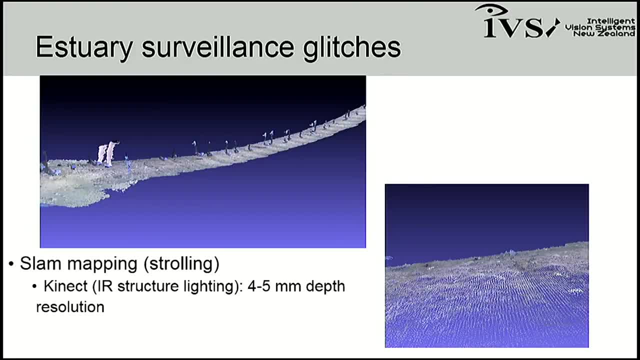 about all succeeding. we have glitches, uh. we said, okay, let's take one of our sampling systems using, uh, one of these, kina- and let's try to make a map of the beach, and basically there were some issues and there was a lot of legs appearing. we realized, too like we're also acquiring the legs of the 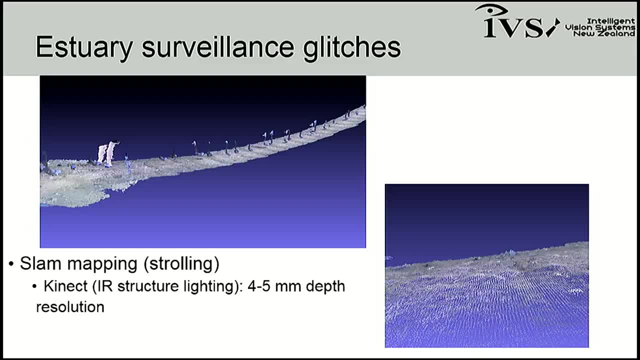 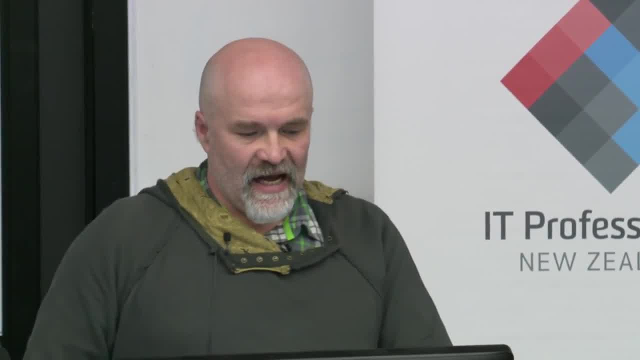 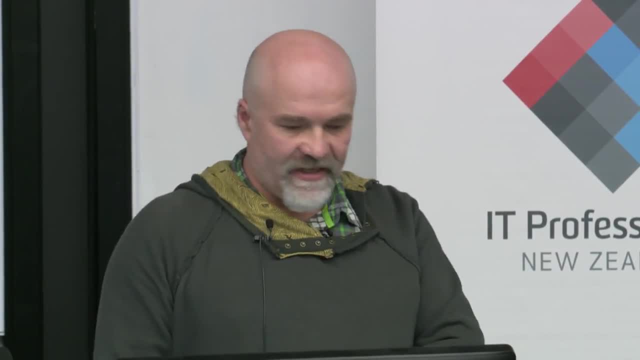 people and reconstructed the legs. every single time same one. Might be two. no, Is it your legs and someone else's? Yeah, okay, Cool, We could extend the scaling and the water and the ground as well. These are two other projects that we have played with, but sadly we'll have to accelerate. I 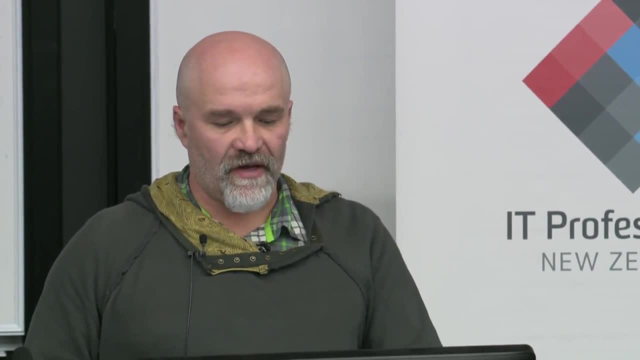 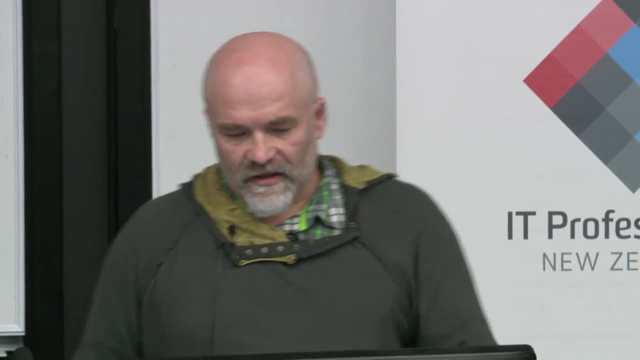 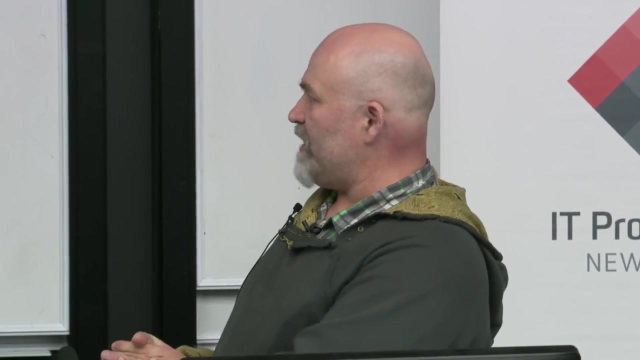 definitely want to show you something I'm very happy with. that was very difficult to put together. Here it is. You have seen what we can do in Lee, What I say: why don't we do that in Mexico? First, because it's a nice place to be. 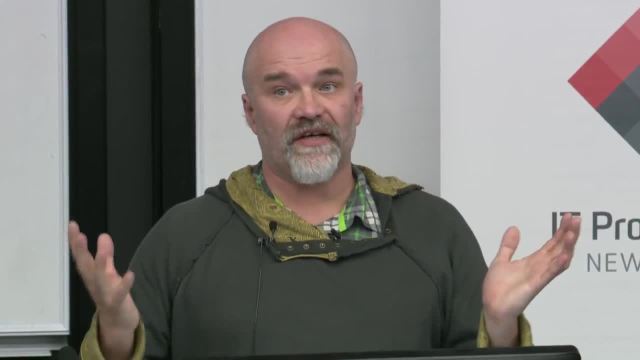 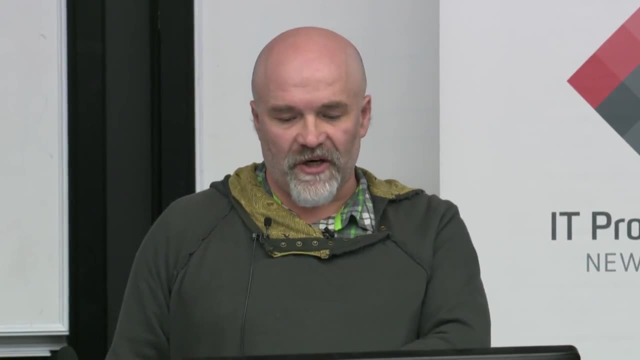 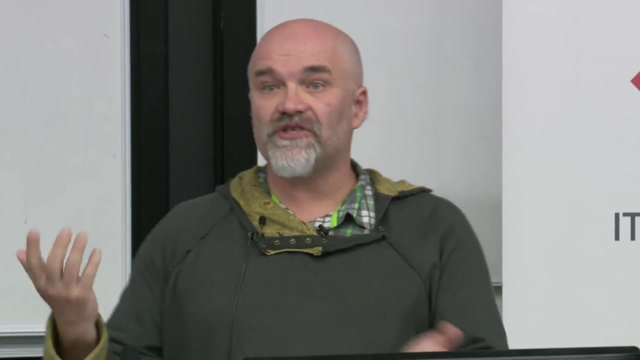 in The food is great. Also, they have lots of archaeological sites and they need to create an archive of that. These sites are being basically some of them. I haven't been open yet and they have taken things away because that sells well. Tourism is damaging these and you have to balance the amount of money you 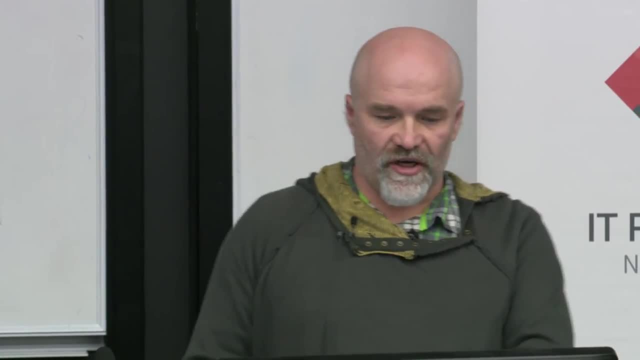 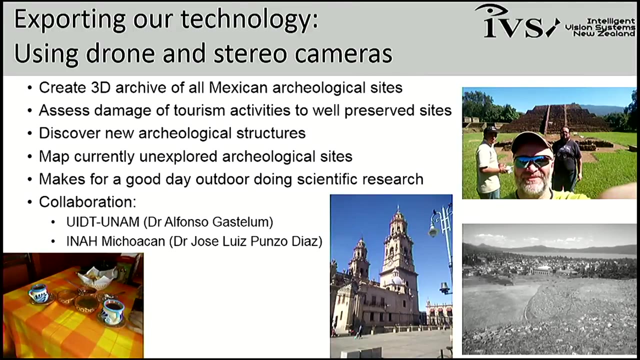 make when you have nothing else to make money, and the damage to the sites you have. Also, in Mexico, there's only about 150 sites open to public, but there's maybe about a thousand ancient towns that they know about, or they expect to know, but they haven't checked them out. So they really want us to explore that. So, Jose, 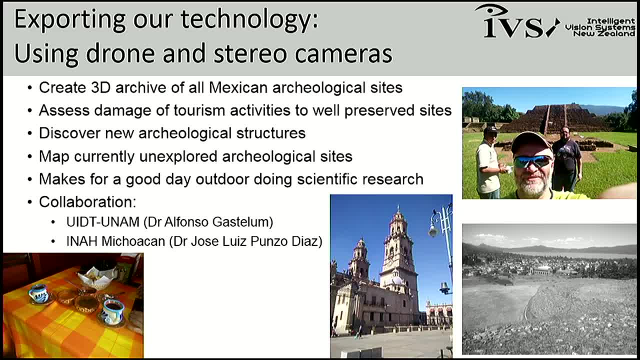 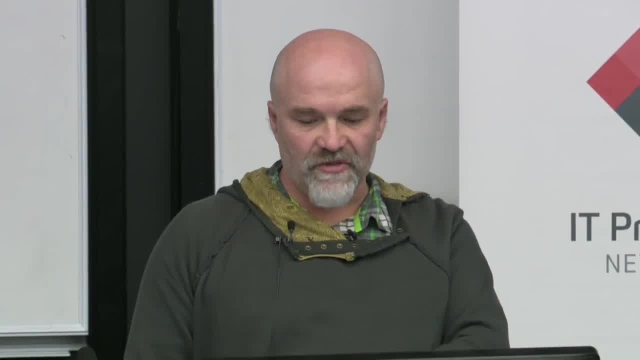 Luis is the boss of the archaeological department in the state of Michoacan, which has got some amazing sites. That's basically what he asked us to do with them, So we had open access to all the sites. We did what is not allowed for. 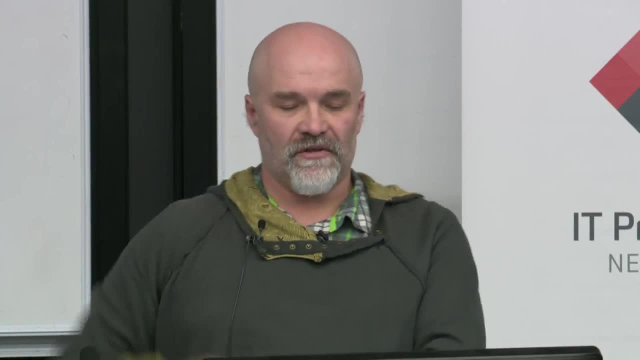 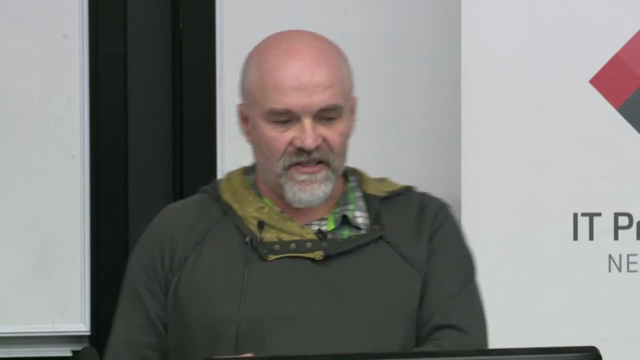 others. We said we want to fly from that pyramid. He said, okay, you go, The others you cannot. Okay. so we went to two different sites and this is Tzintzuntzan in the state of Michoacan. That's the capital or ex-capital of the ancient. 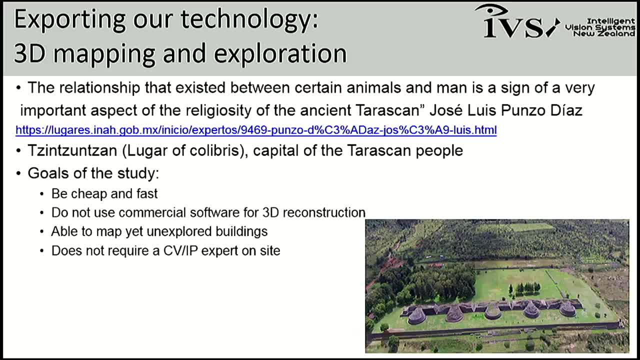 Tarasquean state. Jose Luis is not a specialist in computer vision. That's why it's great. He's a specialist in archaeology. So we learn a lot of things and he learns as well. Tzintzuntzan means the place of the colibris, or hummingbirds. 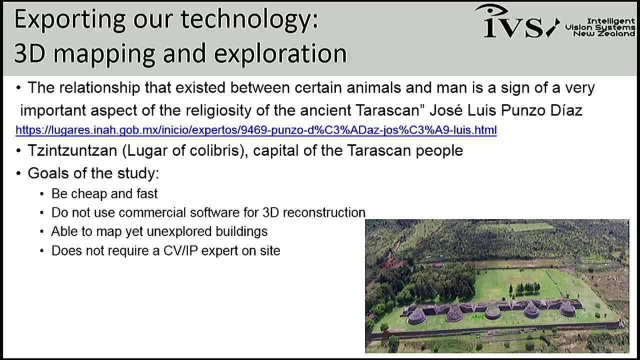 They had a crane coming in a company and that cost them a lot of money. So they said we would like to do that often. We would like it to be cheap and fast. We don't want to use any commercial software, for obvious reasons. We want to be able. 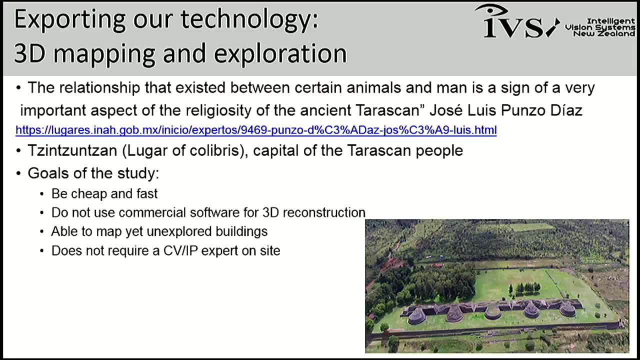 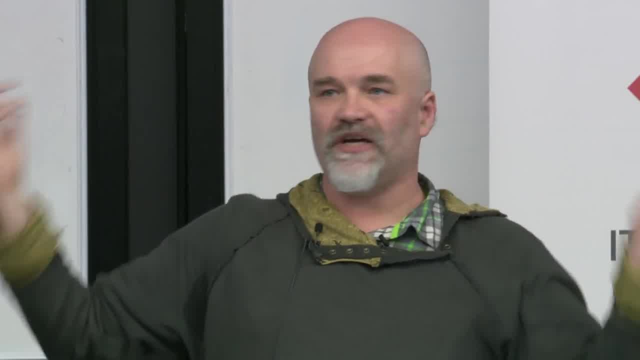 to map and explore buildings and if you look at the back of this, which is the ceremonial center, all the back of it is also part of the town. Actually, he said everything two kilometres around is part of the ancient town. We would like to image everything. 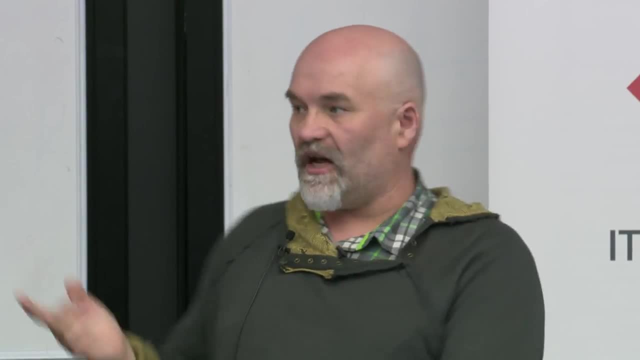 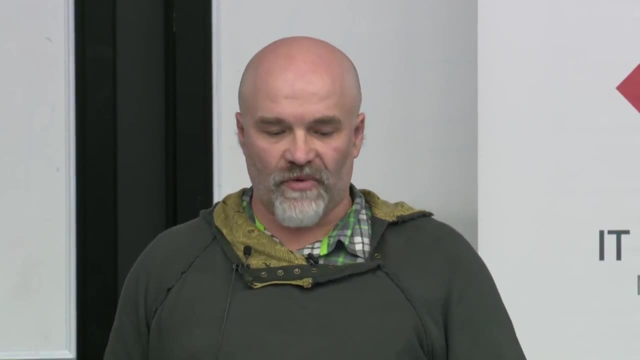 And he doesn't want me to come back every time, Not because he doesn't like me, but because, well, I cannot be there all year round. So he would like the system to be deployable quickly and we can basically provide the data on the go. So there's. 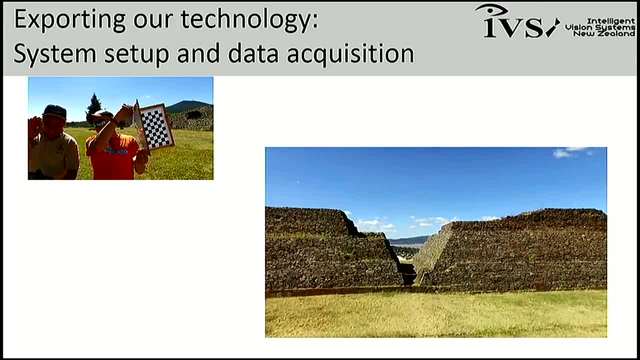 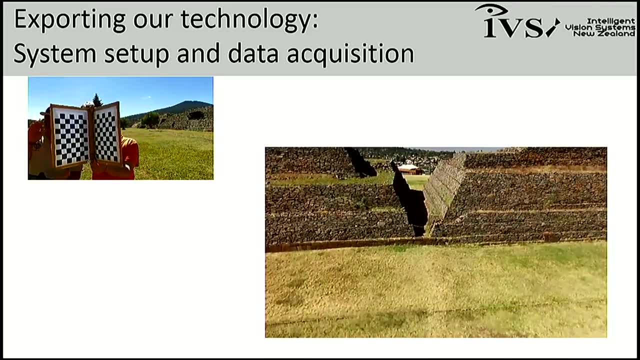 two more slides, Kyogi, and then after you can interrupt me. So we were there in November. We used some of our in-house calibration devices. We explained to them exactly how we wanted calibration on the ground to be placed to ensure flatness, on the ground to be placed to ensure flatness. 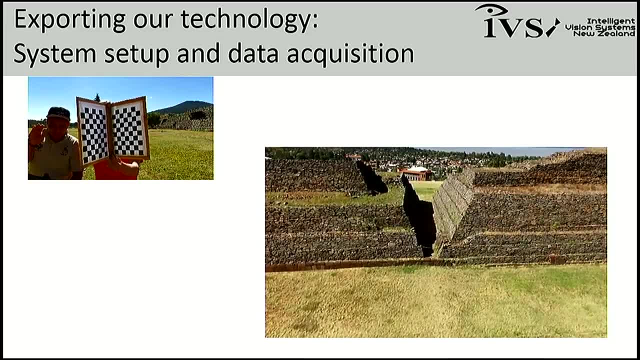 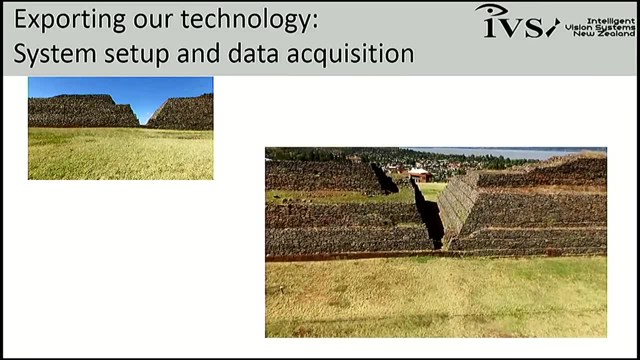 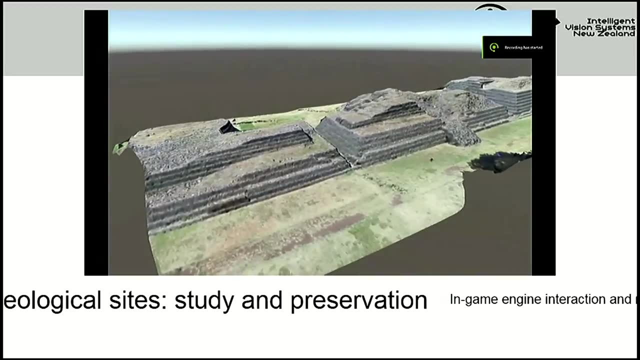 of all the data And we flew through the pyramids. At the back you can see the lake of Pátzcuaro and the new town of Tsintzúnzán there, And we'll show you a 3D model of. 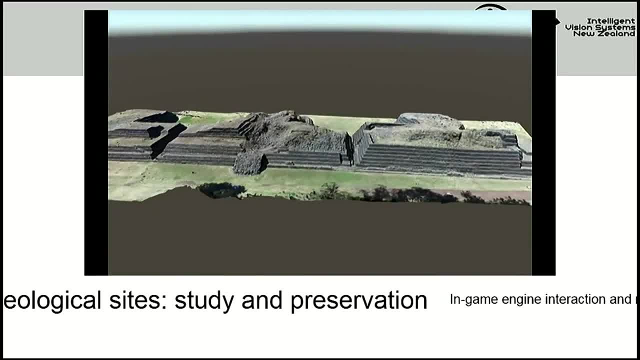 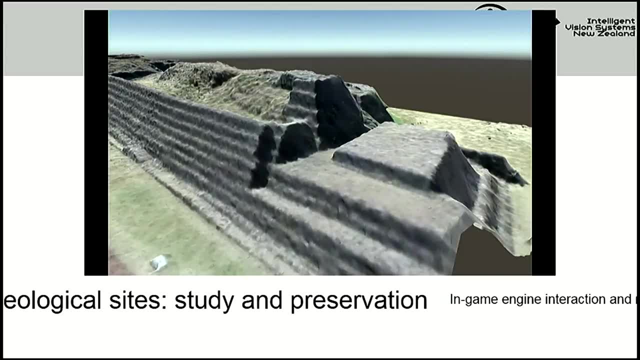 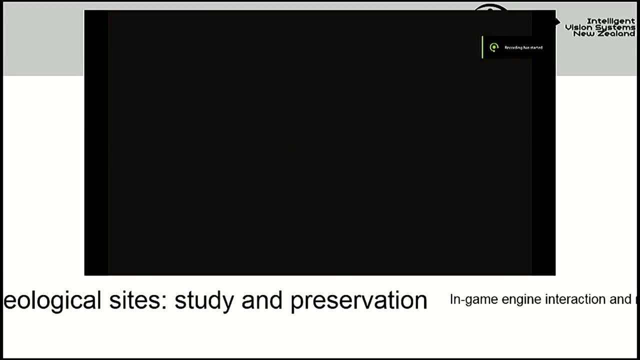 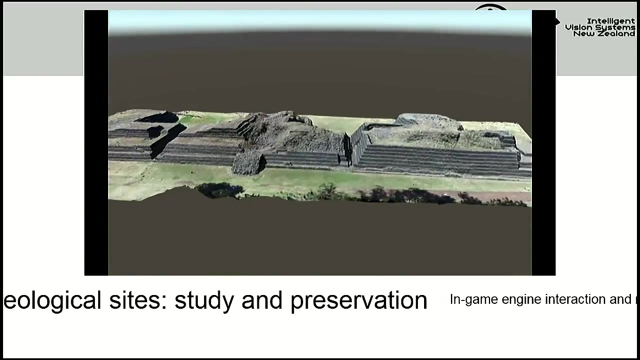 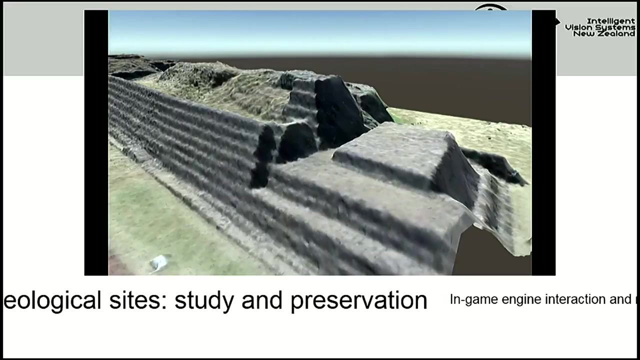 the pyramid that we created. I don't know what the voice is about. Basically, we have reduced the texture level to basically make it manageable. This is an output of the work from Trevor PhD, And basically we're continuing the project with the Mexican DCO. So hopefully Trevor will come with me in Mexico. So what they? 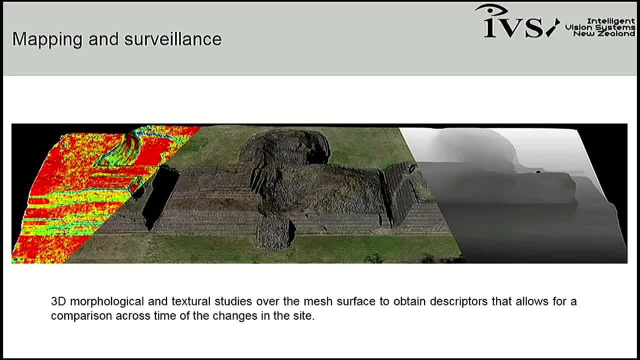 really want to use that for is you have the temple at the center On the left side. you will have curvature and mesh properties and depth And they really want to assess whether actually there is damage to the structure and where they need to make progress. They 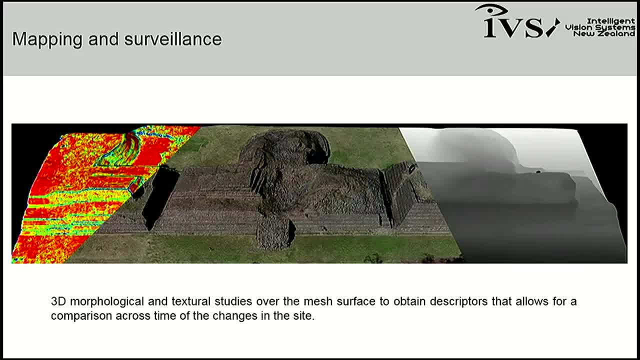 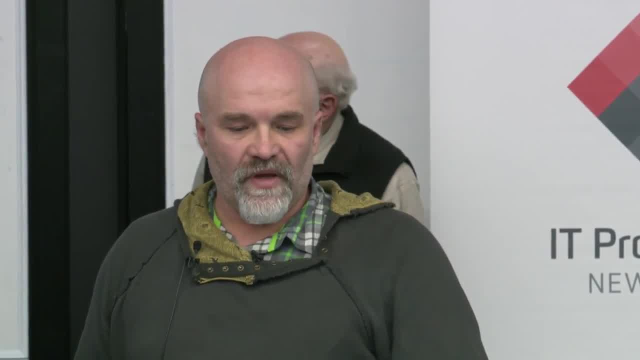 don't have the capabilities to maintain all the sides. Right, We could talk about the hour, We could talk about a lot of things, But I think we ran out of time. Just maybe. just say: if you want to go to online resources, you will be able to see. 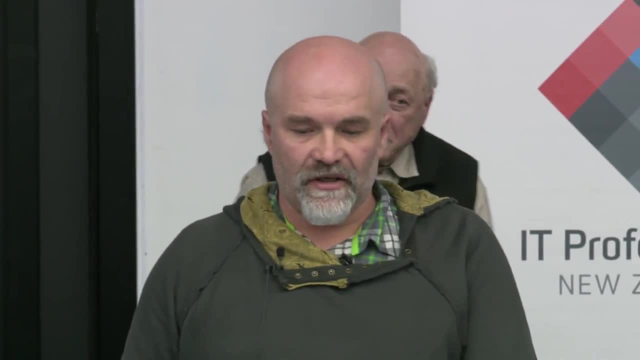 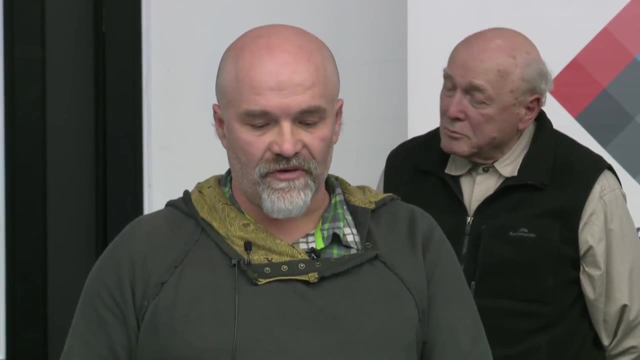 a lot of data there. I encourage you to go and check what we're doing. We are fortunate to get money from the Vice Chancellor To be able to continue research in this area and develop more of these tools that we're using. We don't look about that, Okay. So to conclude, and that's my last slide, 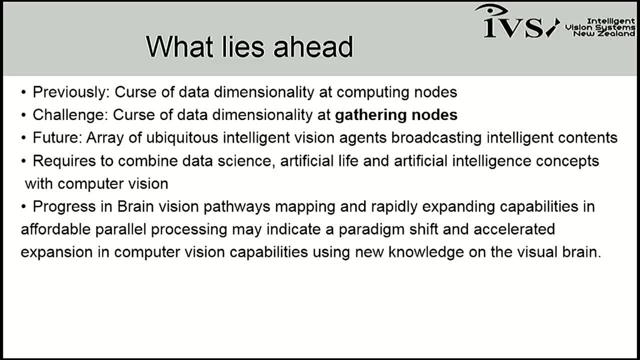 Of the many I can continue with. No, Okay, We used to have what we used to call a curse of data dimensionality at computing nodes, But this is less true nowadays. When I did my PhD problems, I couldn't process the data I had. 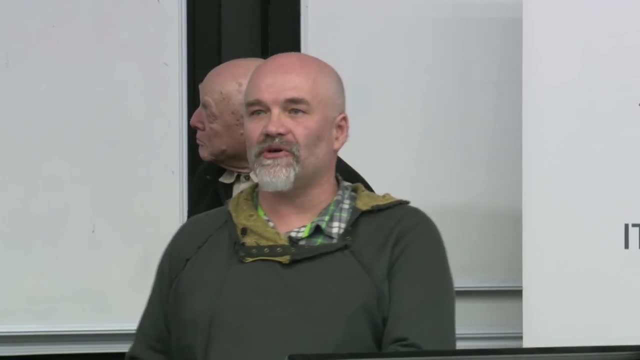 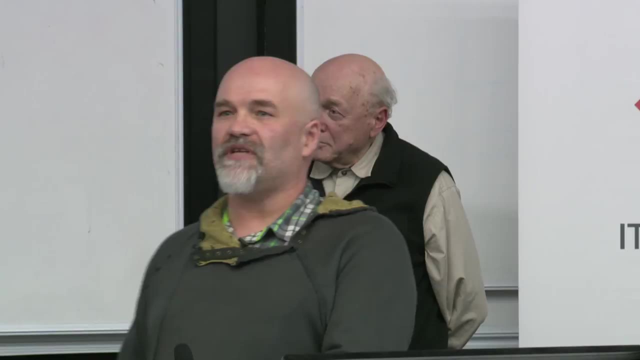 My computer couldn't hold the data My processors was not able to. Today I can take my whole data. put that in the RAM. I don't have enough, I buy more. I need a terabyte computer of RAM and four GPUs. That's okay, It's $20,000.. If it's a big 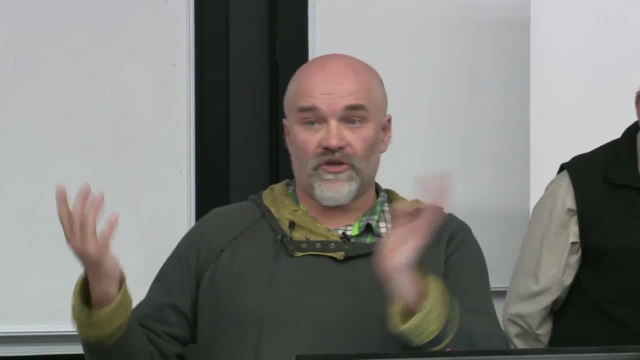 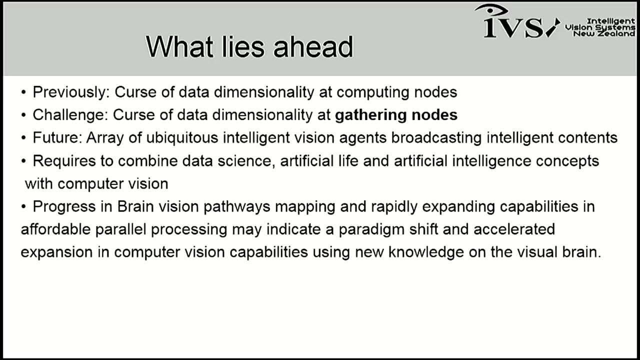 project. it's affordable, All right. This was not available just five years ago, So this is mostly gone. The problem now is at the gathering nodes. there's too much data being created. If you transfer that all back to the system, you're not gonna. 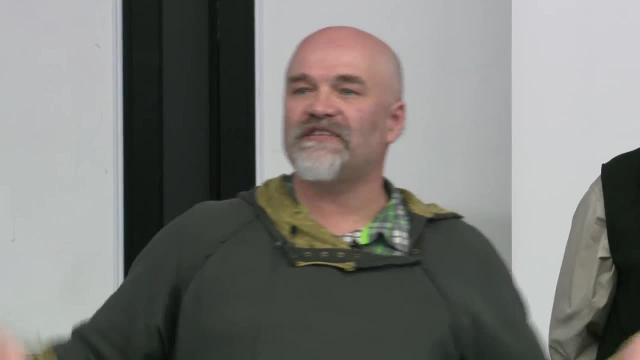 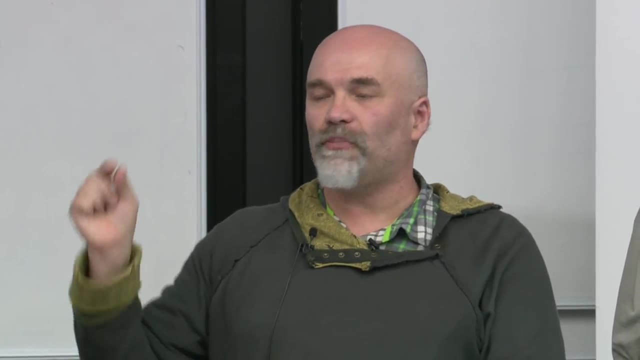 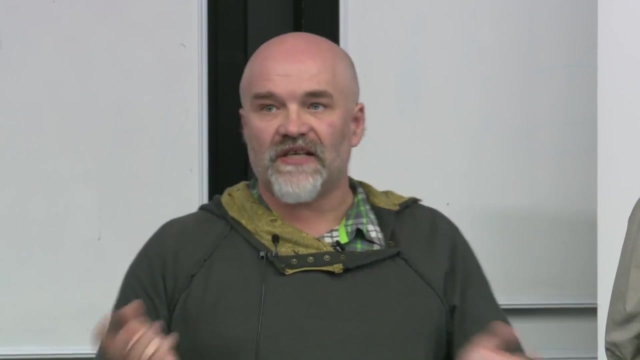 make it. Chicago is implementing an intelligent network of sensors and the guy said each node creates terabytes of data. What do I do with that? I cannot store the data. I need to process the data at the node. All right, And this is the novelty of it. So, basically, this is: 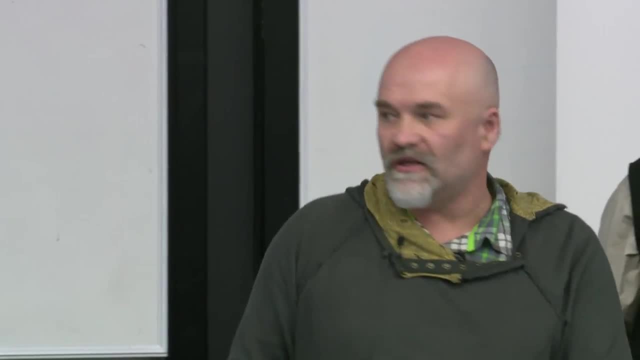 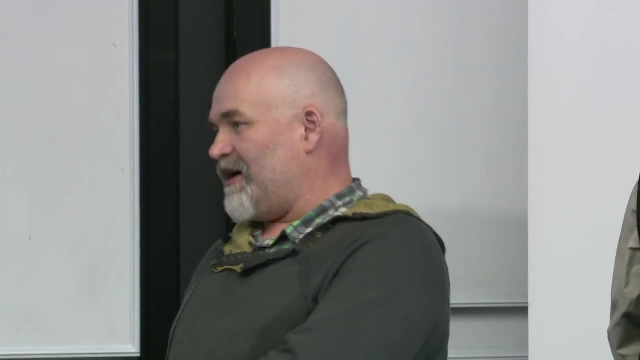 our point. We want these ubiquitous intelligent agents, such as the ones Bella is working on, to roam the beaches, to roam the forest and anywhere in New Zealand. That's your job, Um- And basically to be able to do that. So we need to be able to do that. We need to. 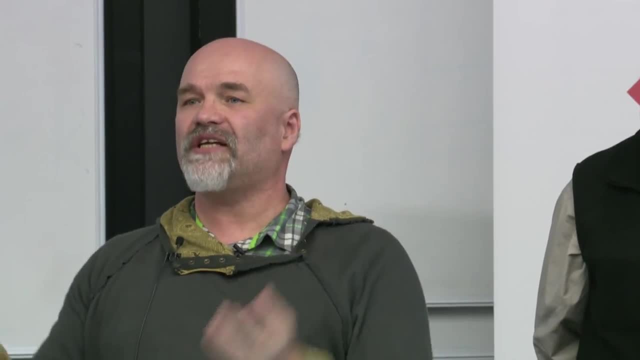 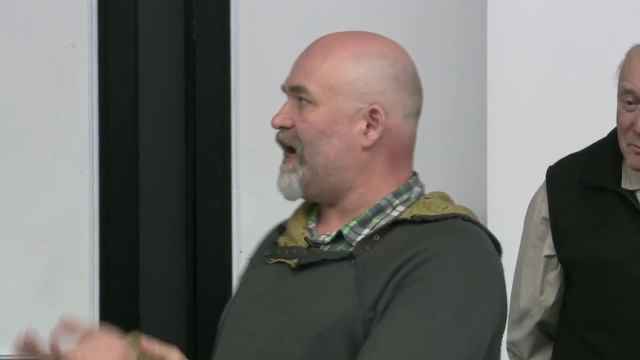 be able to collect data, but not just random data. It's to already analyze the data, Know what's in there And to transmit only what's meaningful to the central systems. All right, You can do that on your own. You need a multidisciplinary approach, You need data scientists, You need 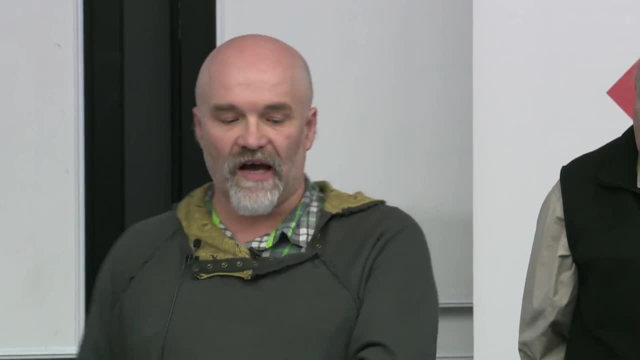 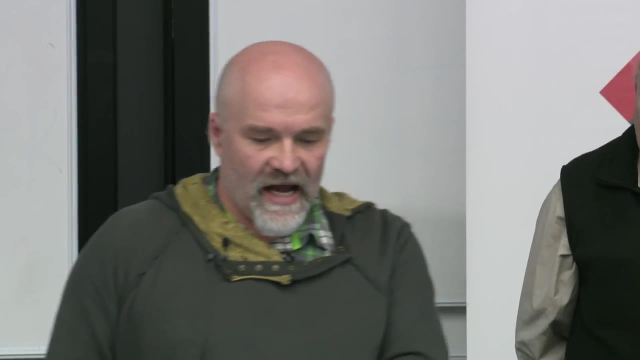 people simulating these type of agents through artificial life systems. You need artificial intelligence to create the algorithms And, of course, you need computer vision. All right, The great part is that we don't know how our brain is working, but it's progressing fairly. 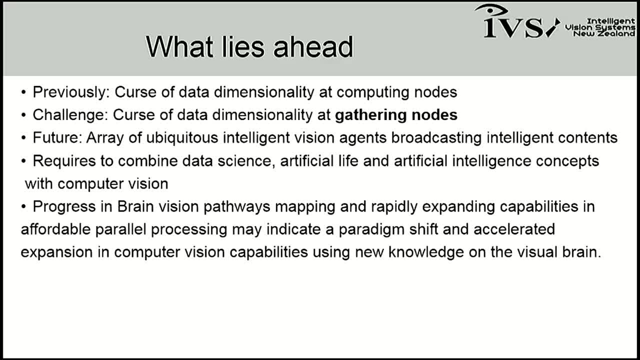 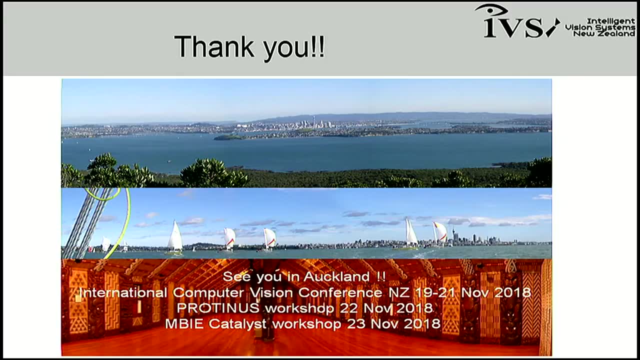 fast So we may have a chance to know enough in 10, 20 years to not emulate the full brain, but maybe a bit of the visual brain. And we'll have a conference in November and workshops. You're invited to join us And thanks a lot for your patience. 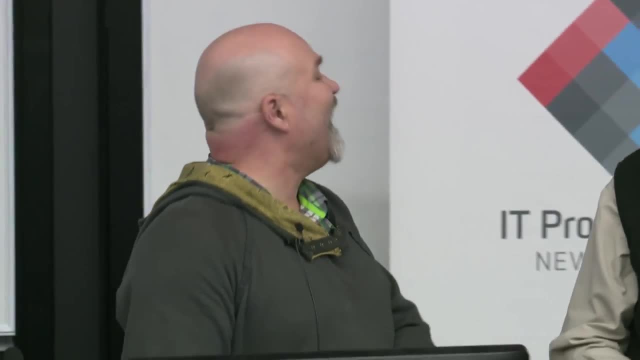 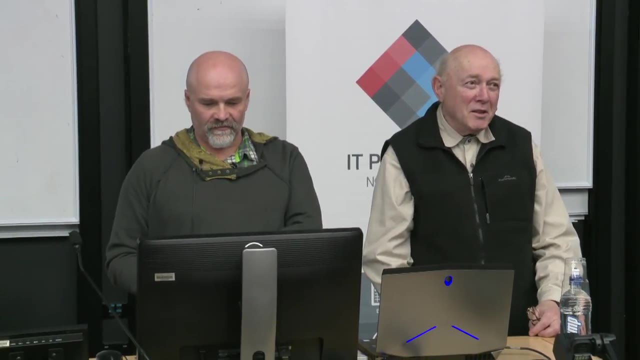 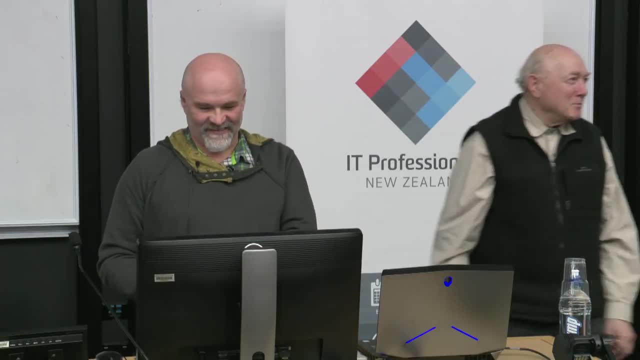 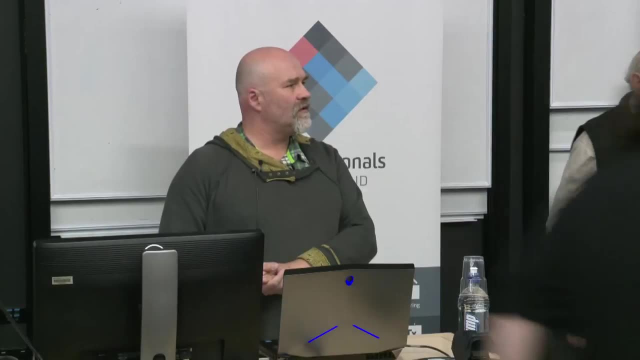 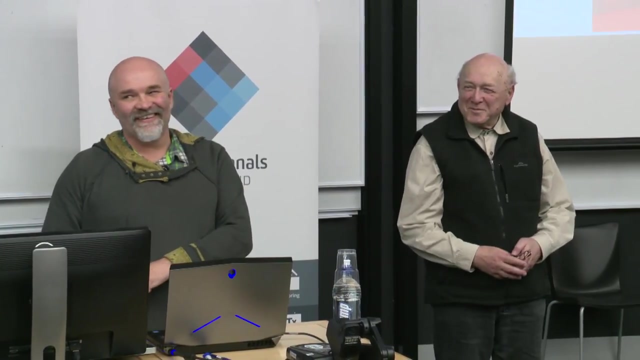 Yeah, That implies 50 shades grey. Just in case I cannot talk for you, I cannot talk for Onley. Oh, I'm excited, I'm very excited. Thanks very much, Thanks, Thanks, Thanks, Thanks, Thanks. 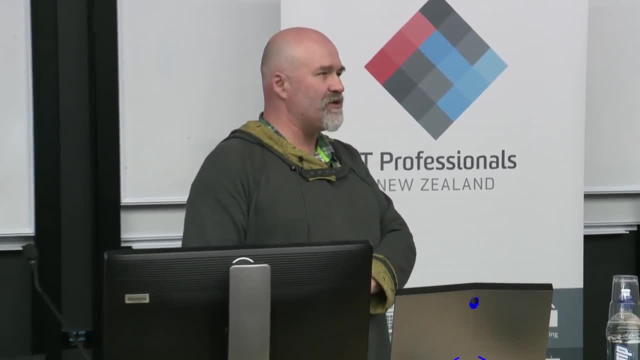 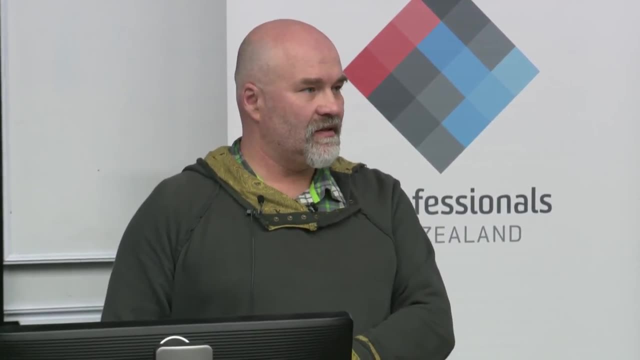 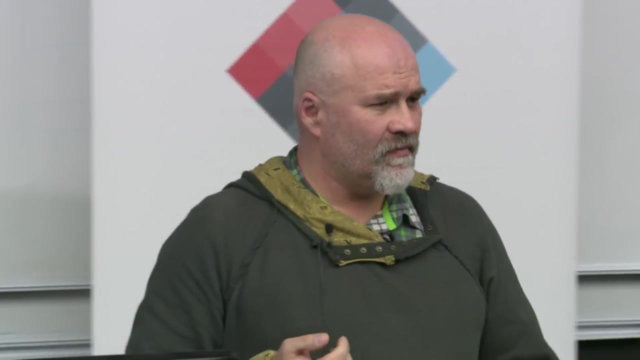 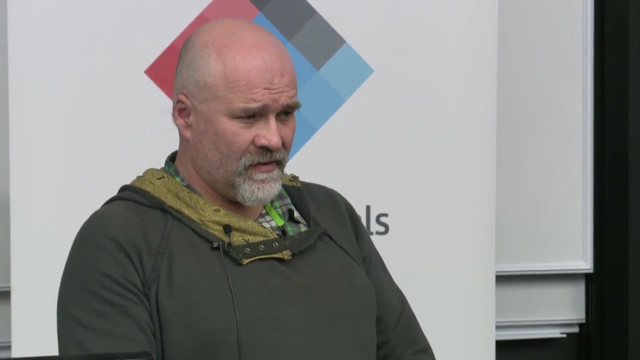 The books are horrible to read so I didn't watch the movie. I thought that would be worse. I'll take it back to the comparison between the human brain and machine systems at the moment. Yeah, You were saying that at the moment there's no comparison. between the 10,000 nodes of a machine compared to the billions inside a human. But it's also true that the human processing power of neurons is only about 200 per second, whereas the processing capabilities of computers is in the gigahertz. 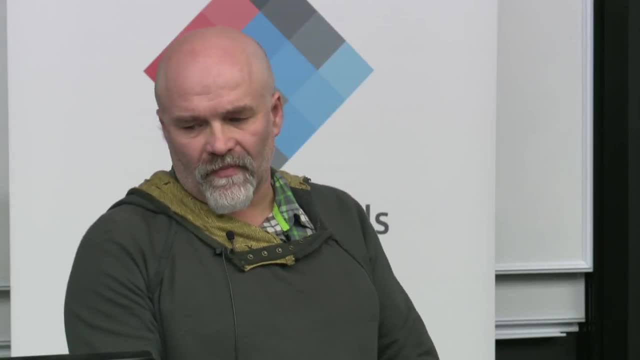 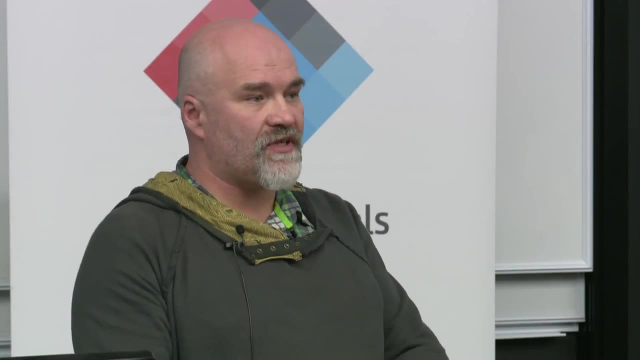 So I mean, does that kind of even it out? I don't know how we can say that, Look, if I take a robot with cameras in any given situation where humans are able to solve a problem in most cases, what I didn't say today. 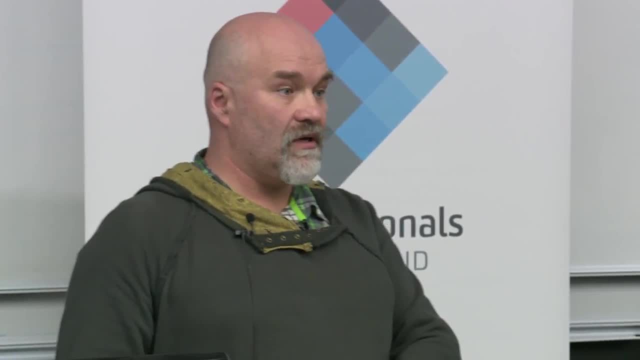 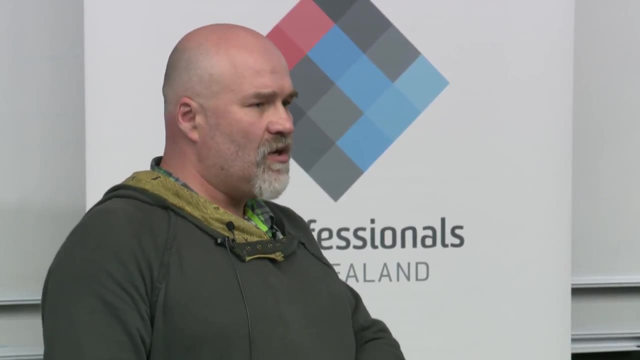 is that In most cases, what humans can do, robots cannot, And what we humans cannot do are not made to do robots can. So that processing power, as I said, it's not just about processing power, There's all these different senses that we integrate when we visualize. 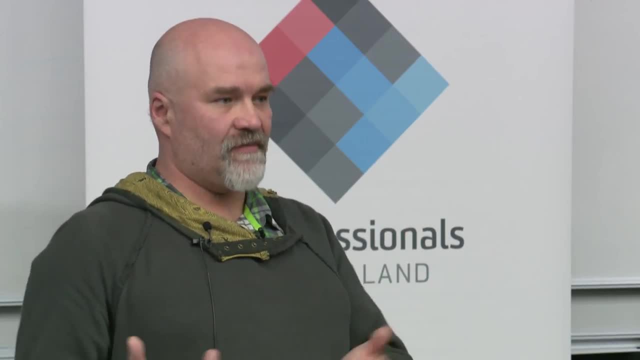 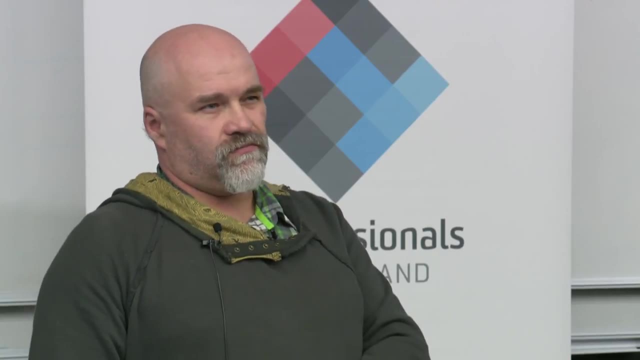 What we perceive is not what we see. It's what we make out of it And the way we model this world. I'm not really sure how this works. Is it more of a software problem than a pure hardware problem? I think it's theoretical problems. 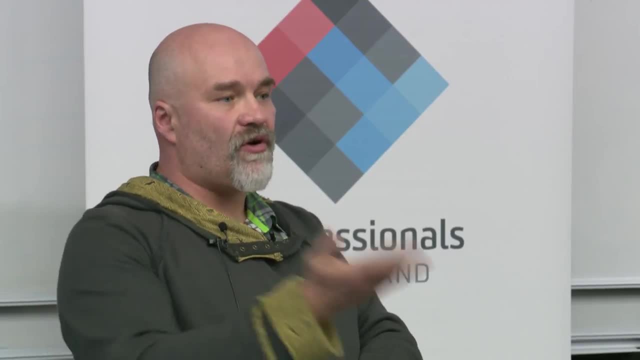 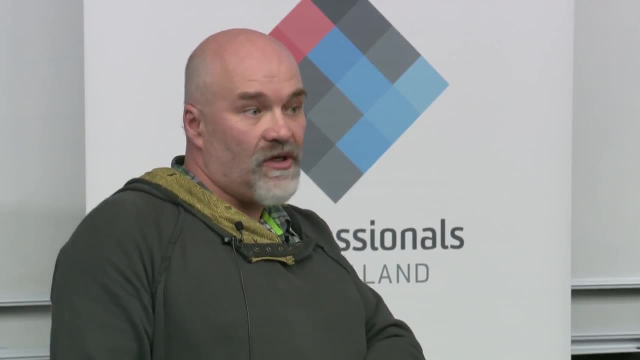 We don't have any models that actually can. If your question is: is it just a problem we cannot model what we do as humans, because we just don't have enough processing power, the answer is no. We don't have the models. We don't know how it's wired in the brain entirely. 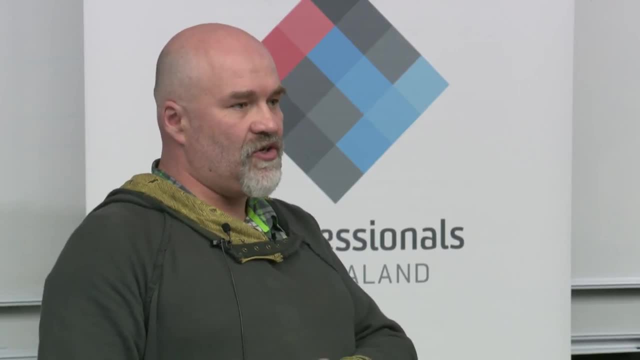 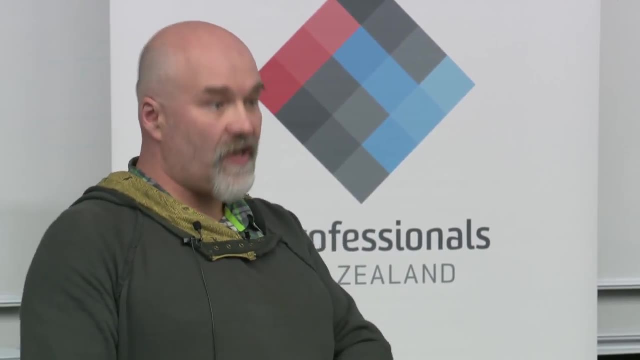 which parts are activated or not. So there's a long way to go. You need at least several generations of improvements, not on the neuroscience, on the imaging equipment. It's not good enough. The resolution is not there and there's at least two or three steps. 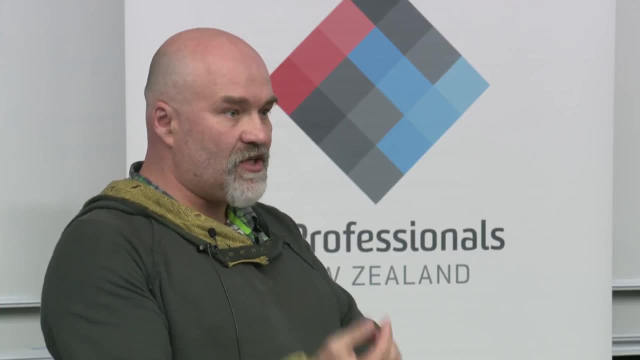 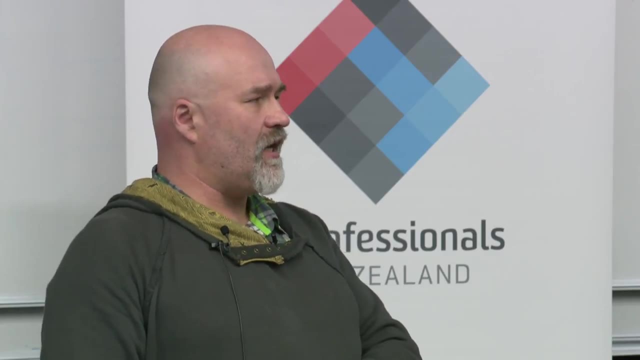 which means 10, 20 years before we can see it. We need to see something Another 10, 20 years before we maybe we can model things properly. So 40 years I can retire at 89.. I can beat you, Georgios. 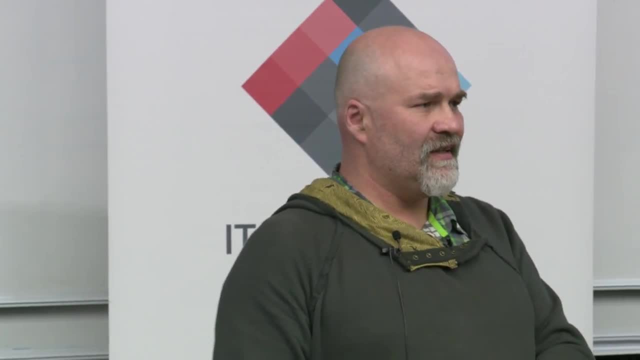 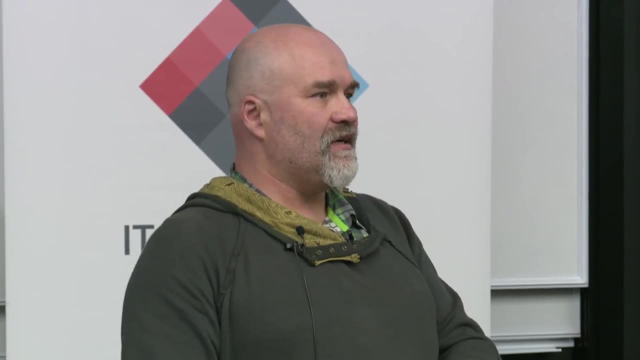 Yes, So is it too, say it's brute power, it's number crunching. brute power versus extremely elegant, sophisticated human cognition. Yes, that's why I don't. Is that too simplistic to say that? No, that's really that. 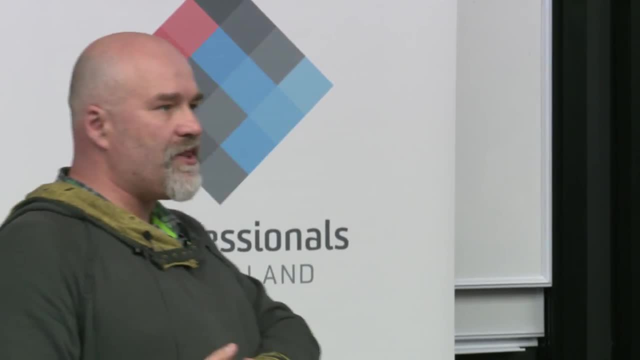 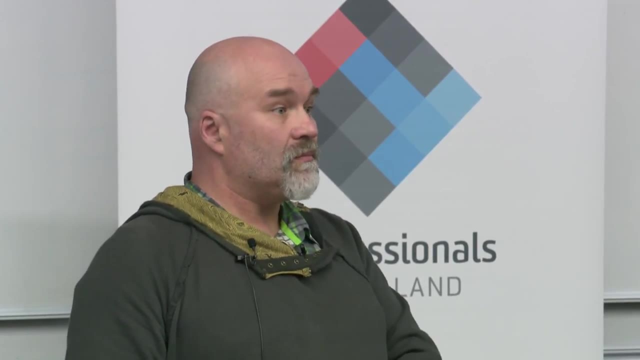 We don't know what's going to happen. what's happening? So if we could model what the brain was doing finely properly, then processing power is not necessarily an issue, All right, But we don't know. As simple as that. 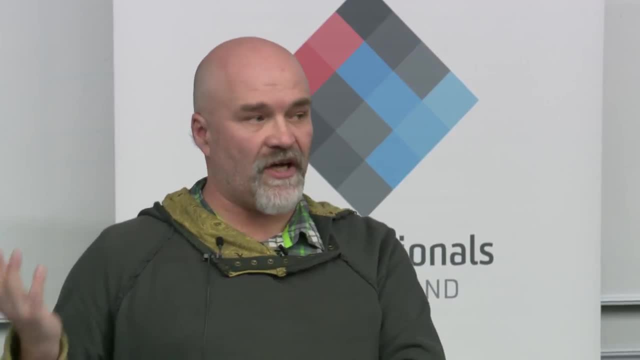 You can look everywhere. The people I talk to that are actually doing neuroscience project in Japan. they say, well, can you help us see beyond that? And I say there's nothing to be seen. Yes, we're missing the data. 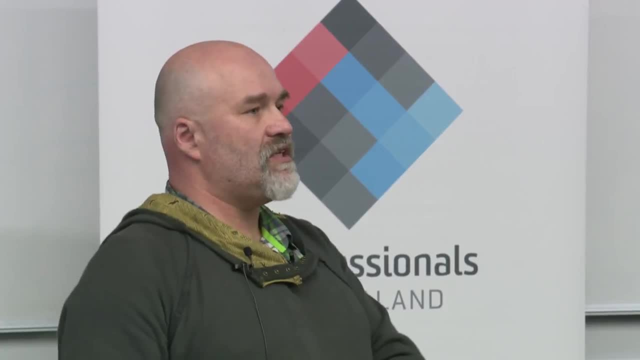 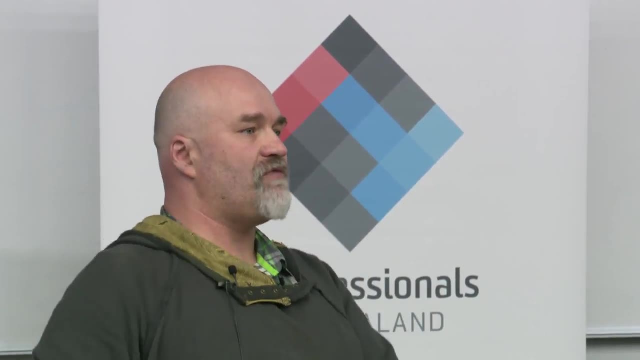 You need to connect that. I say I cannot do these things. There's thousands of neurons going one way, going the other way and in between it's lost, And they want to really be able to connect all of them. There's a scaling issue there with the fMRI and CT scans. 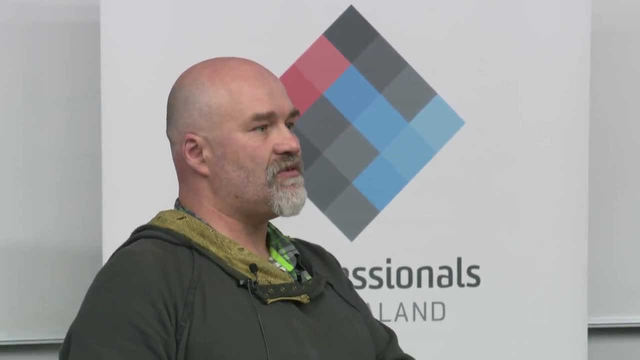 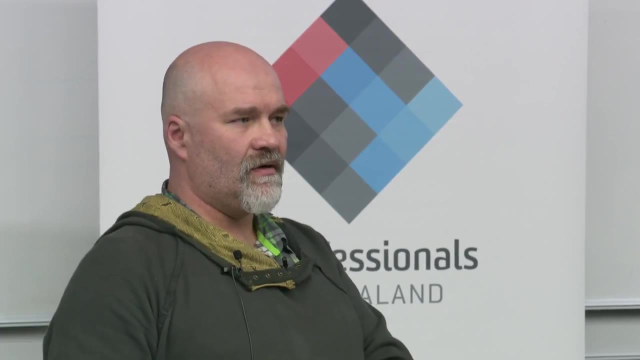 that are not yet capable to see what we need to see. So is human cognition lossy, Lossy. Can we try a lot of ways? Can we try a lot of data away? Yeah, Yes, We're good. Yeah, Well, I'll give you that. 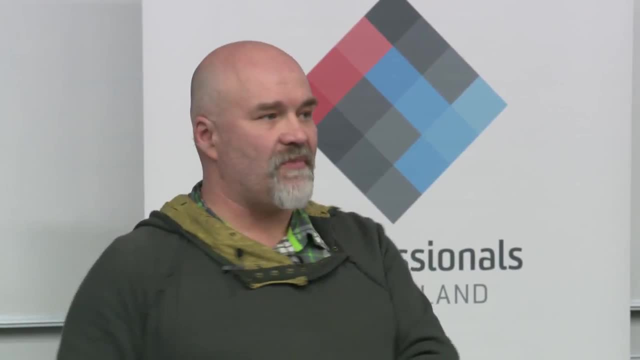 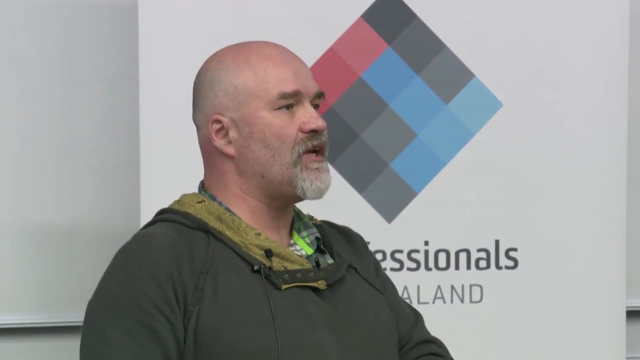 When you see, We were looking at a pre-Mentis image the other day and I did a bit of processing, I transformed that in a black and white one And I could still recognize that was a pre-Mentis image. So how much do we need really from what we see? 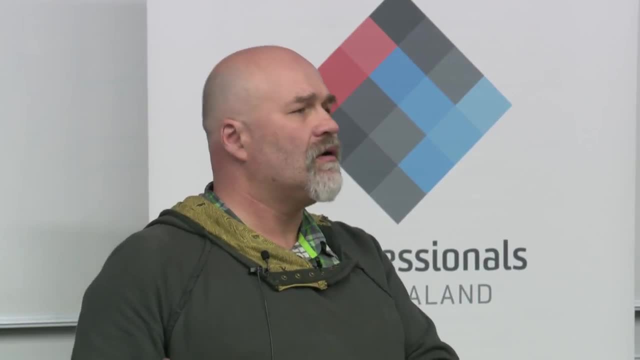 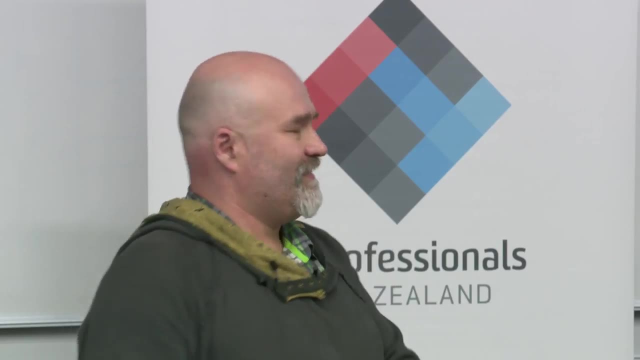 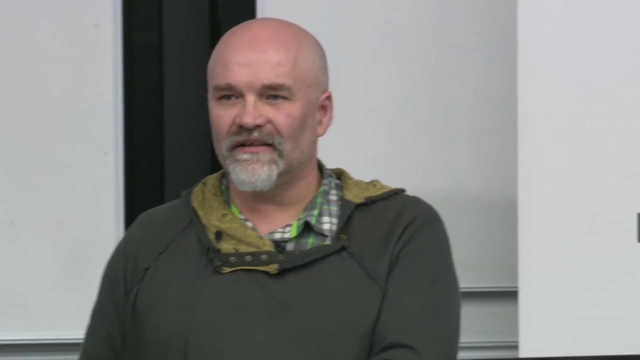 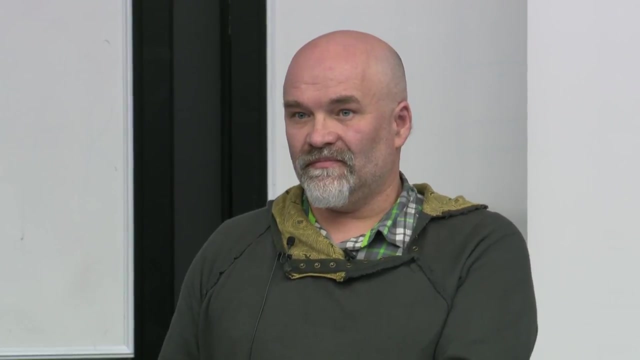 This is why people say, oh, 40 million pixel phone, What for? I mean, come on, I still want that phone, but Have you thought about using dynamic vision sensors for yoga, Such as, Like the DBS camera from the treatment during? 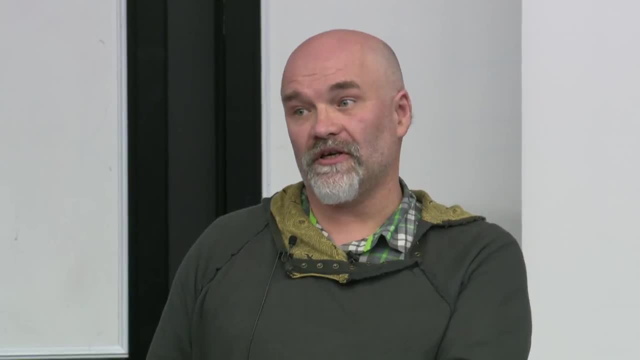 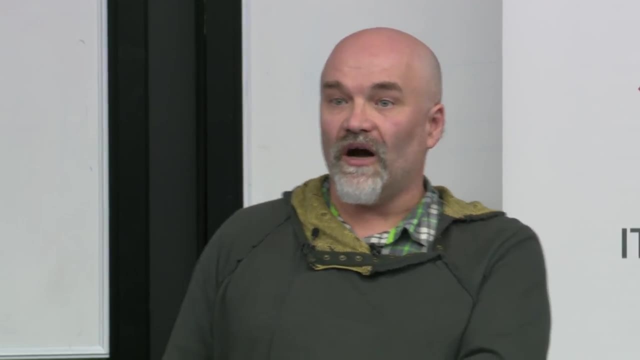 No, Okay, But I would like to go to Zurich so I can talk to them. Why not? No, there's. So to give you a more serious answer, right, It's important. I don't know how heavy that is. 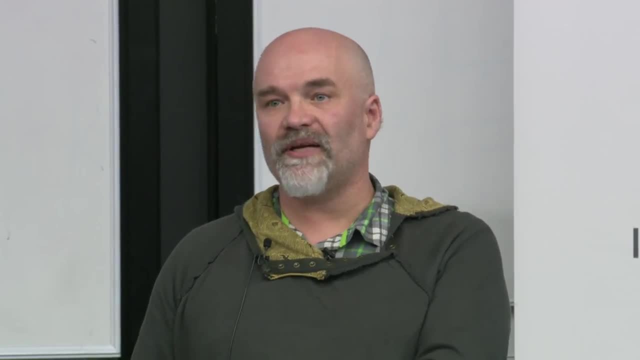 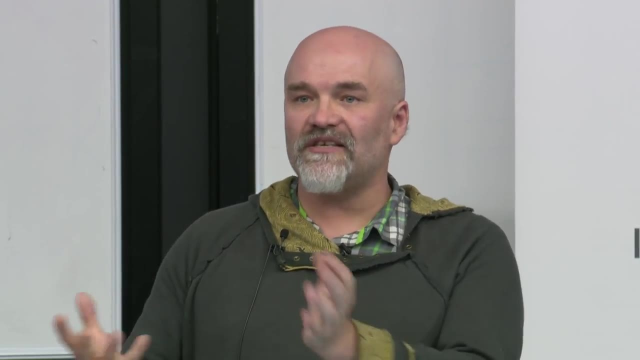 I don't know how much processing power they need, how much battery capabilities. We're really at the How can I say? We're really at the edge of what we can do at the moment. So I don't know. Our system is not like. 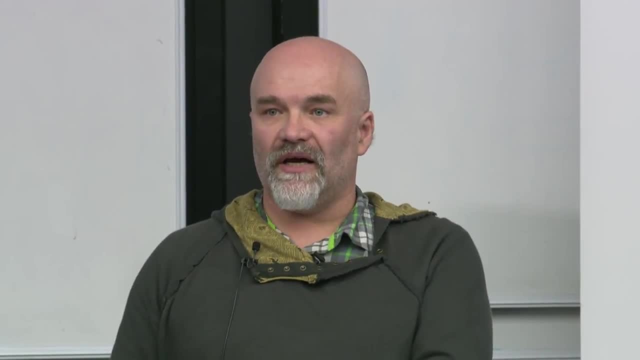 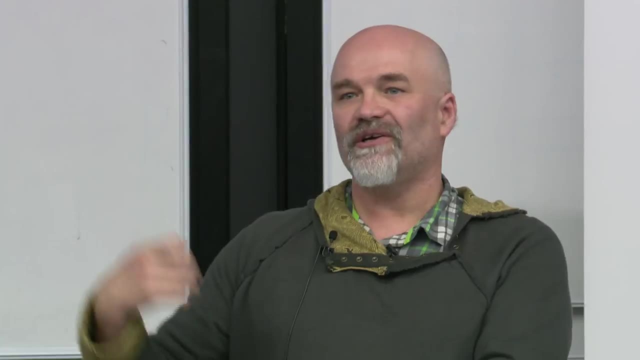 We don't have a plane, We fly 10 kilos and we're happy with that. We're really struggling to just carry what we need and we buy new systems every two, three years. because that's not Two, three years? because that's the cycle to buy lighter and cheaper systems. 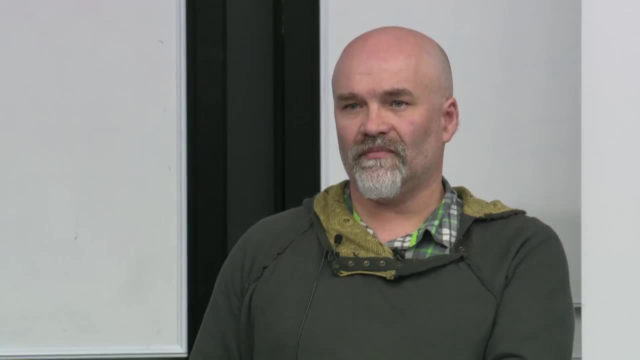 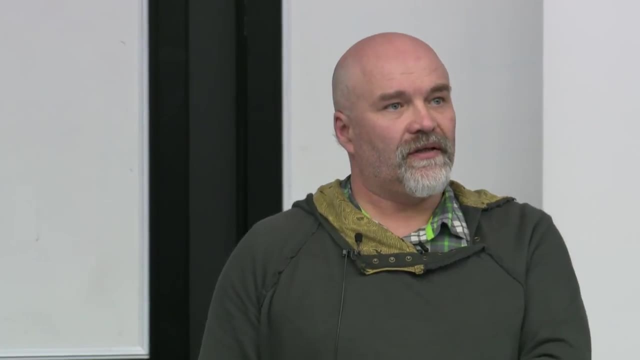 They're actually more powerful. It doesn't use a lot of energy, then. Okay, Well, that's a good point, though, so we could look at it. Why aren't you doing the performance in the cloud or something where you just upload the image and 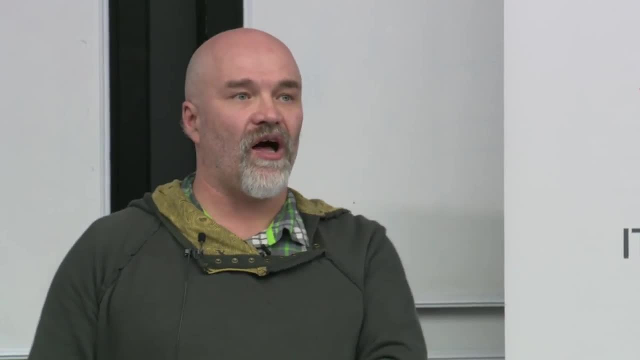 All right, Okay, Very short answer. There's no cloud in Fungatio Harbor, There's no internet there, There's nothing. So But that's a reason why That's the same we've discussed with Bella for a project. 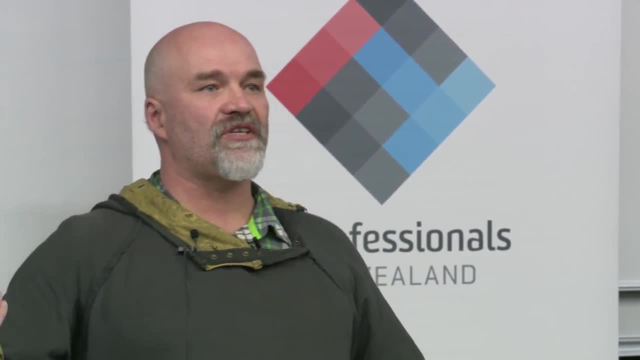 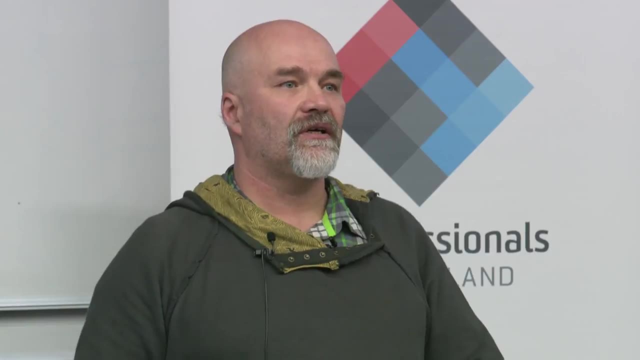 Okay, The robot is isolated in New Zealand in a far north beach. There's no Wi-Fi there, And if you use Wi-Fi, how much power do you need? Isn't there somewhere that you need to survive? A robot is on survivor mode. 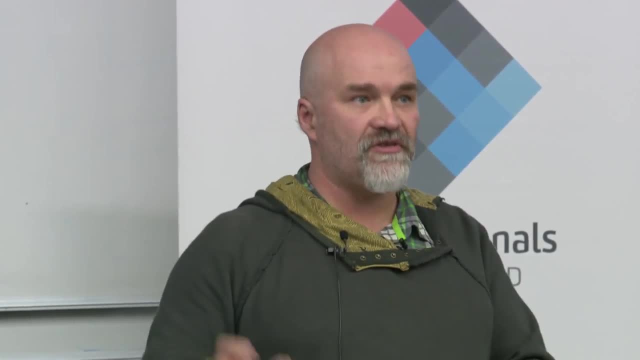 It needs to be able to have enough energy. Are you gonna start using the Wi-Fi? Do you see what it does to your phone? No, you don't want that. So what we want is these tiny agents to be able to roam around. 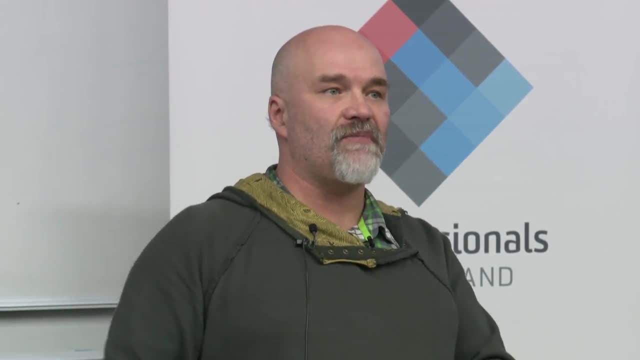 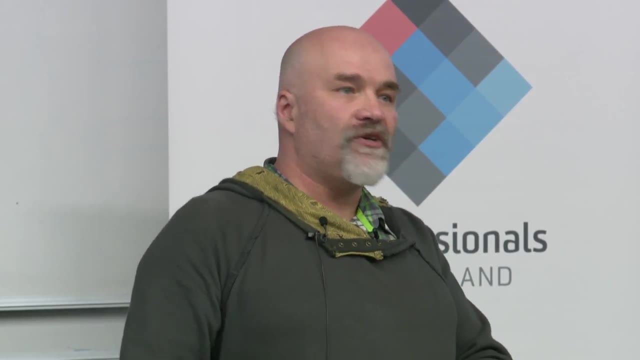 gather the data. keep only the data they need because it's gonna be limited. go back to base. If they have something meaningful to transmit, they will. And the good thing is you transmit new data, your cloud system. of course, we use the cloud for our web server. 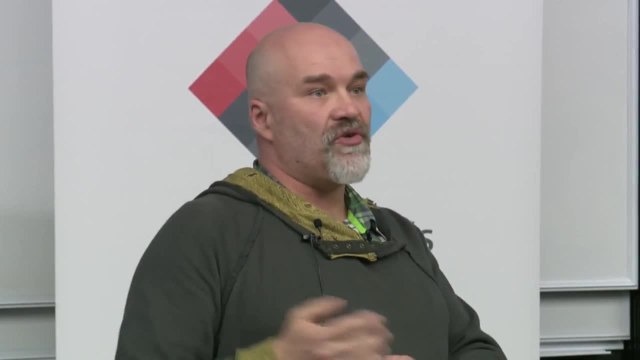 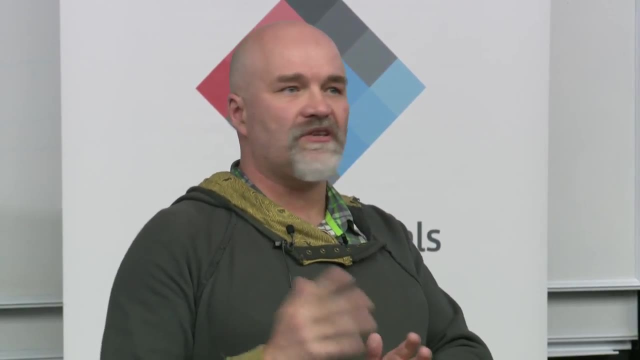 but it's only whenever we can connect. Once you have the new data, you can let the system train until the next start and go again and get better and better. So that's exactly the way we want to do it. There's no problem there. 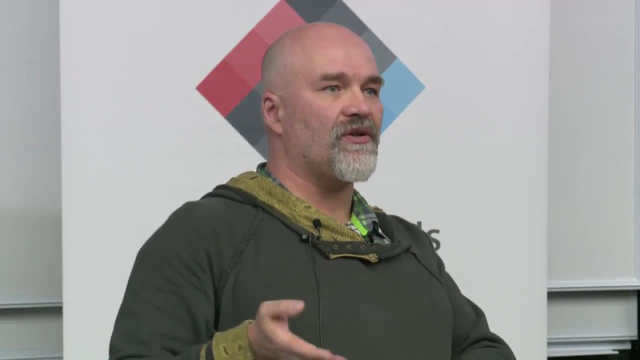 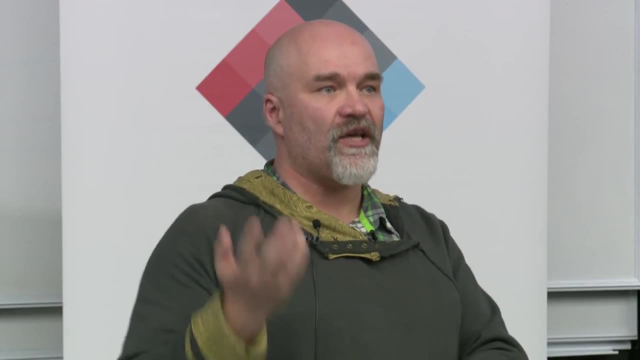 But at the moment you cannot say I'll be always connected, And it's true in New Zealand and other places. And the places where you want to place these agents is where humans cannot go, because it's difficult, it's time consuming. 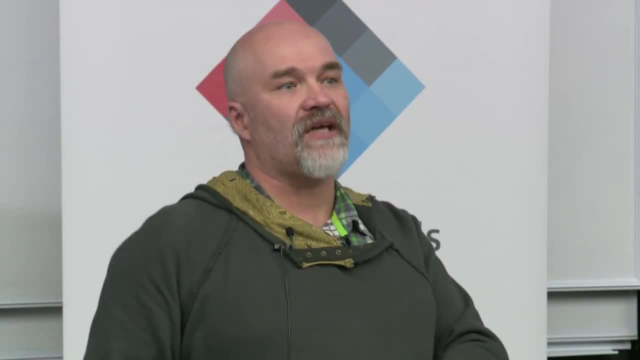 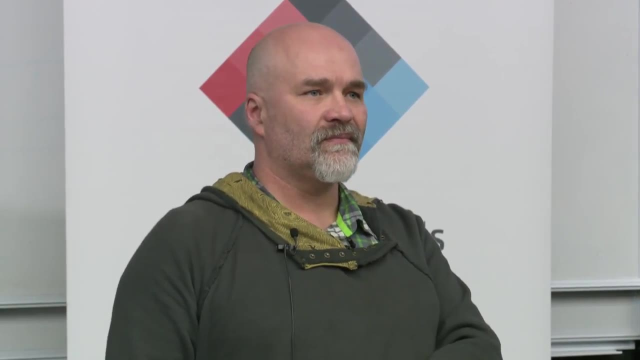 And in these places in Mexico where we were, there's limited capability as well. So it's often the difference. You know, in the city there's no problem, right? I have a supplementary question. It's completely different to this. 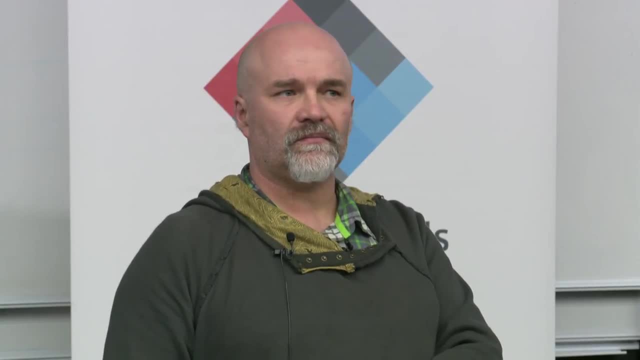 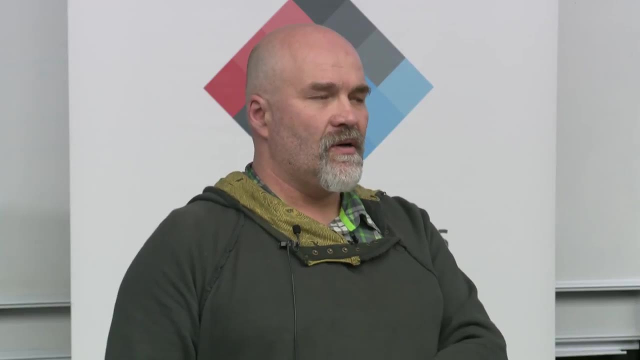 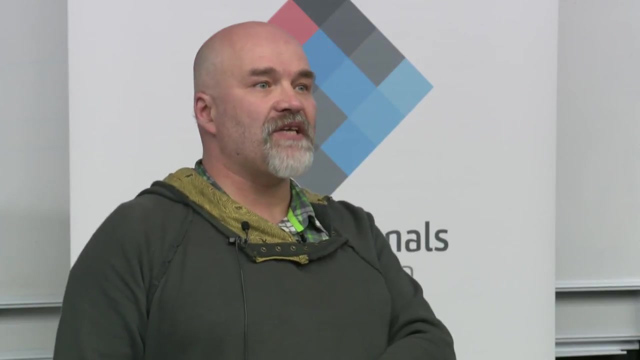 I know you mentioned you worked on VECA and neural network and all those utilities. Have you looked at TensorFlow? Have you got any opinion on that? You don't want to hear my opinion about that, But no, there's basically No, we haven't looked at TensorFlow yet.